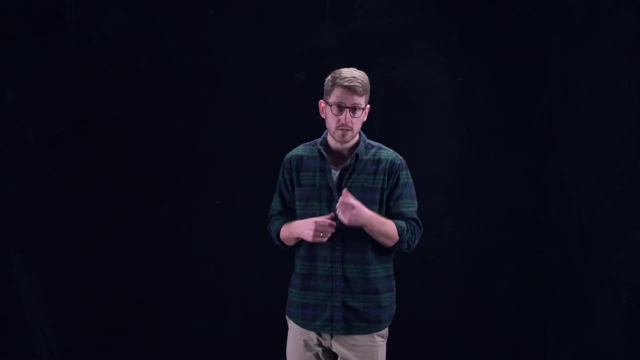 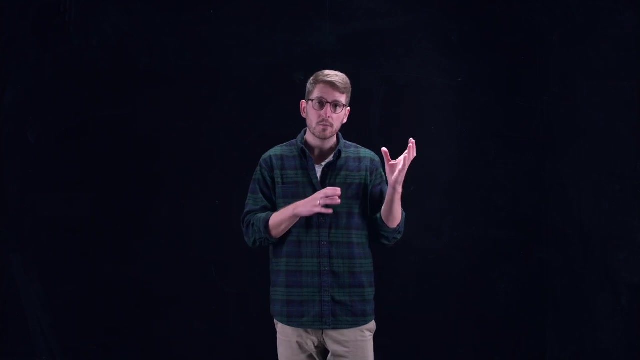 fundamental set of solutions. right, it's just finding roots of that characteristic polynomial. Now we've spent a long time burying our head in the theory, so what I want to do today is I want to do a little bit of application and, in particular, I want to focus on mechanical 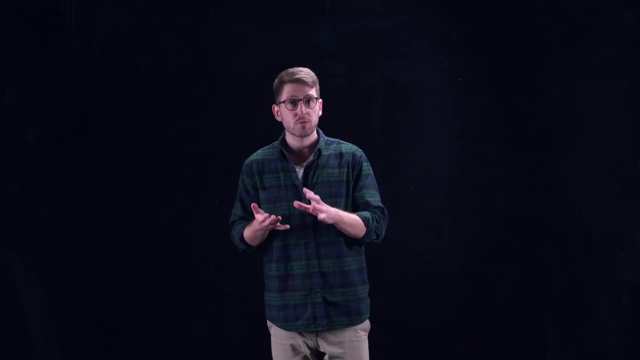 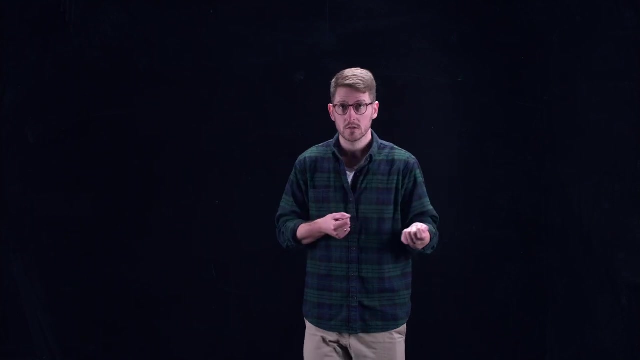 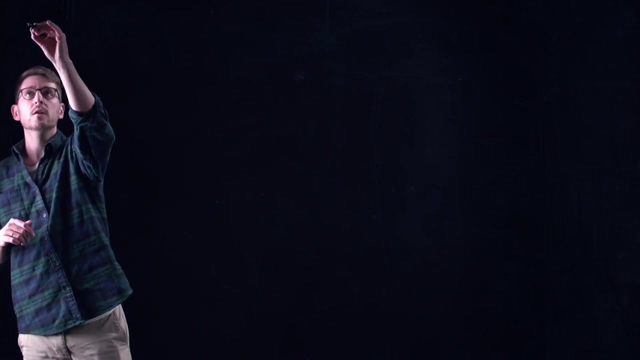 vibrations. So what I will do in this lecture is derive a second order linear constant coefficient differential equation that comes from a specific mechanical system, to show you where these things might come up and how we can interpret the solutions. Now let's go ahead and get started. The specific system that I want to look at is a very, very simple. 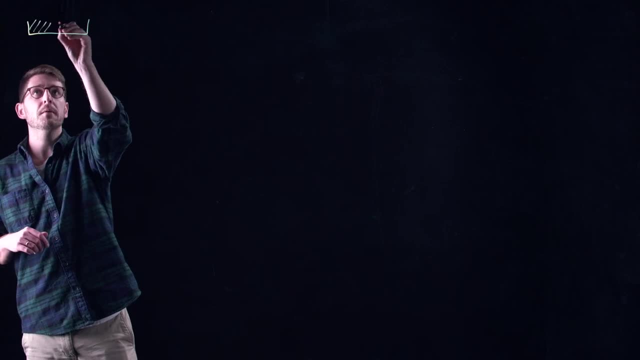 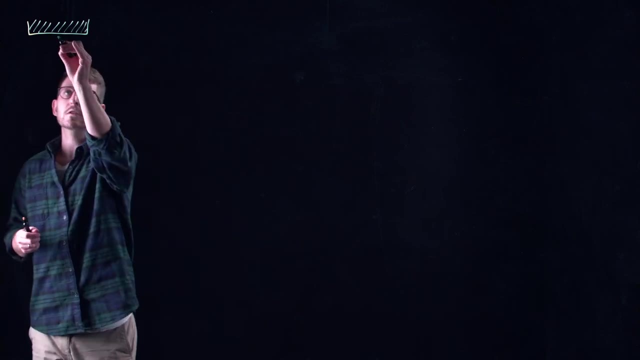 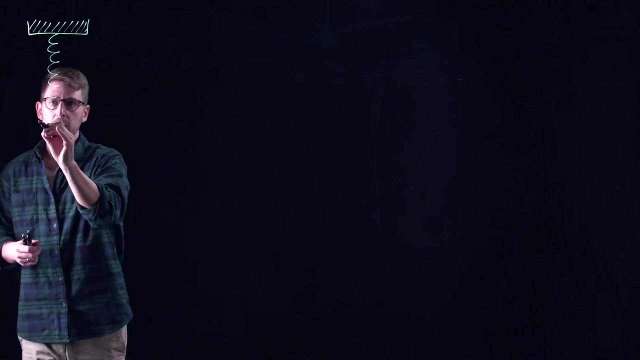 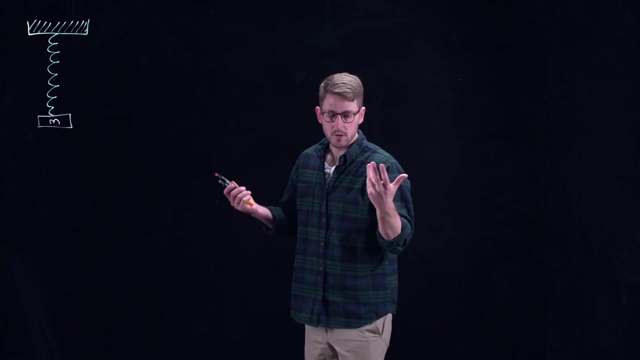 so-called spring mass system. So we imagine, maybe we have something that we can anchor to- this might be maybe the roof or something along those lines- and we have a spring that's being pulled down off of this thing, and what's pulling it down is some mass that sits underneath it. So this mass is going to be of- uh, this is going to be. 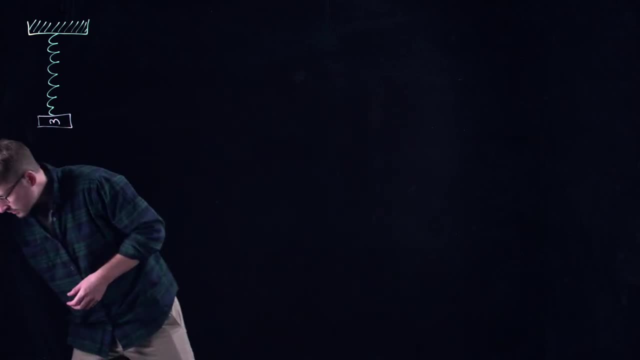 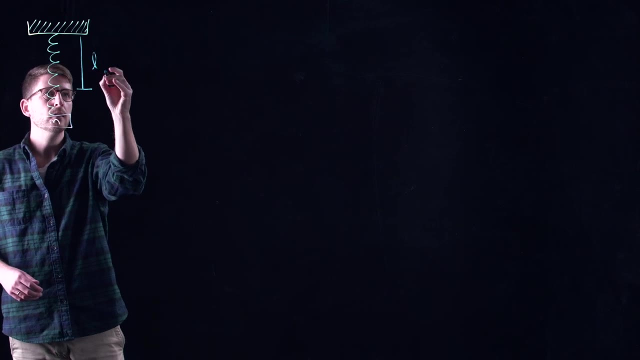 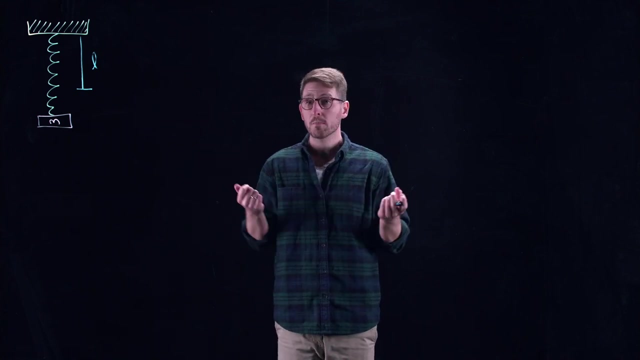 a little kind of physics, but it's going to be m kilograms, and there's a few things that we should denote on this right away. First of all, we will let little l equal to the unstretched length of the spring. Okay, So if you just take, say, out of your pencil and look at your spring, you 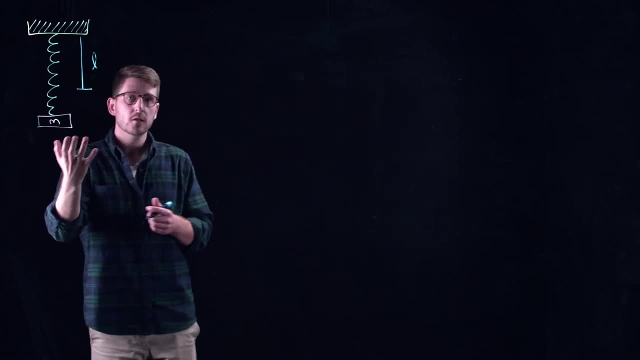 measure the length of that spring. that's going to be, uh, this little l. Now, of course, you can probably imagine what's happening here if I put a mass on this thing and I just lean forward and the spring is going to be m kg and that will not work. 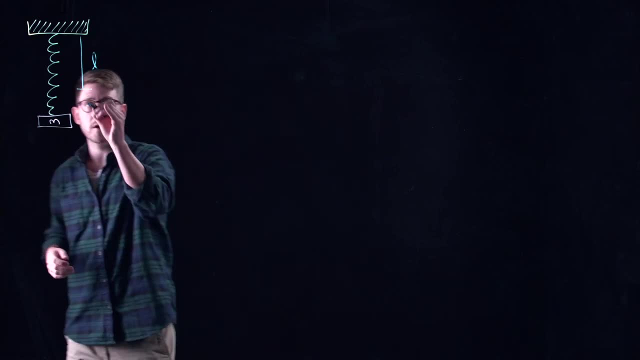 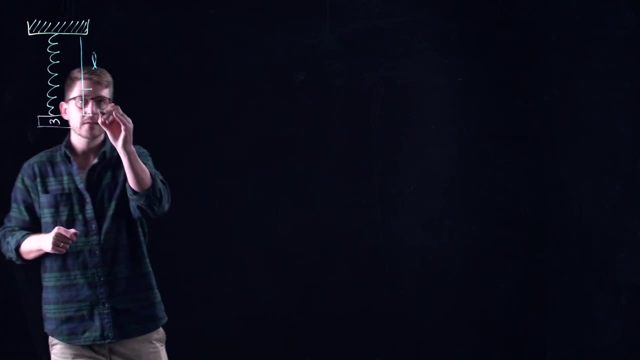 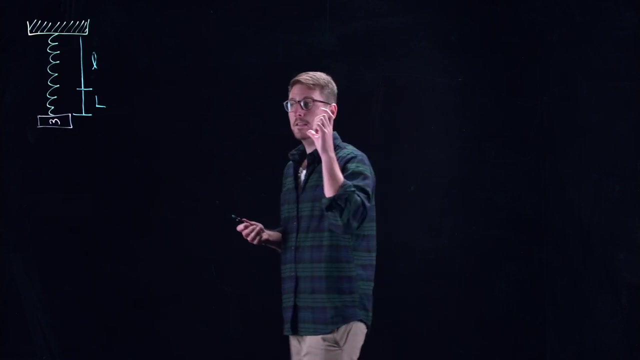 let it sort of hang there. It's going to stretch out the spring by some amount. Again, just take your spring from your pencil and pull it a little bit right. And so in this case, we're going to use capital L to be the amount or the distance that the spring is being stretched by this mass. 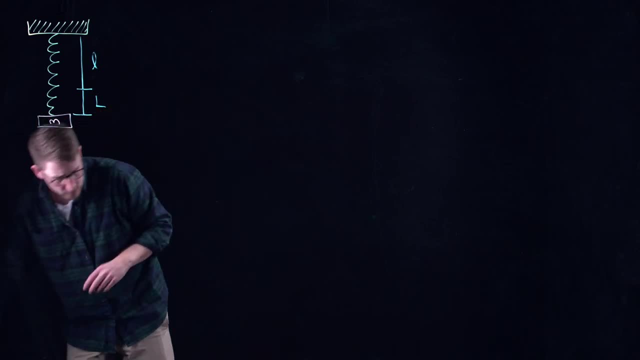 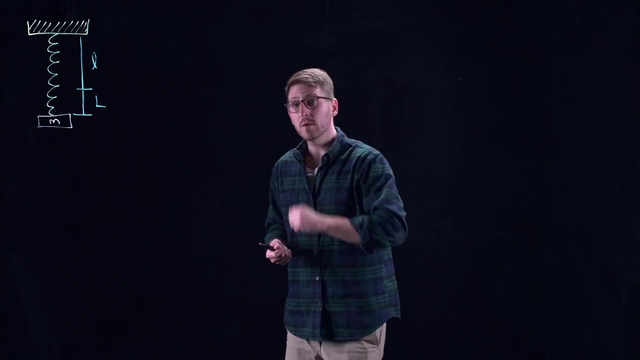 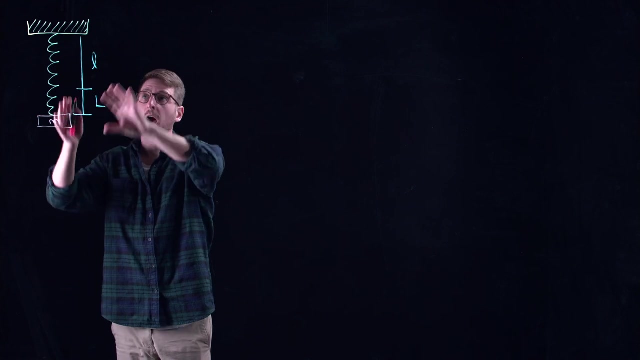 that's hanging down here. Okay, so the first thing that we do when we derive mathematical equations is we go back to first principles. That means going all the way back to the physical forces that are acting upon this thing. Now, for the time being, I'm going to think of just the spring. 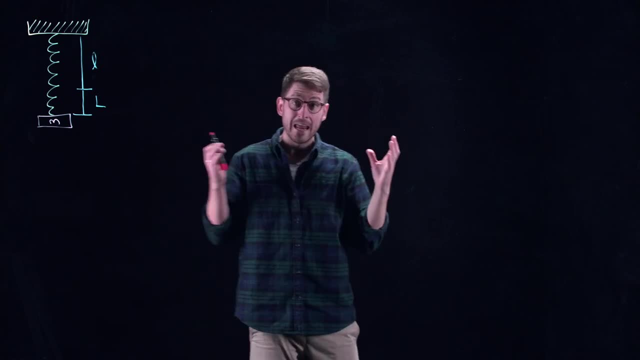 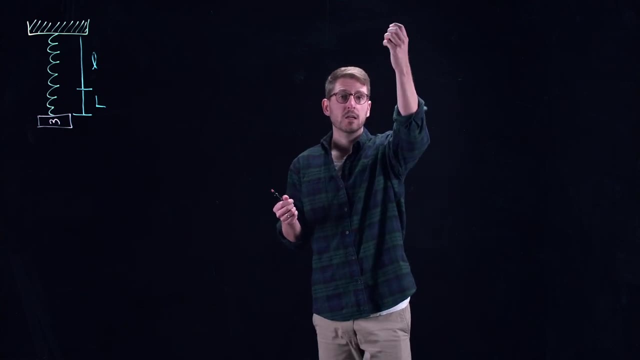 being stretched and pulled down by the mass. There is no dynamics here. This is a static system, That is, it doesn't change in time. So what I did is I hooked this thing up and I put this mass on there, I let it go, I let it pull the spring down, I walked out of the room for it. 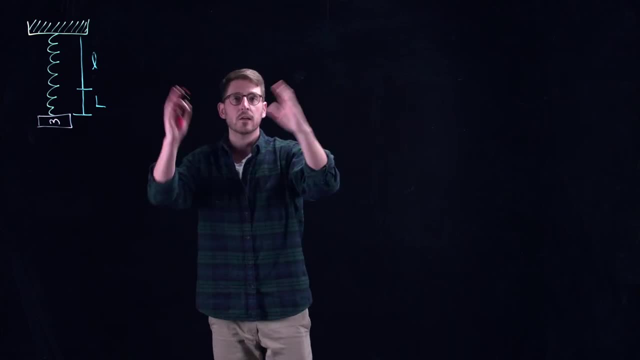 to do all that work. I let it go. I let it go. I let it do all that work. I let it do all that work. maybe an hour or something like everything settled down. it came back in and everybody is in a nice. 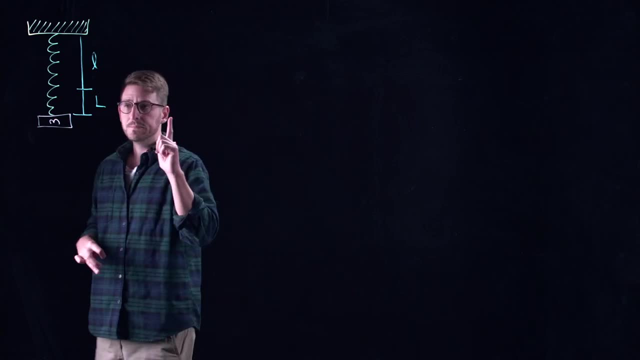 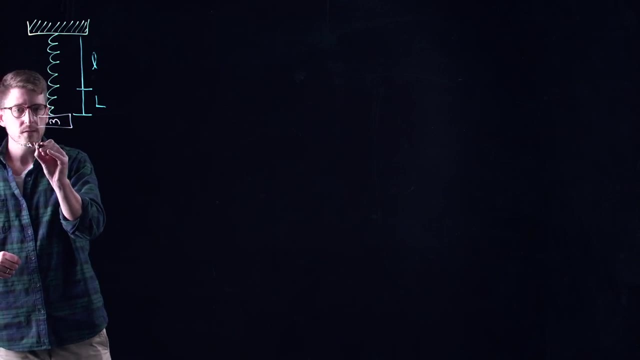 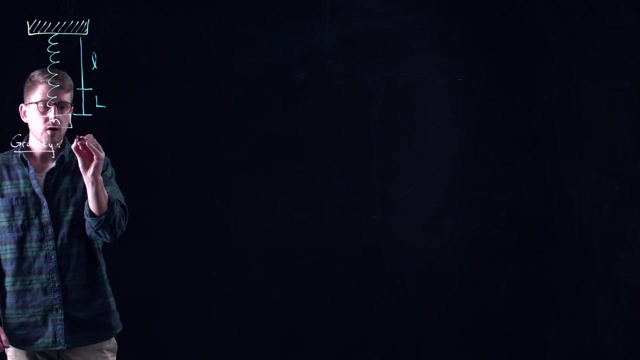 static state of equilibrium. well then, immediately, there is one force that we know is acting on this thing, and that is the force that's pulling the mass down, that is gravity. and in this case, we know from newton's second law that the force due to gravity is just equal to mass times. the gravitational 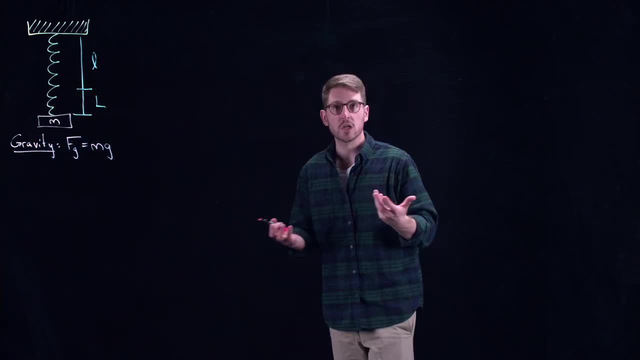 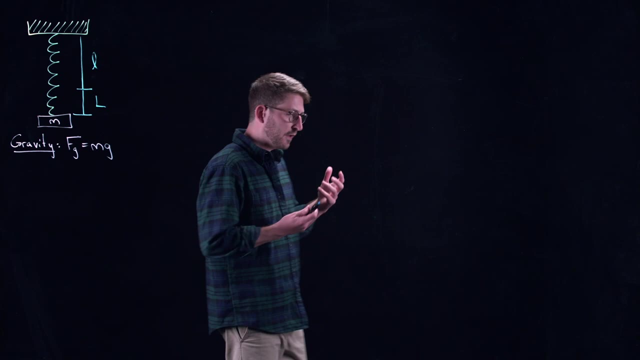 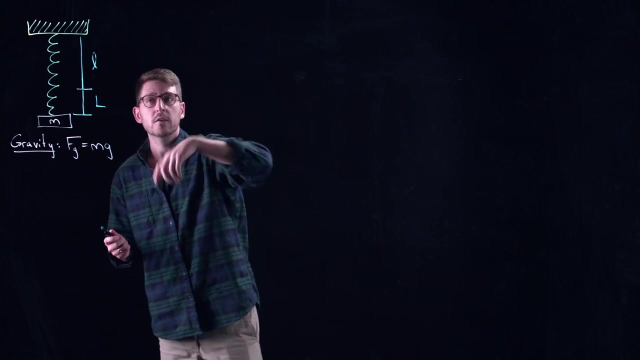 constant of acceleration. so this is g, this is 9.8 meters per second squared. now, if you think of how to do a free body diagram, we know that we need to have. in this case, if gravity is pulling us down, there has to be some equal and opposite force that is pulling us up. 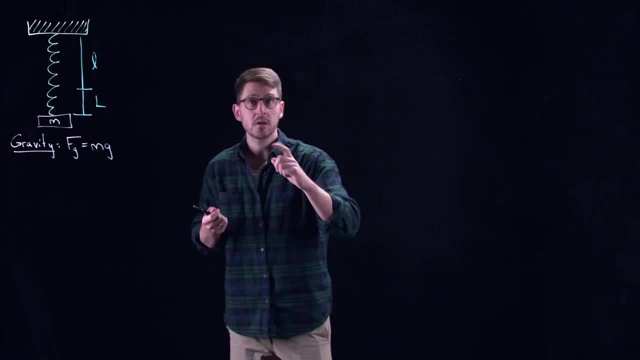 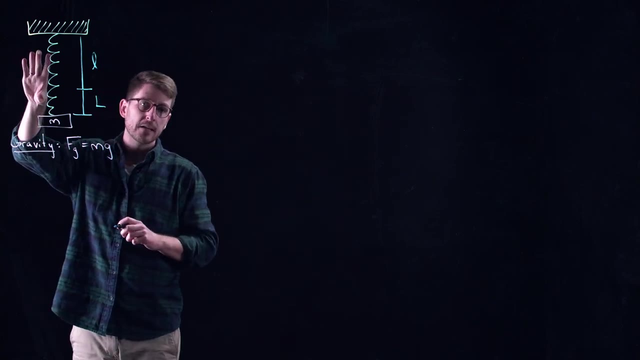 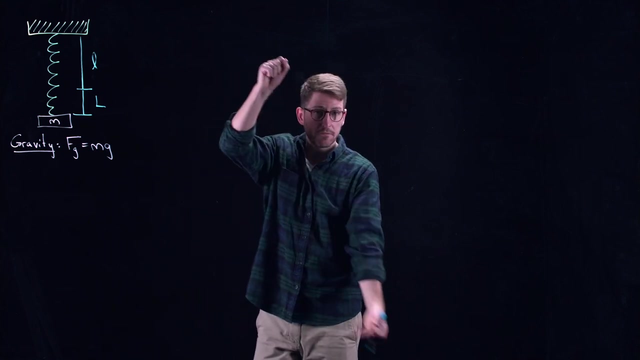 again, this thing is in this state of equilibrium, it is standing there, so there's got to be something pulling us up as well. and you You might remember from a physics class that that is actually going to be the spring tension, right? So the spring wants to be put together, right? It just can't fall forever, right It's. 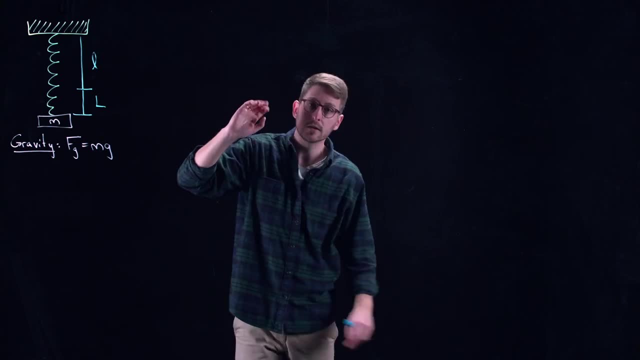 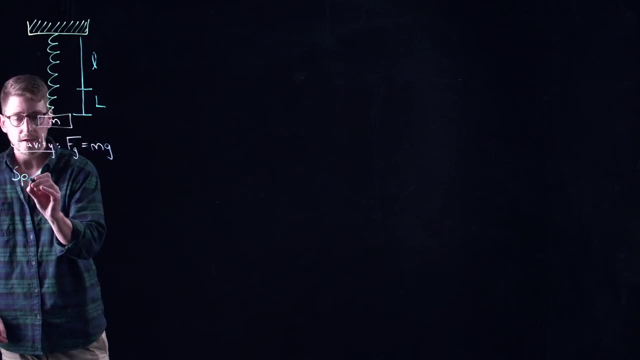 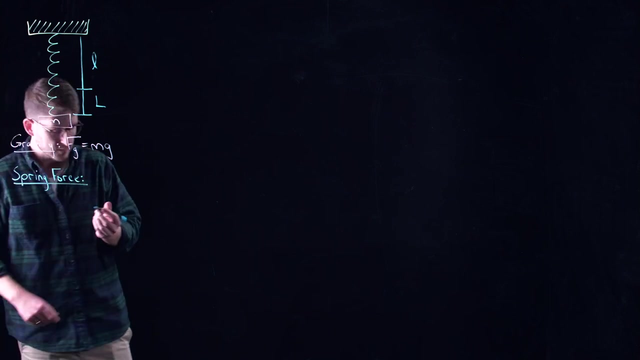 not like a piece of rope, where if I put a mass on it it would just fall until it hit the floor. The spring is pulling this thing back up, So we actually also have a spring force, and the spring force in this case is given by what's called Hooke's law. So I'm going to call 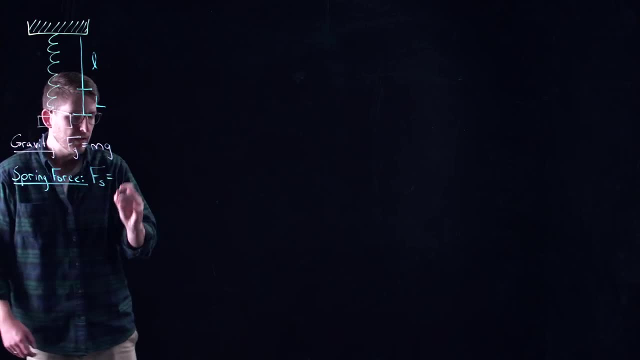 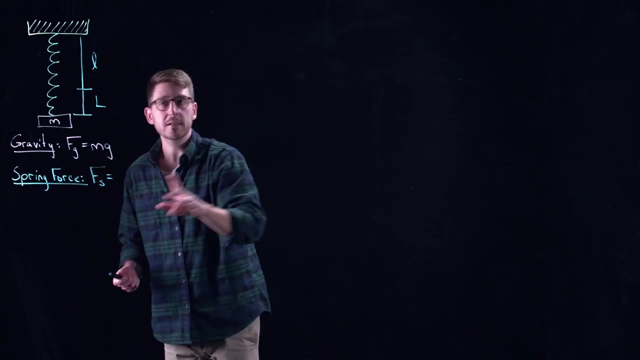 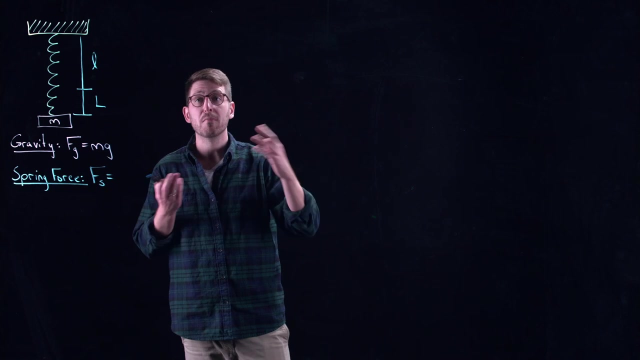 this F sub S. Now I'm talking about gravity going downwards and I'm using that to be the positive direction. That means the spring force is acting upwards. I'm going to use that to be the negative direction, the opposite direction of gravity. That's all minus means here. okay, 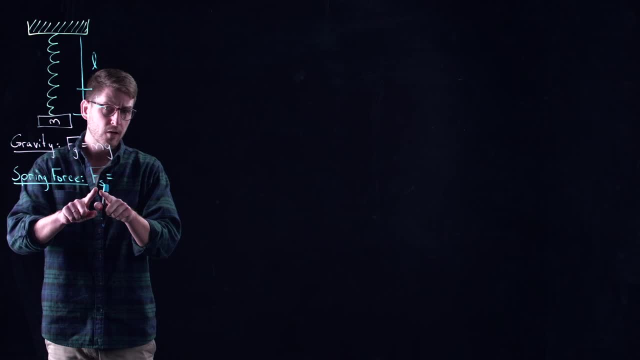 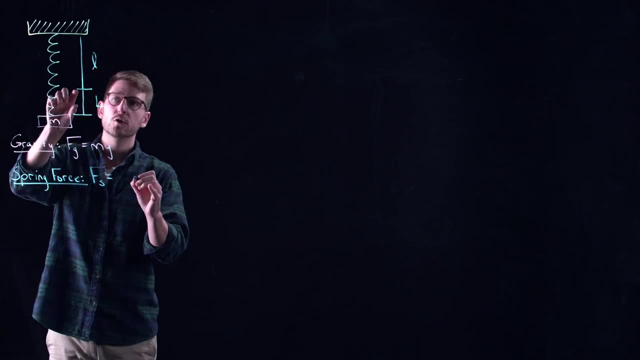 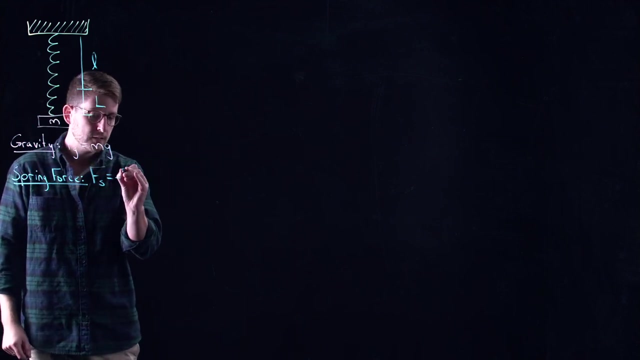 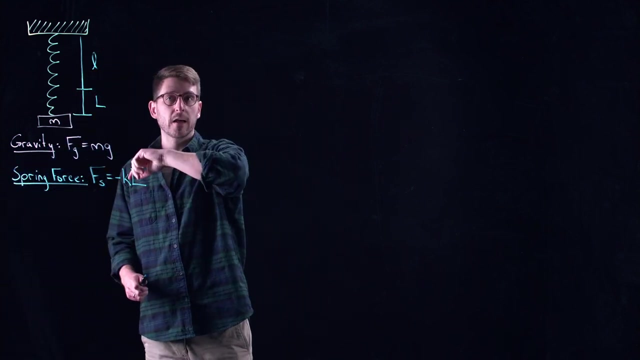 And in this case we can use Hooke's law, which says that the force of this spring pulling us back up is proportional to the length that this thing has been stretched from its original length. So that is minus K times L. L is the amount that it's been stretched beyond its natural length. 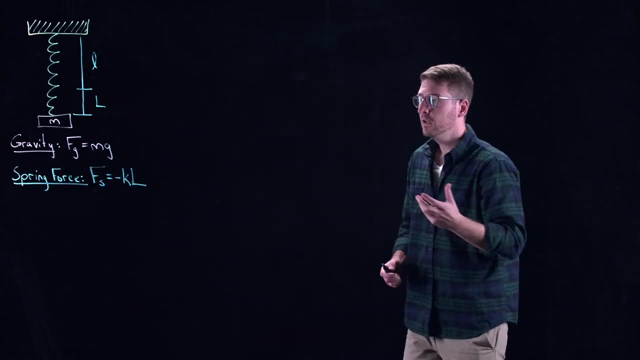 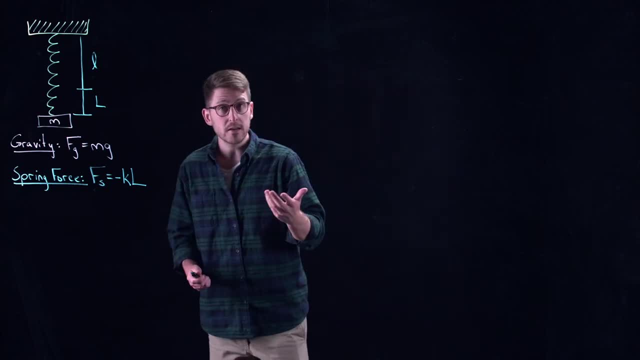 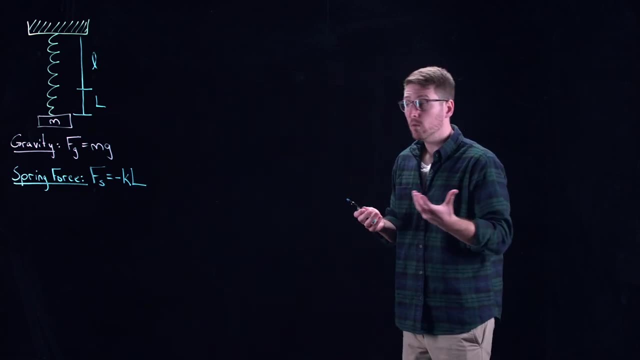 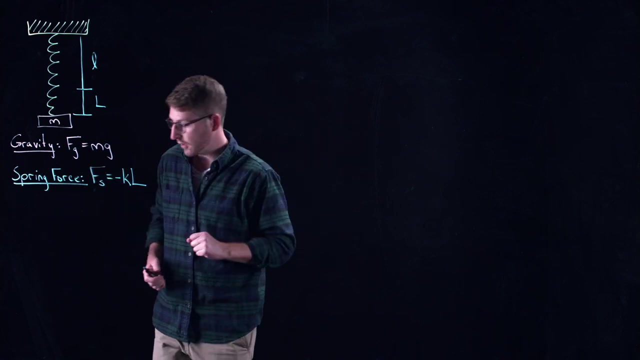 So K is the spring constant. This is something that can be estimated from data. So if you were to sort of measure out this spring, we can actually find what this value is in the lab. But for our purposes we are just going to call this thing K. It's a positive number, That's all. 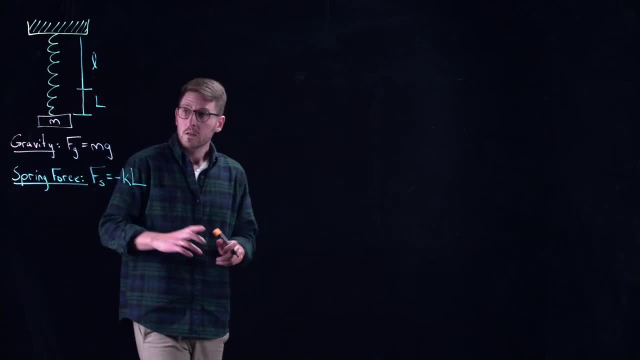 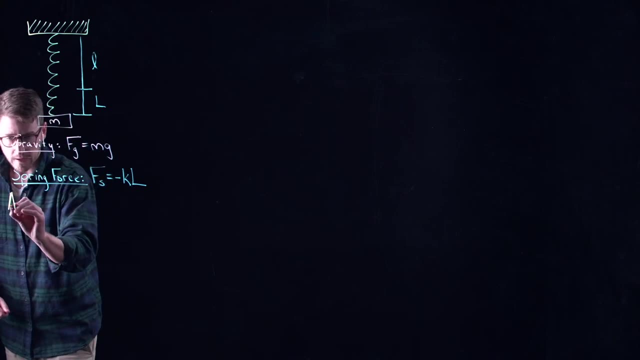 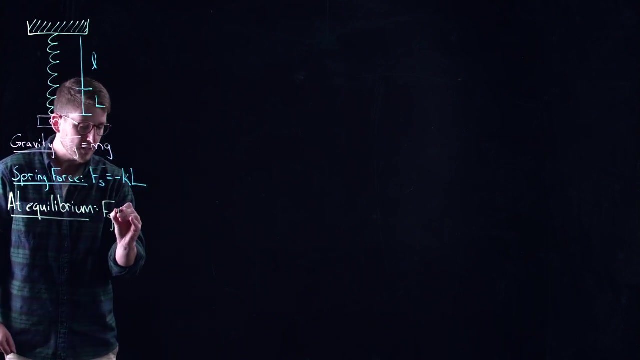 that we care about for the time being. Now, at equilibrium, this thing is a perfect state of balance. So that means that, at equilibrium, so at equilibrium, well, these two forces are equal to each other, They're balancing each other out. So it says that FG plus FS is equal to zero, which tells me that MG and then minus KL. 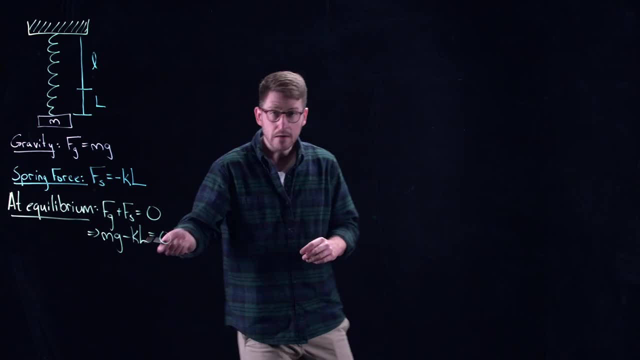 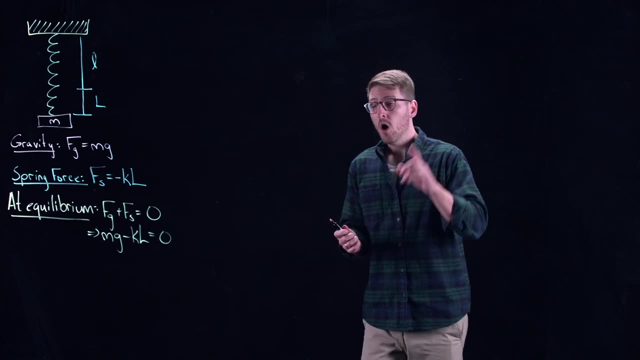 is equal to zero. Now, what you can get from this equation: you can rearrange to isolate from L, which will tell you exactly how far the spring has been stretched. Or, as I said, if you build this in the lab, you can just pull out your ruler and measure what. 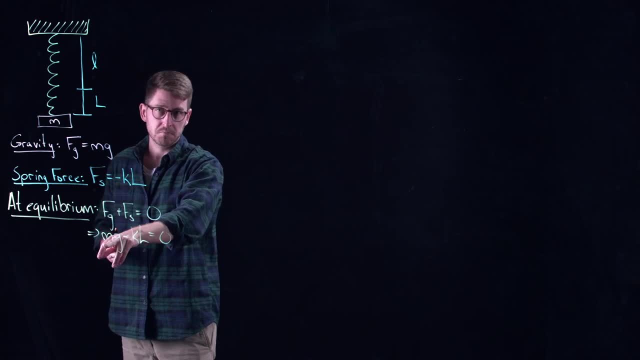 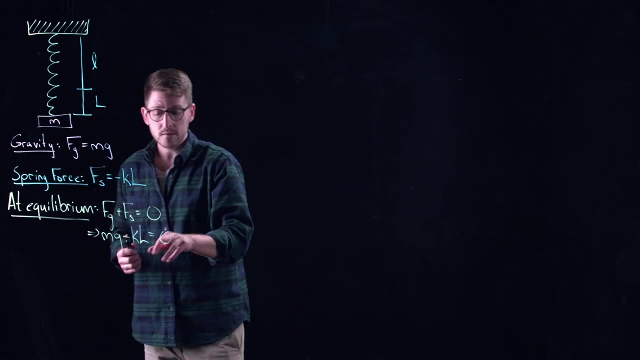 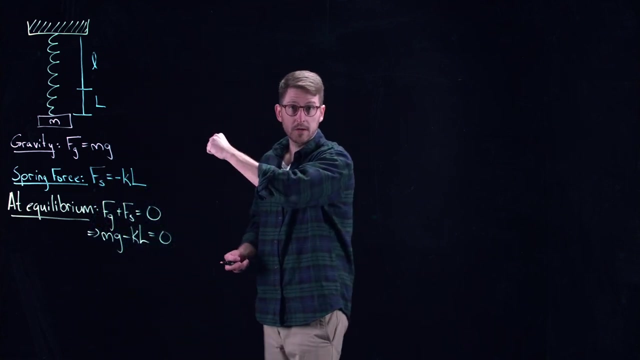 capital L is. We know what the mass is. Again, put this thing on a scale. We know the gravitational constant of acceleration And this equation, right here, provides us with a method of finding K from a physical experiment, right? So, even though K may feel a little bit inaccessible here, 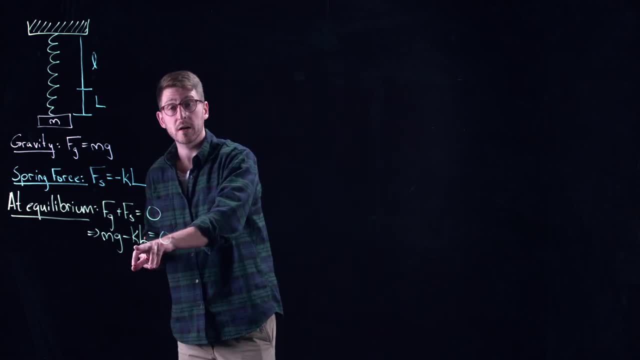 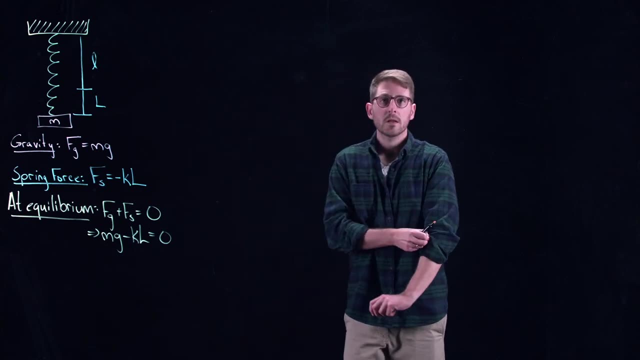 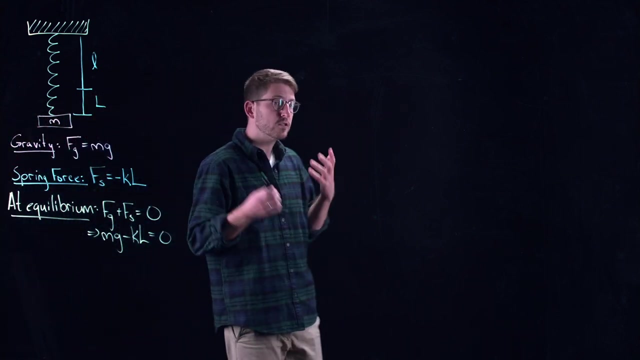 we just said, it's a positive number. I can actually go into the lab and I can find what this value is just from this equilibrium equation that I have right here. Okay, this is at equilibrium. There's no dynamics involved. That means that there's no differential equation associated to this thing. 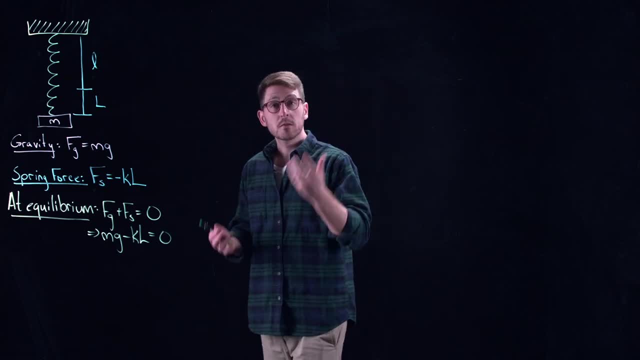 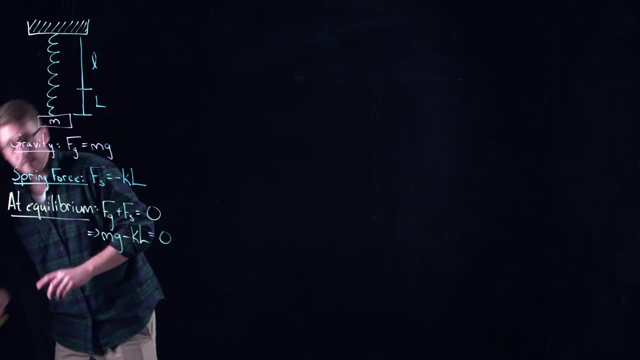 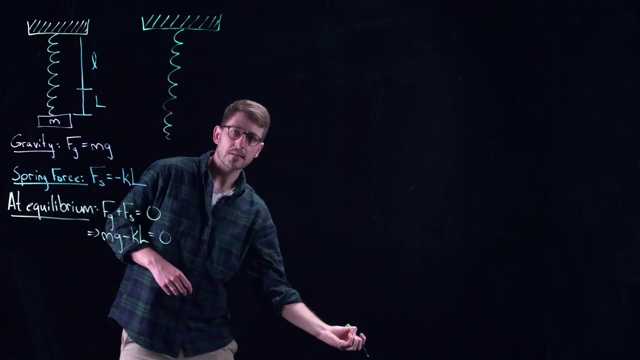 The question is: how do I incorporate a differential equation in this? Well, let's look at another scenario. So let's look at the K-1 equation. In this case, when I'm not at equilibrium, Maybe I let this thing settle down and then I walked back into the room and I pulled the mass down a little bit. 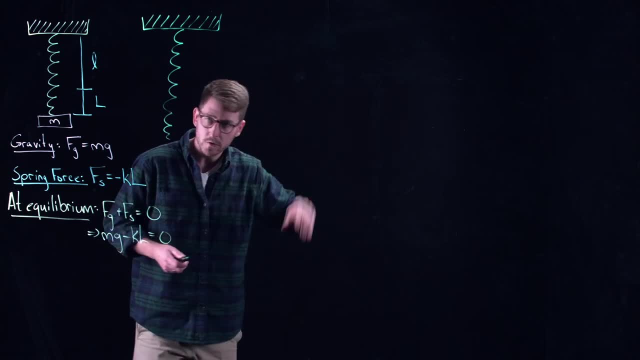 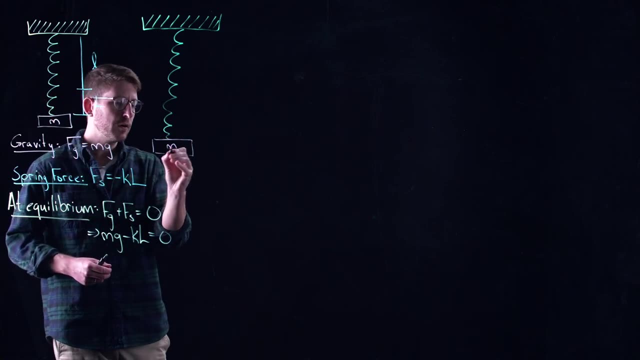 And then you can imagine what's going to happen. right, It's going to sort of wiggle back and forth, up and down. So the question is: how do we describe that mathematically? Well, what we're going to do is we're going to introduce another quantity here. 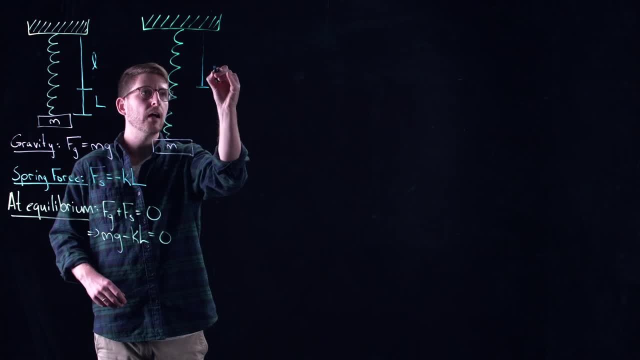 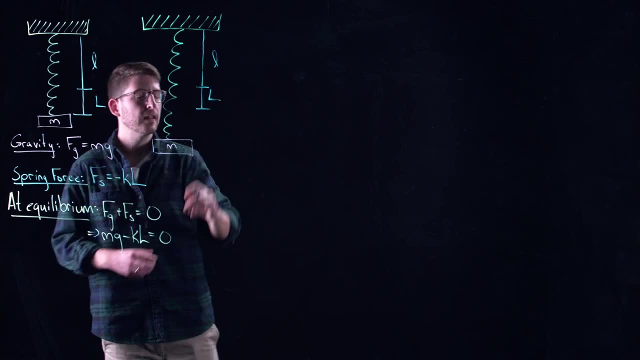 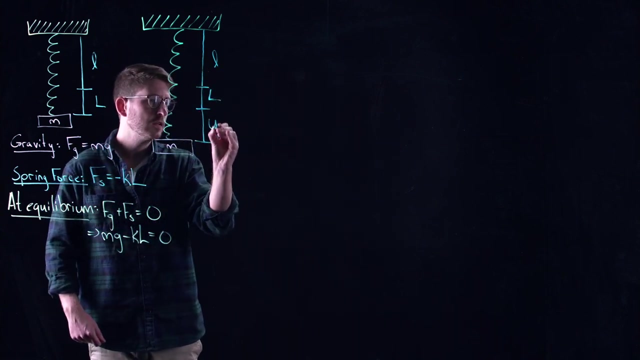 So first of all, we have the same two from before. We have little l, the natural length of the spring. Then we have capital L, the length that is going to be the displacement to equilibrium, And then what we will do is we will let u of t. 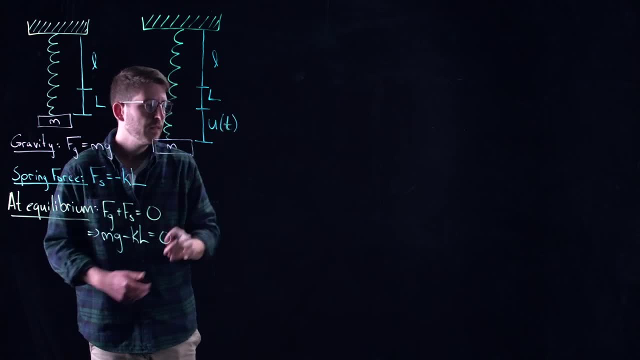 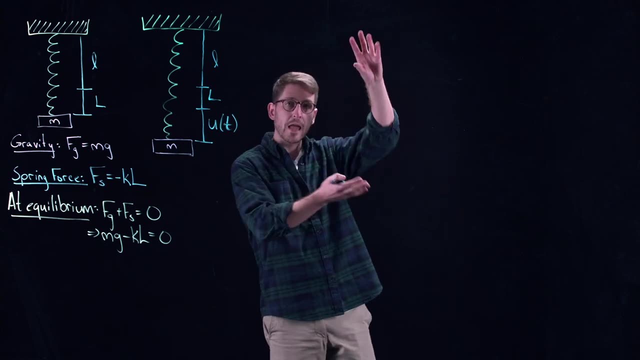 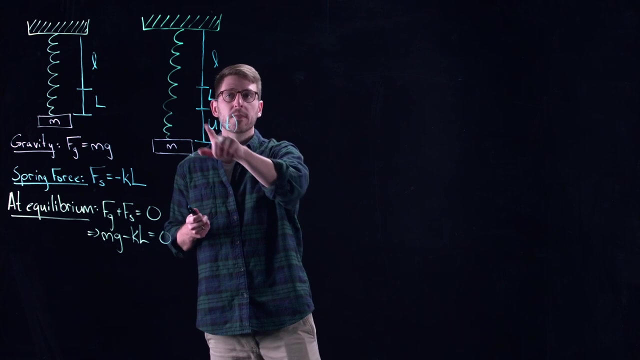 So it's going to depend on time. This is the displacement from equilibrium. So again, remember, this thing might be hanging from the ceiling And I came in and I pulled it down a little bit And let it shoot back up. u of t is describing this displacement from the equilibrium due to me pulling it at time. t. 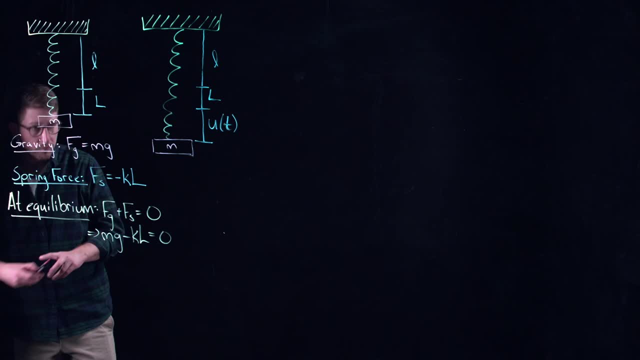 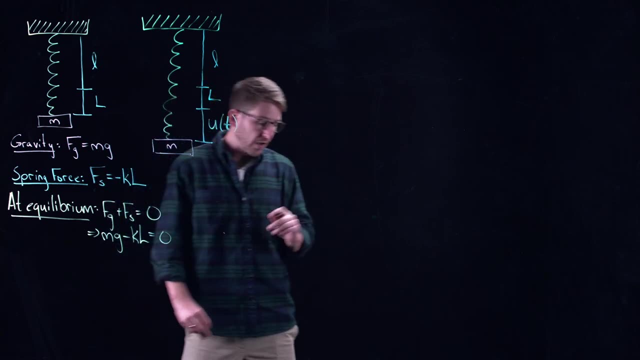 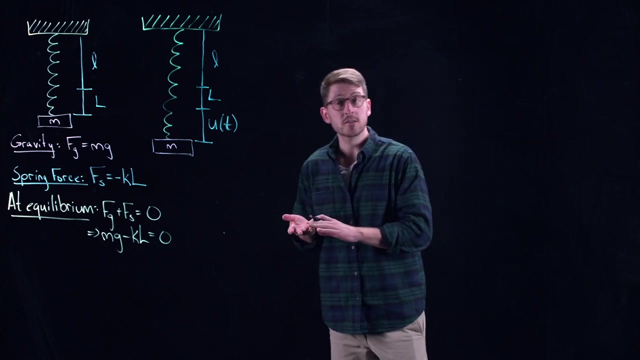 Well, here's what we know. We know that the forces on this thing are going to come from Newton's second law, So I've emphasized this before through this lecture series. But most differential equations that we encounter, particularly from physics and engineering problems. 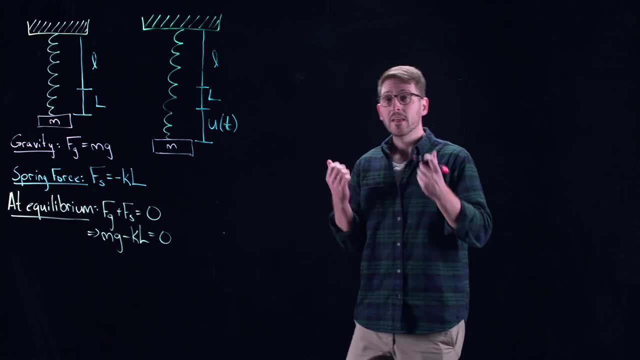 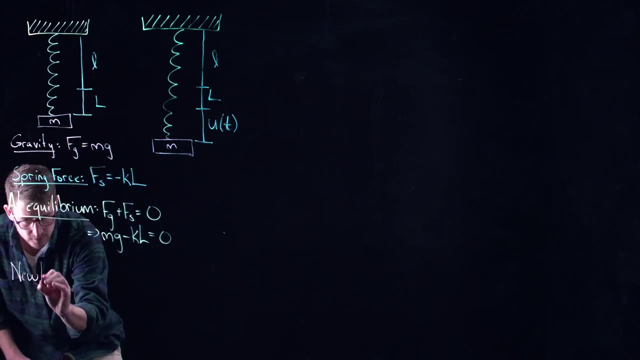 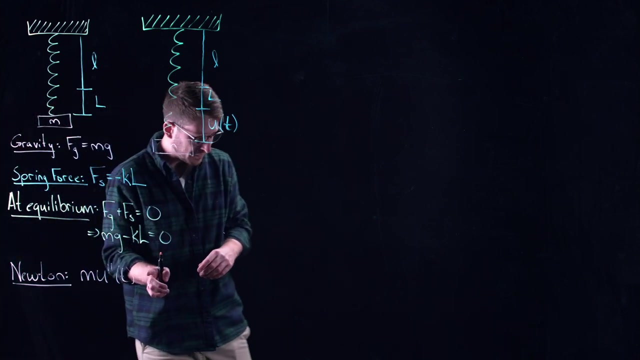 are going to be second order, That is, they depend on the acceleration, And that comes from Newton's second law. So here's what Newton tells me. Newton says that the mass times, the acceleration of my displacement, is equal to the sum of forces that are acting on this thing. 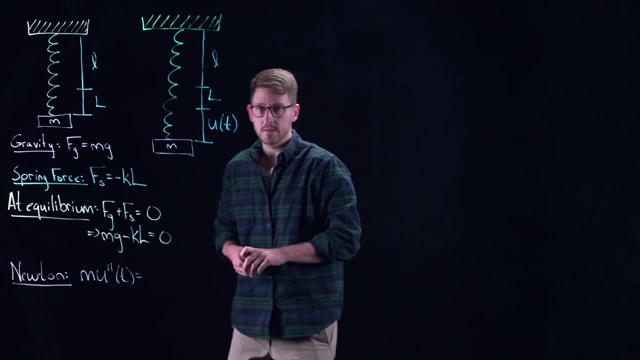 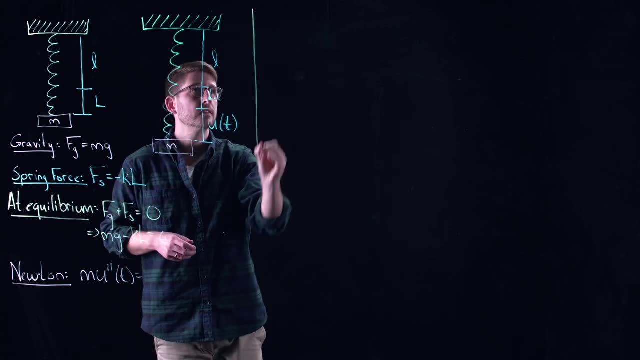 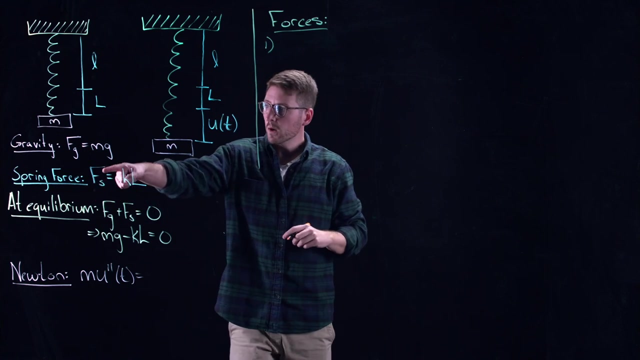 So, before I write down what this sum of forces is, let's talk about some forces that could be acting on this. So let's start here. So forces: Well, again the first one we've already seen here, and it could be the gravity. 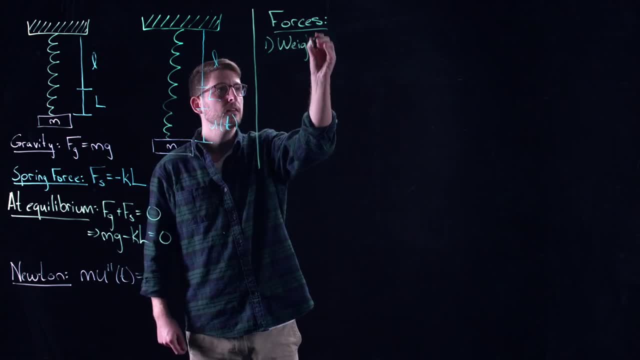 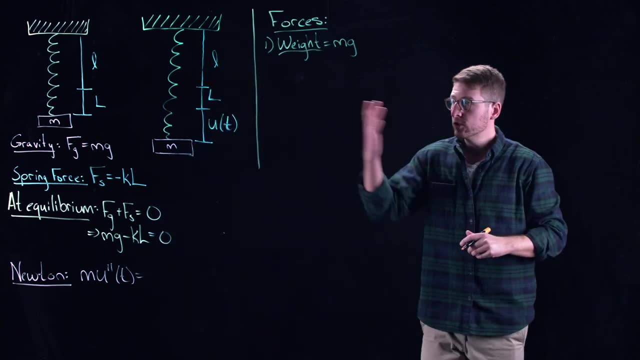 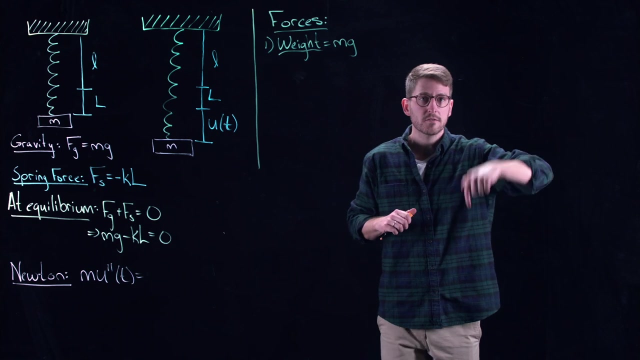 So in this case, this would be the weight, which is equal to mass times gravity. Okay, so that's still there. It's just acting on the mass, The mass, in exactly the same way. So, pulling down, we're using gravity to denote, or we're using the positive direction to denote downwards. 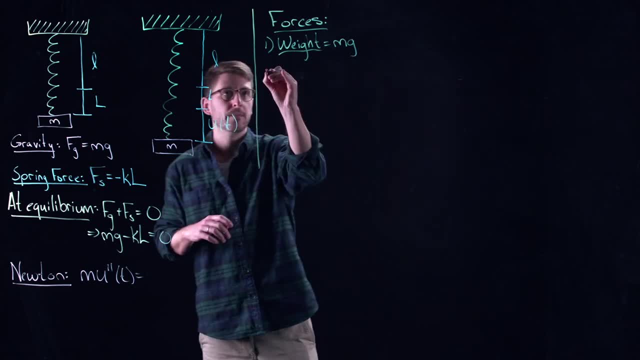 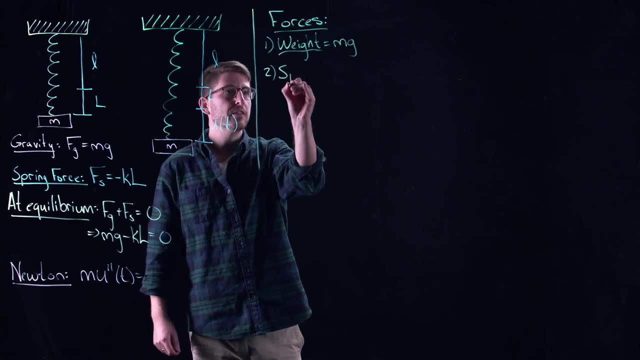 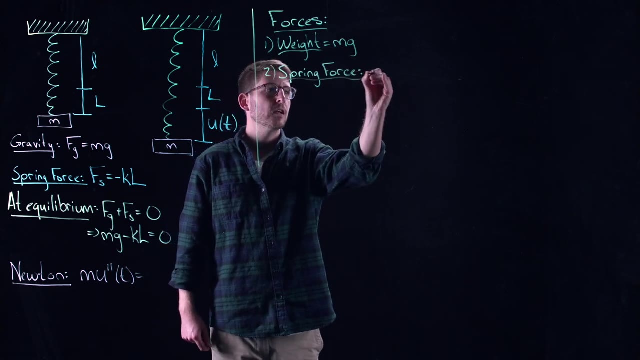 That means going in the same direction as gravity. Similarly, we still have a spring tension that we need to account for. So we have the same thing here. We have a spring force, But now it's a little bit different. It's still proportional. 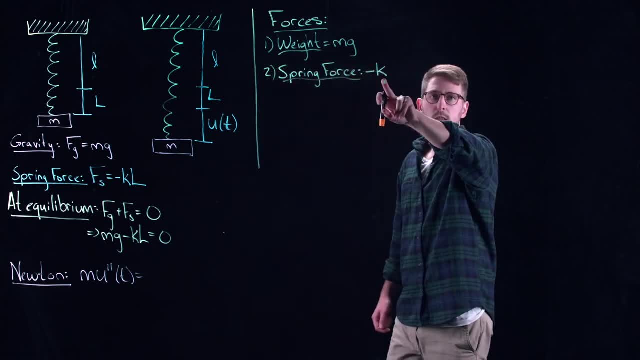 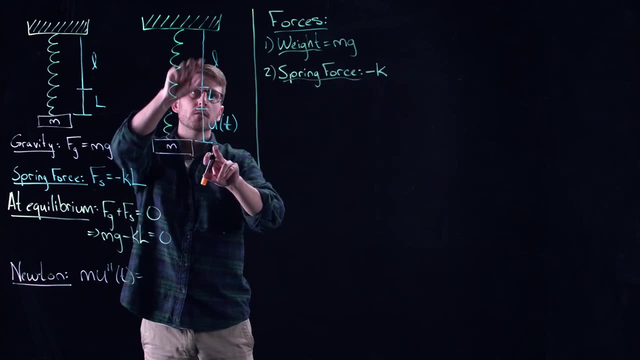 So going in the opposite direction of gravity. It is proportional. That's what the k is in here. But now the length that this thing is being stretched from its original little l is l plus u, So there's a little more. 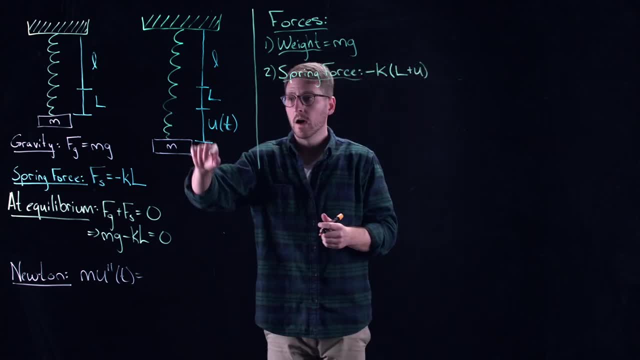 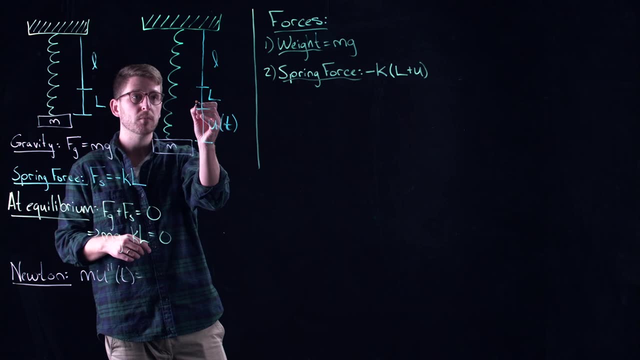 Right. l could be positive or negative, depending on you. know I've drawn this in such a way that u is positive, But you could imagine this thing bouncing up and going above equilibrium as well, which would give you a negative value of u. 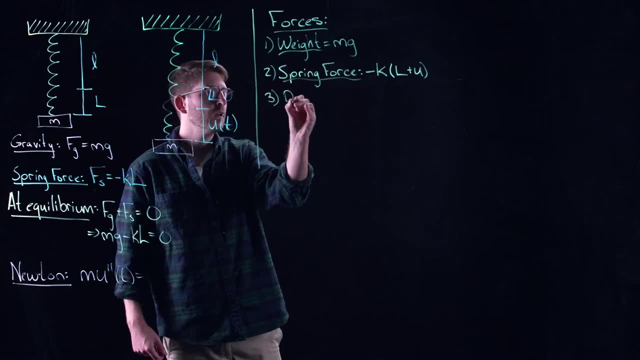 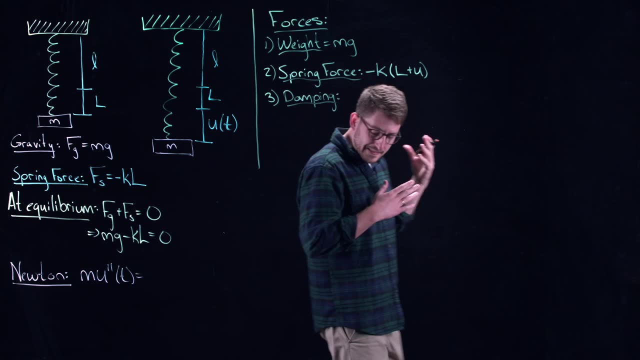 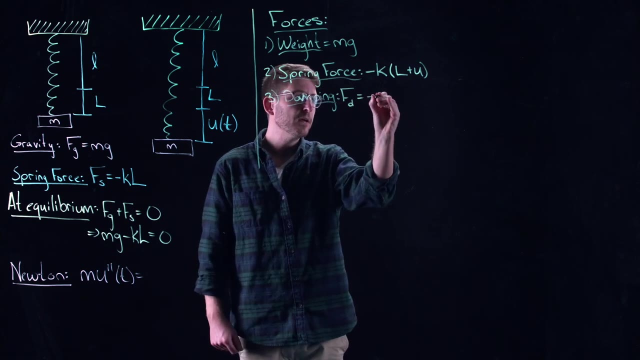 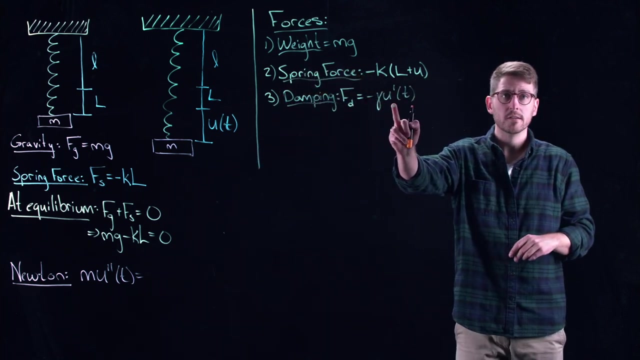 Okay, let's keep going. We could have another force that's acting on this thing, And it could be damping. So in this case, say Fd, And damping affects or is proportional to the velocity of your displacement. So here gamma is again going to be a positive. 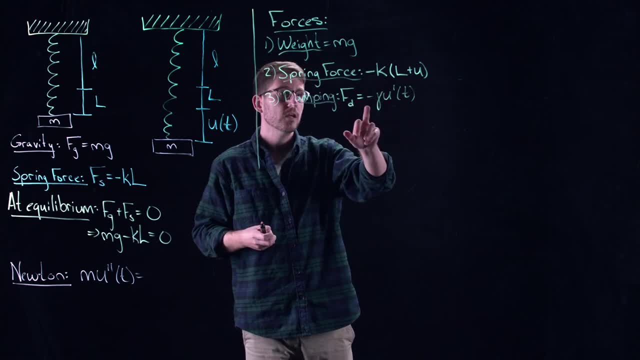 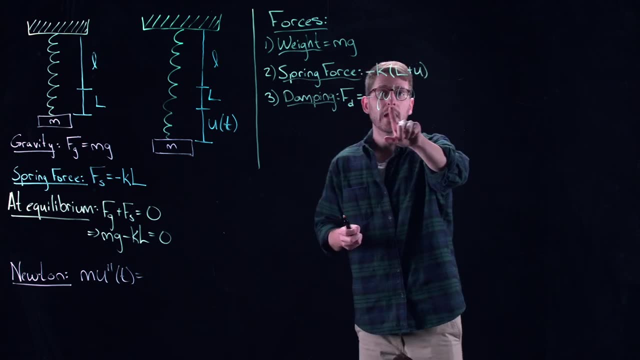 A positive quantity. Just like my spring force, This is going to be pulling me in the upward direction again, So it's sort of pulling against me And it's pulling against me. So the faster I go, the more of a pulling that I get from this thing. 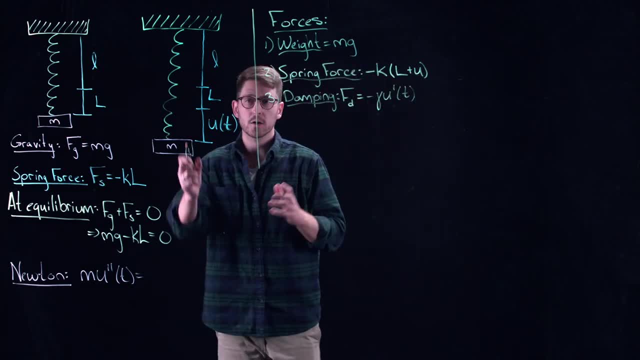 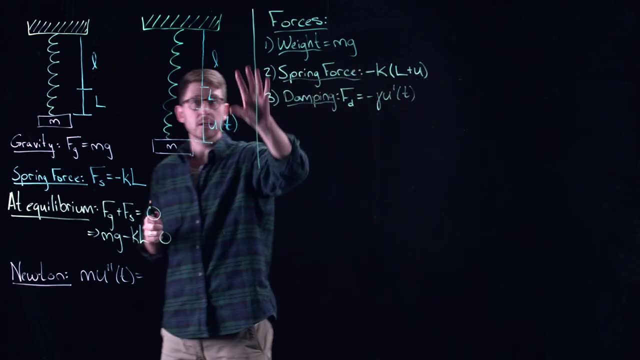 So there's all kinds of different ways that damping could be observed in this system. It could be something like air resistance, Or maybe you're doing this in some other medium than just air, So, for example, you could imagine you're doing this underwater. 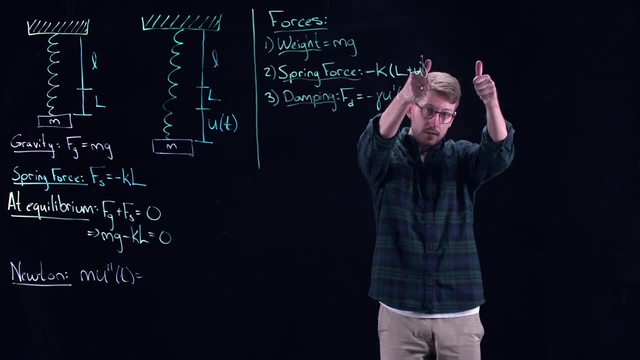 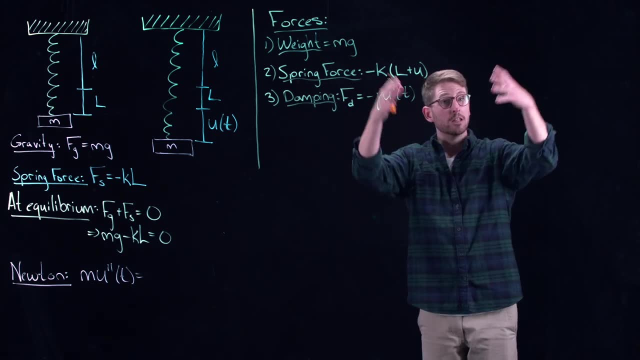 Well, the faster that thing's going, the more of a push the water resistance is giving you. That's exactly what you're seeing right here. Or, if you really wanted to make this crazy, you could imagine doing this in a big tub of honey. 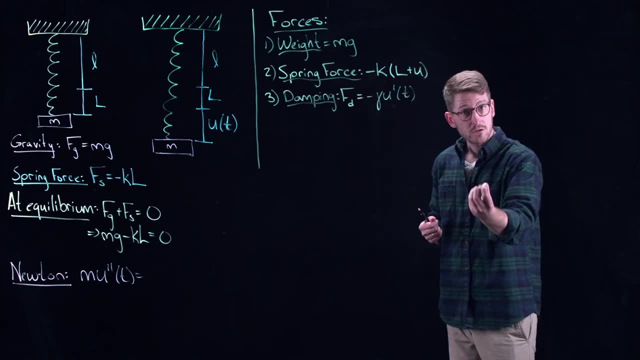 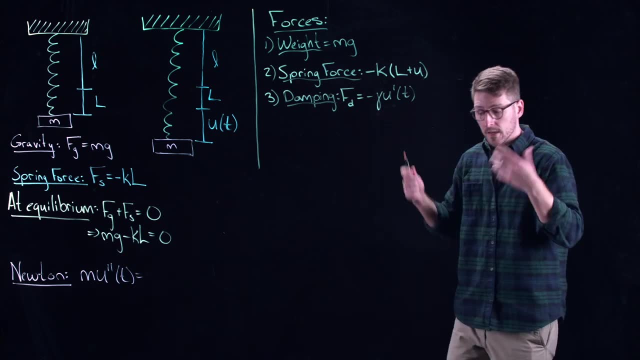 So it's extremely, extremely viscous. The faster you try to move here, the more the honey is pushing against you, So that gamma would be huge if you were in, say, a big tub of honey. Now, another way that this could sort of present itself is if you were to draw, maybe. 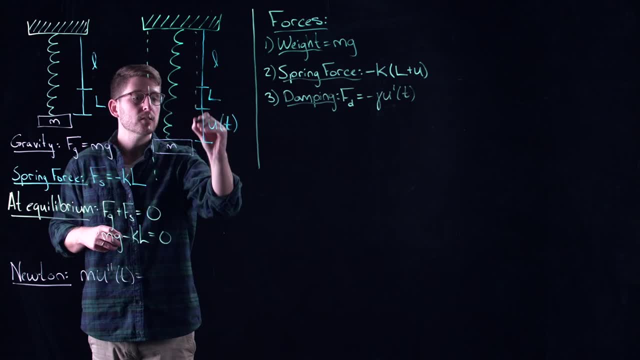 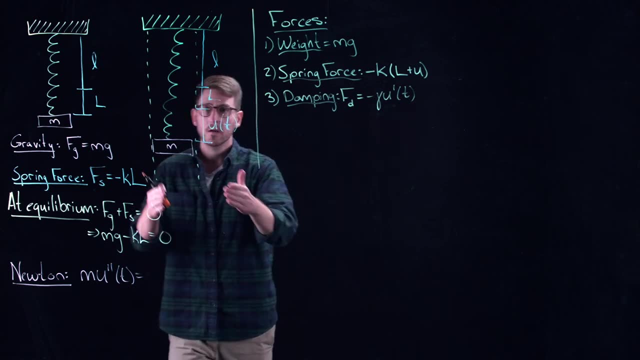 or if your experiment had some little guide rails to make sure that your mass was only going in the vertical direction. There was no left and right displacement here. Well then, this could account for the friction against these guard rails that you've set up here. 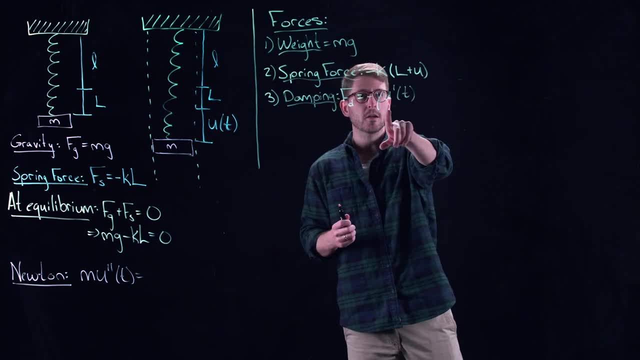 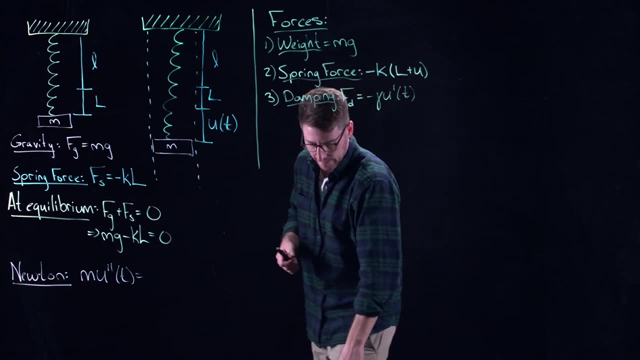 So that's another way that damping can come in here. The faster you're going, the more velocity you have, the more the friction is going to erupt. So it's going to come up here and it's going to act against you. So there's a lot of different ways that this can come up. 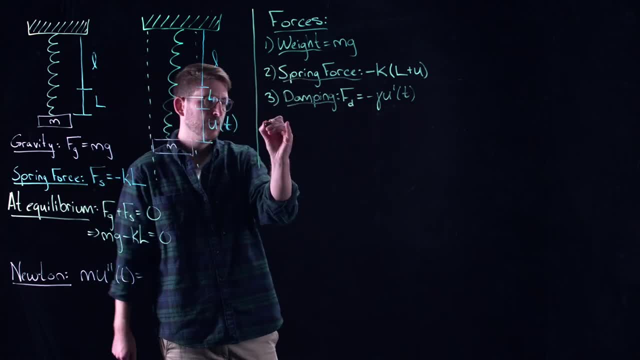 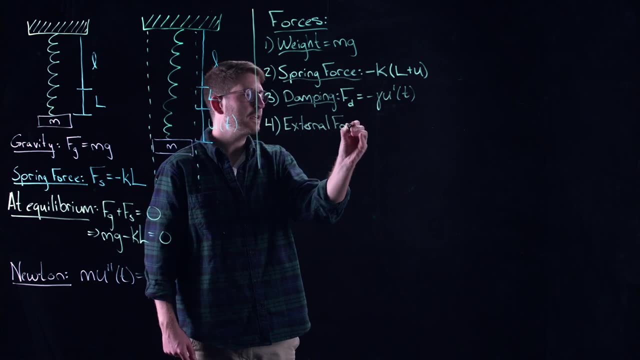 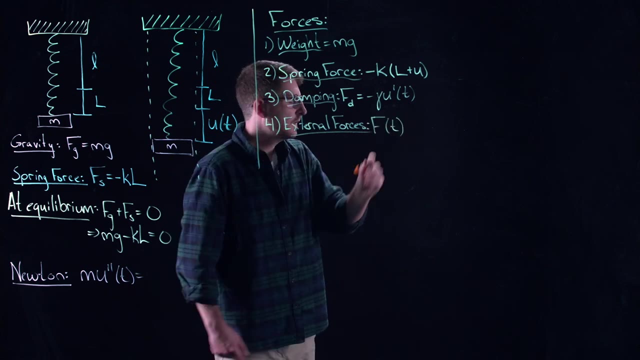 I'm just going to encode it by this piece right here. And then the last one is external forces. So we'll look at this later on in the lecture more, But I'm just going to call this capital F of T. So one example of this is maybe the ceiling that I bolted this to. 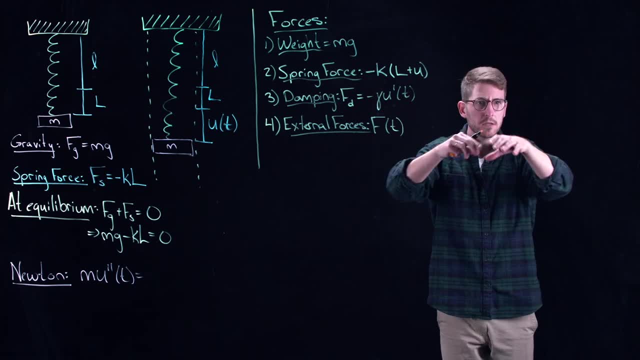 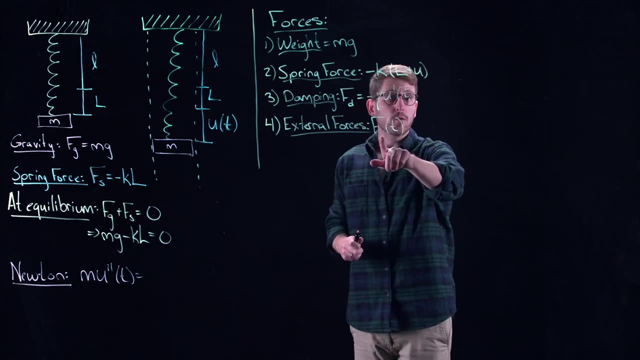 Maybe I have some control over this. Maybe it's not a ceiling, maybe it's just a long bar And I can shake that thing up and down. Well, that would be an external force. That's me acting on this thing in a prescribed manner. 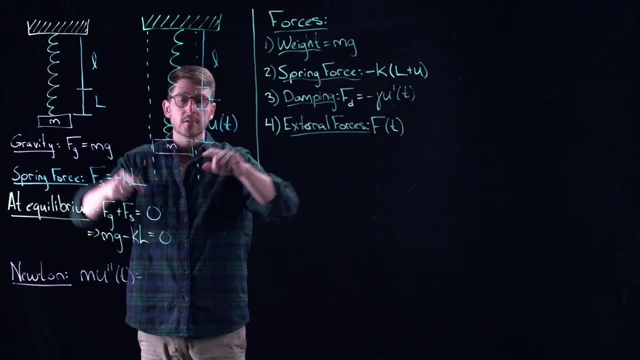 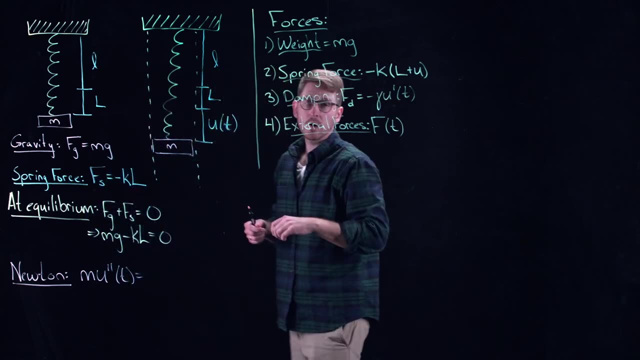 And of course you can imagine if I'm shaking this thing up and down, for example. that's clearly going to travel through the spring and cause a weird action on the mass as well. So those are the four forces that we are going to consider acting on. 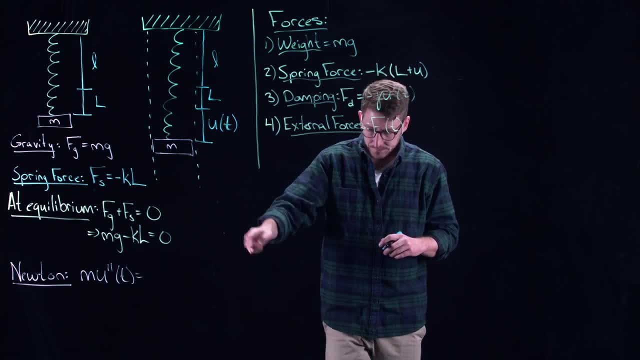 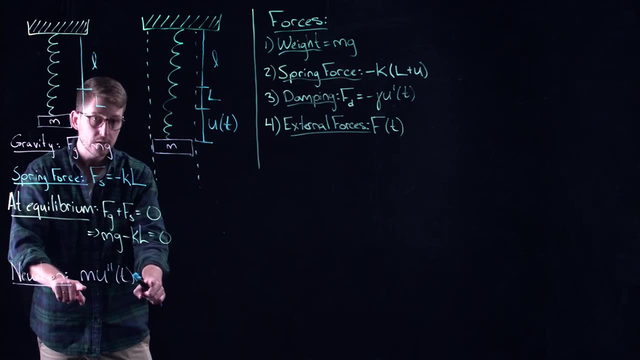 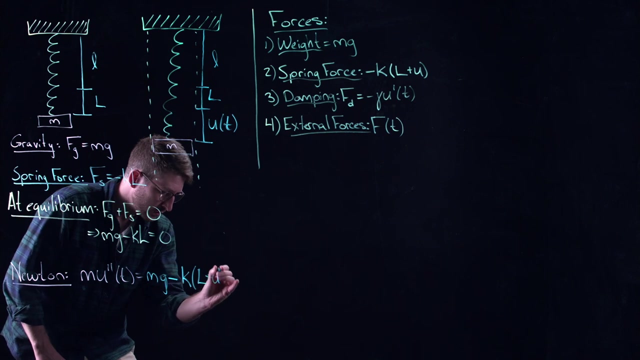 If we sum them all up, in this case we are going to get again from Newton: mass times. acceleration is equal to the sum of forces acting on us. So first one weight, mass times, gravity. Then the second one is the spring force. 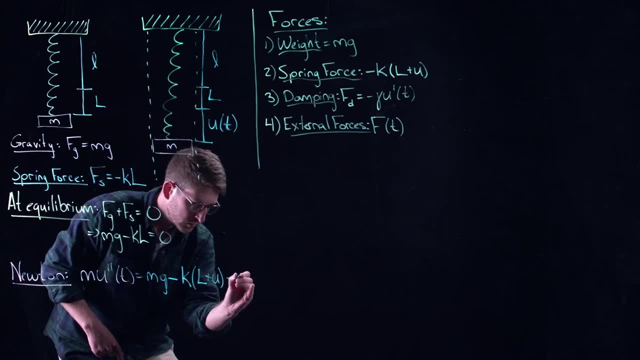 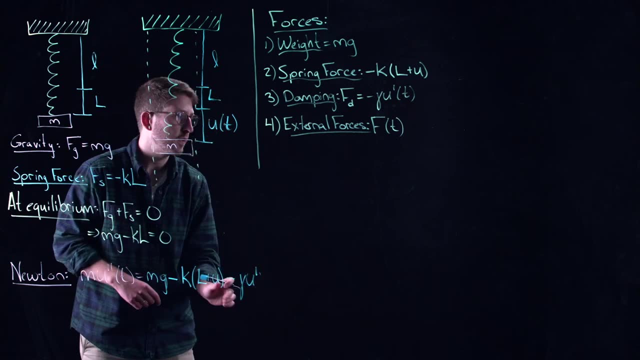 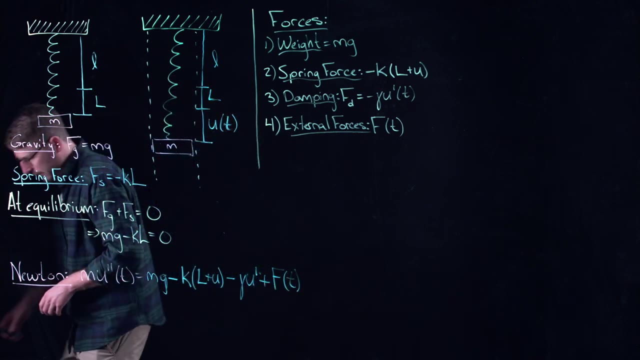 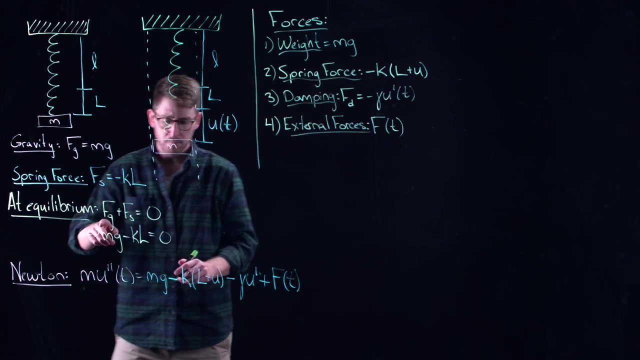 And then the damping force- And then I won't put the T in on this side, just because it will make it uglier- And then plus the external force. Okay, So now what we can do is we can rearrange this, And what I want to use is the equilibrium point here. 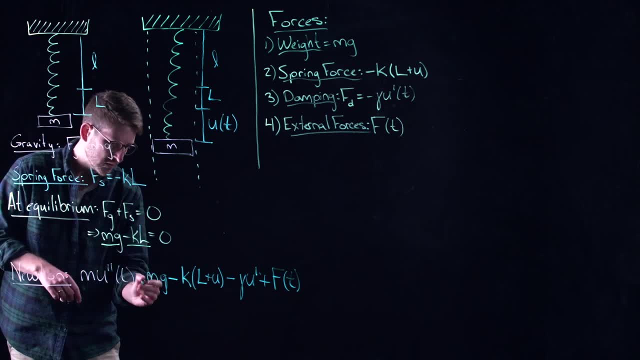 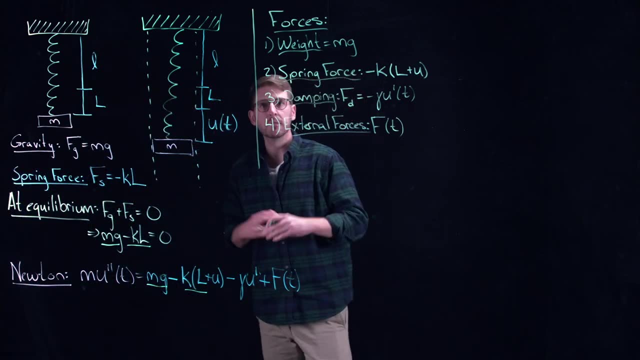 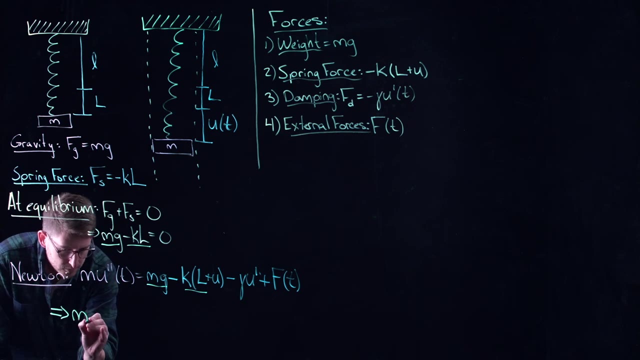 So I know that Mg minus Kl is equal to zero. Mg minus Kl, That piece is equal to zero. So I'm going to write this in the way that we've been writing differential equations all along: All of the dependent variables on the left-hand side. 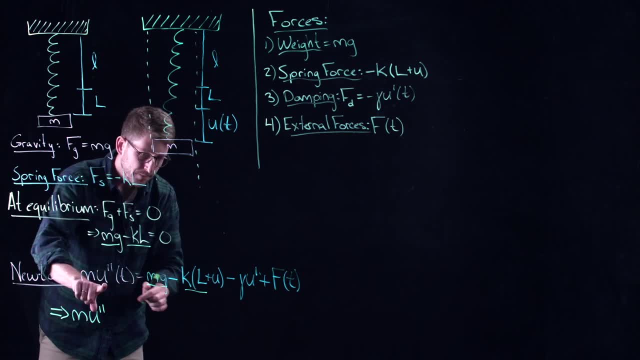 So that's all of the u's, So Mu double prime. Now this comes over and becomes plus Ku, And this comes over and becomes plus gamma u prime. So I get plus gamma u prime, Plus Ku, And then this is equal to some external forcing. F of T. 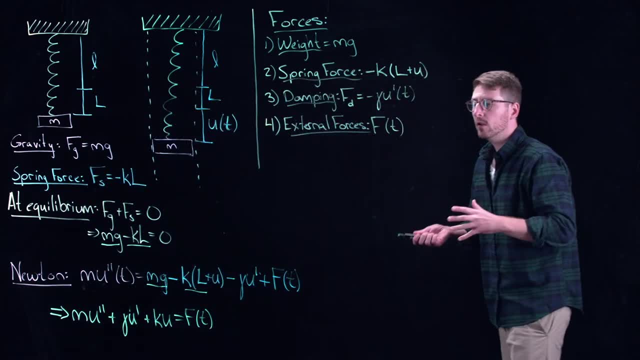 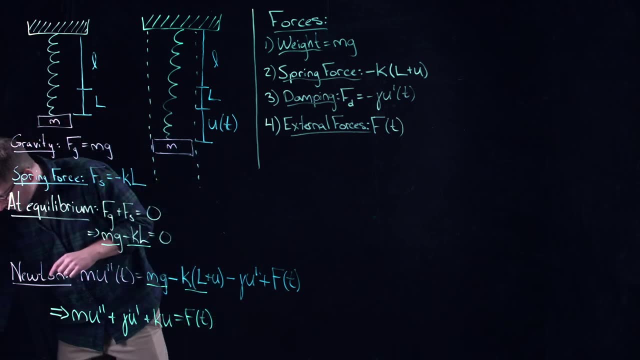 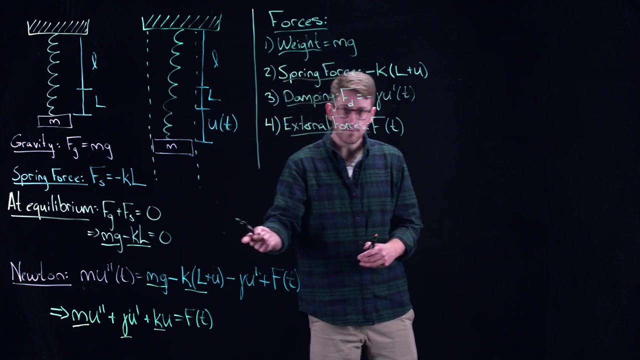 That is my most general equation to describe this mass spring system. Now what I really want you to notice here is I have constant mass, Constant damping coefficient gamma And constant spring coefficient K. So this is a second order differential equation that is linear. 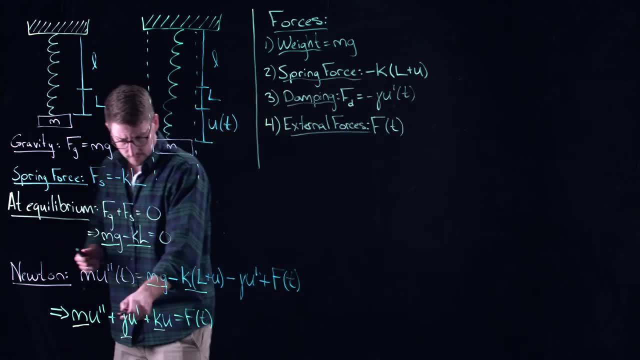 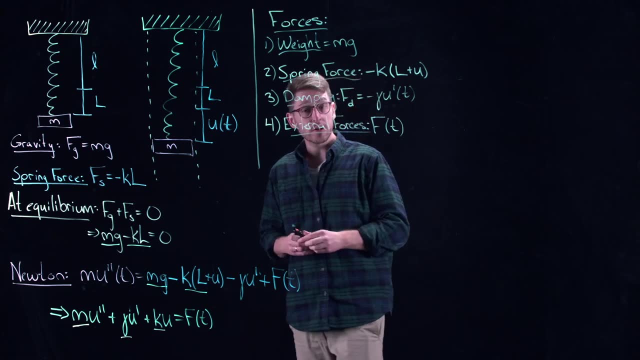 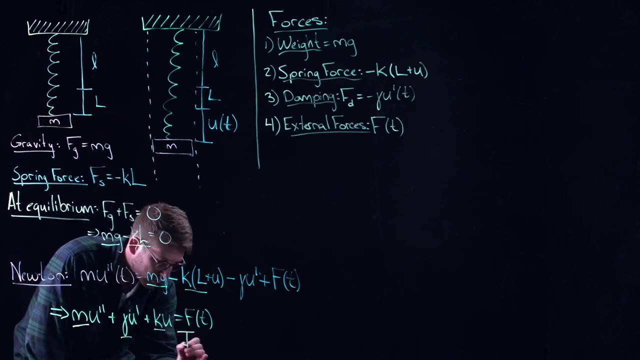 That's fairly obvious. And all of its coefficients are constant. It's a constant coefficient equation. That means that it has a characteristic equation And that means that we can analyze it. And the last piece of this is that I can turn this into an initial value problem. 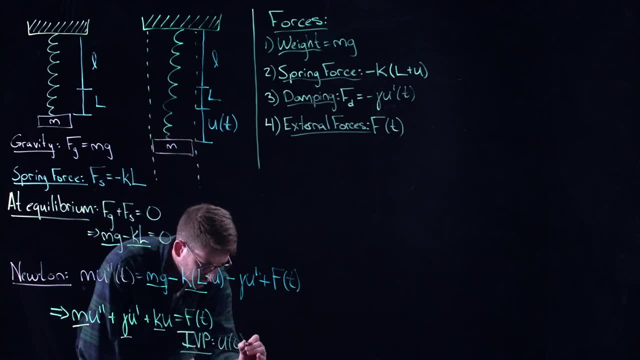 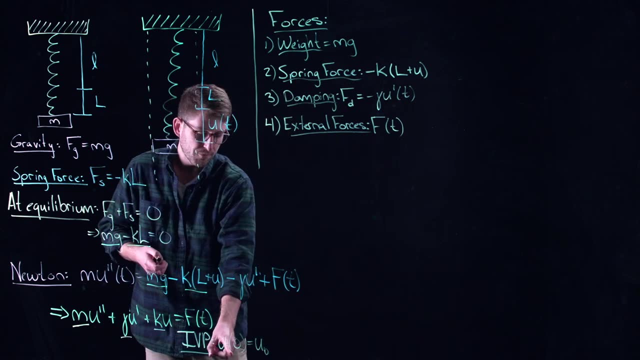 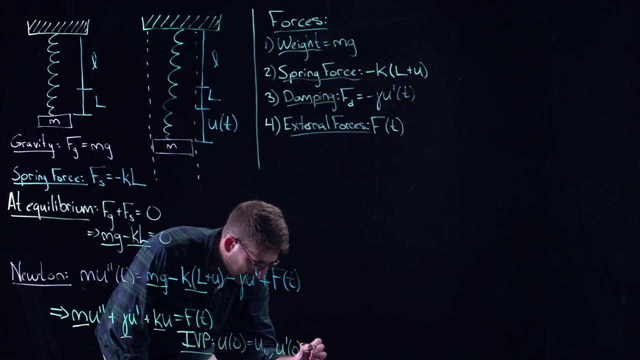 If I know the initial position Of this thing. So maybe Again, if I'm thinking of my example, pulling it down and letting it go, How far I pulled it down from equilibrium? And I also need to know Its initial velocity. U prime of v zero. 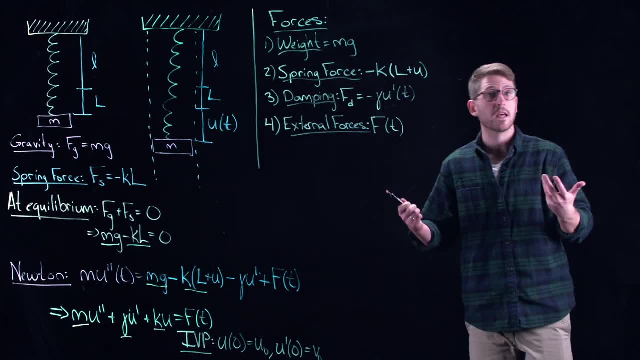 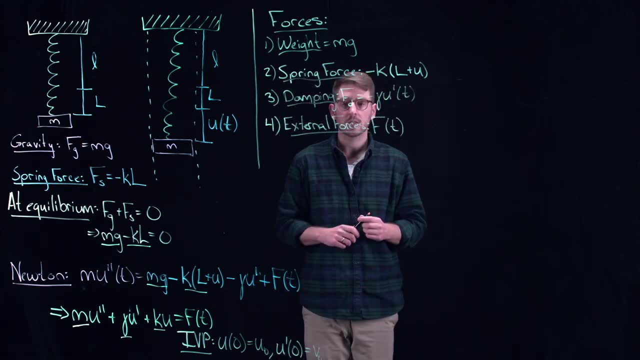 U prime of zero is equal to, in my case, v zero. I'm just using that to denote the velocity. So this would constitute a well posed second order differential equation. So here's what we're going to do for the remainder of the lecture. 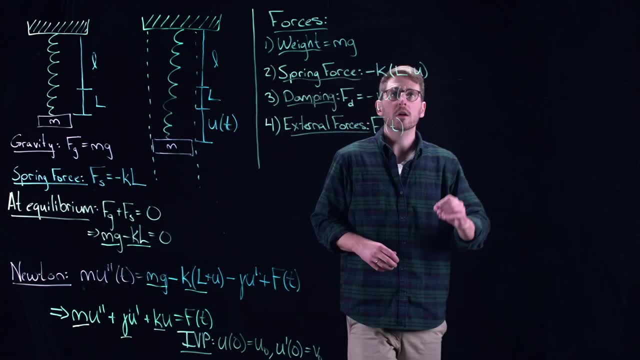 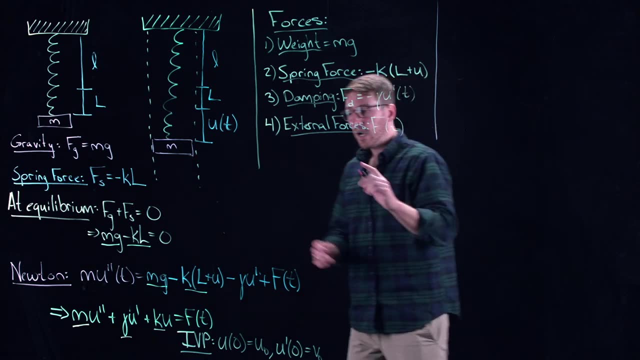 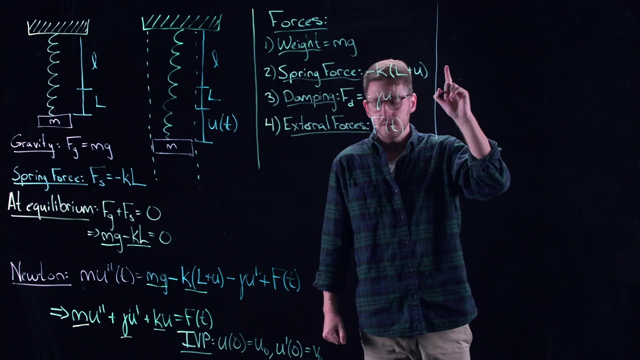 We're going to walk through this differential equation And we're going to look at a bunch of different cases here To better understand what's happening, And I'm going to slowly build in more pieces as we go through. So the first thing I want to look at is undamped free vibrations. 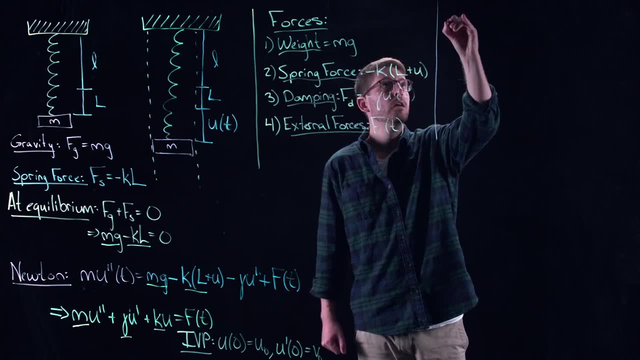 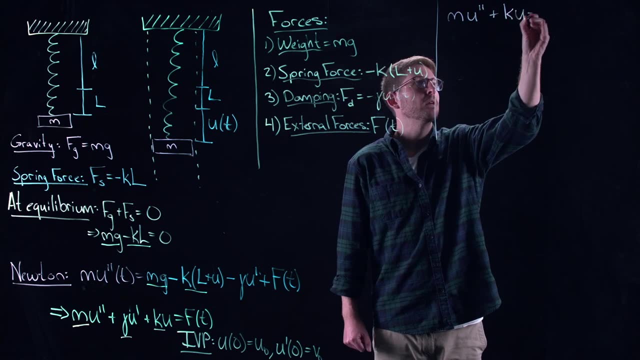 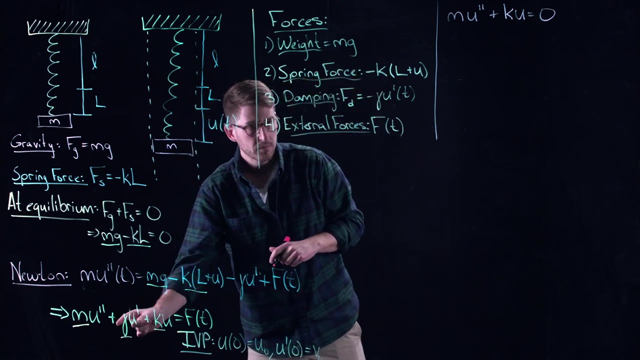 So let's take a look at this: An undamped free vibration, Okay, so what does that actually mean? Undamped means no damping, So that means that I'm not going to consider this term, So I'm going to imagine there is no, say, air resistance. 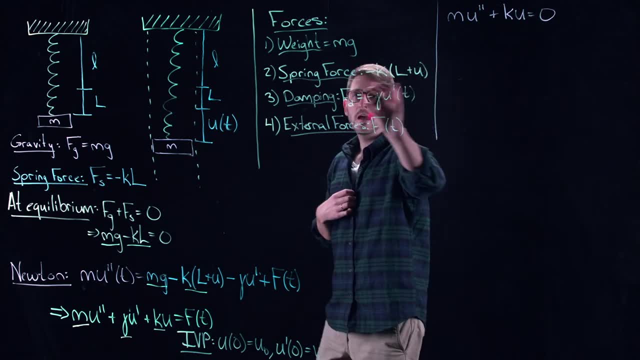 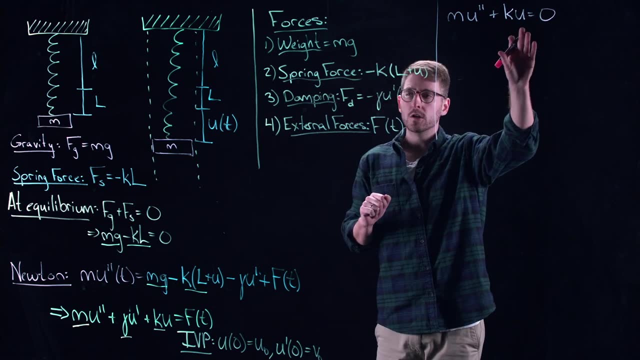 Water resistance, Honey resistance, Friction, Whatever that thing happens to represent. We're not including that in the forces. Now, the free vibration part of this Comes from the fact that there's no external forces. This thing is a closed system. 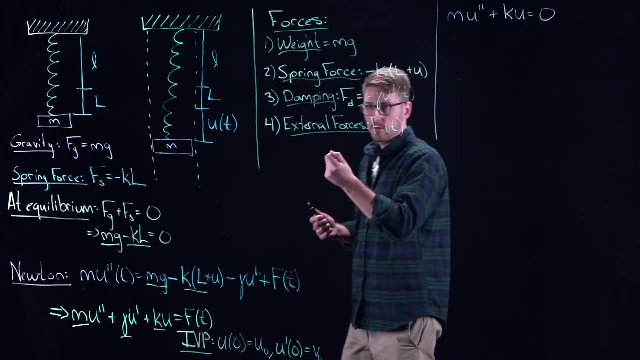 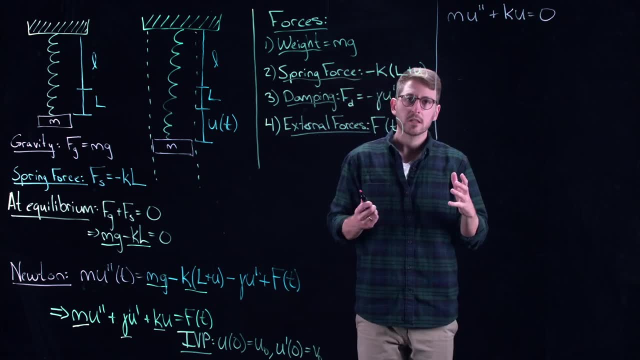 Nobody is affecting this model. Okay, so the only thing that can happen Is that the mass and the spring Are sort of bouncing and interacting with themselves, And that alone. Nobody is shaking this thing. There are no external forces being applied here. 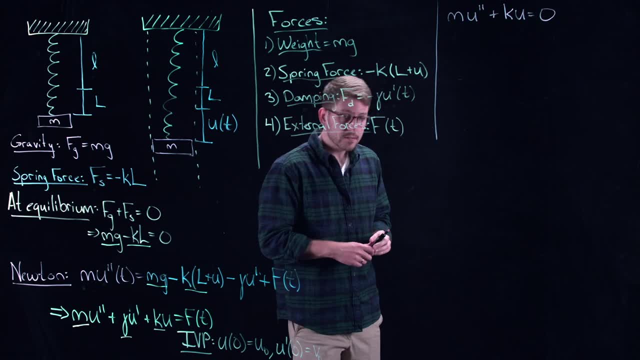 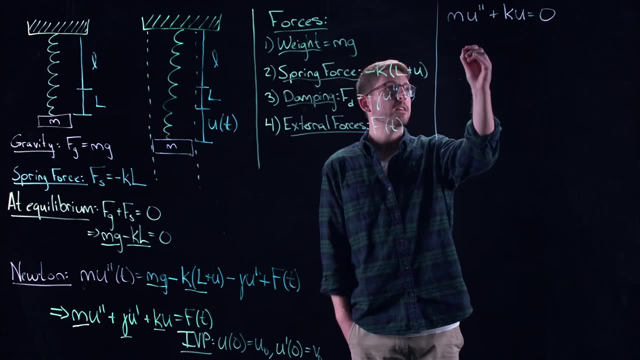 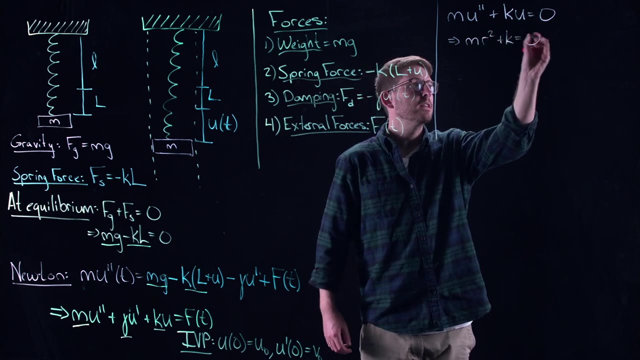 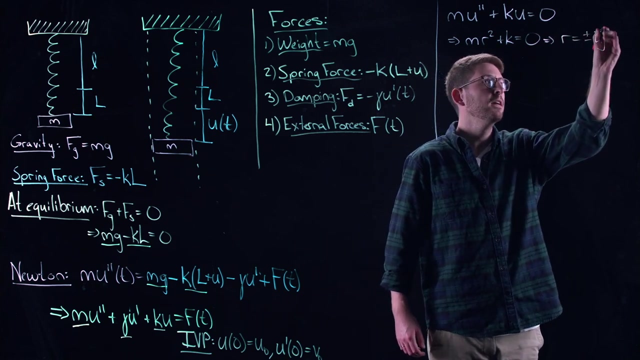 This is a very, very nice little differential equation. Second order, Constant coefficient, The characteristic equation for this thing. So let me write this: MR, squared plus K Is equal to zero. This gives me R is equal to Plus or minus I. 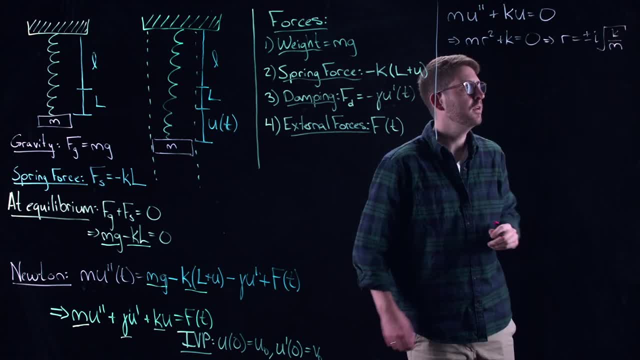 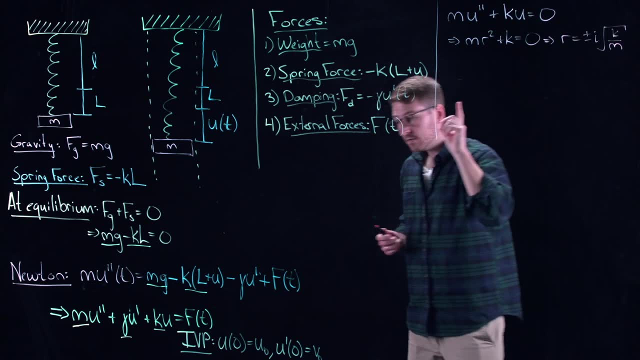 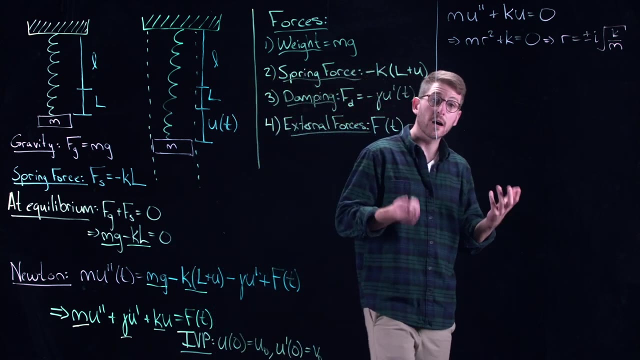 The square root of K over M. Okay, so clearly this thing is imaginary. That comes from the fact that K and M are both positive numbers. So again, M, gamma, K, Always- are going to be Positive. in the case of gamma, It's going to be non-negative, right. 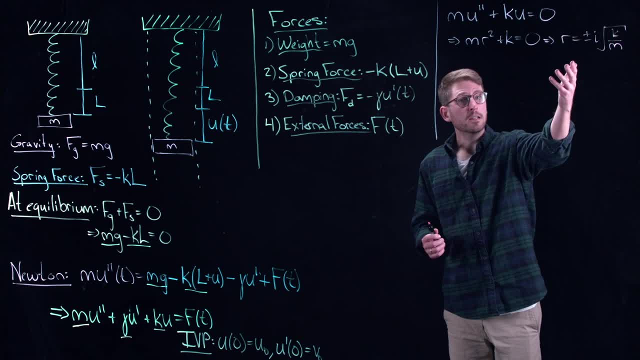 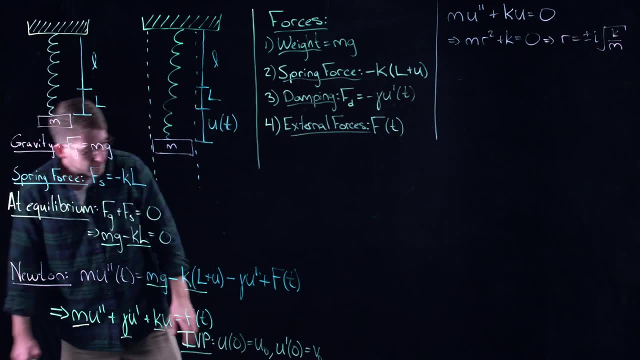 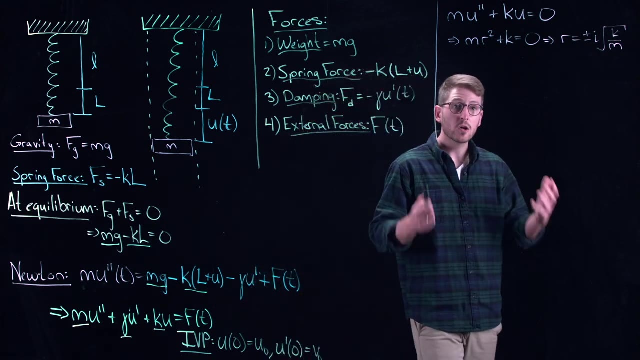 We're allowing for zero value there, But This gives purely imaginary roots to our characteristic equation. Now We know what imaginary roots do, right, We know that they lead to oscillations. Oscillations means Sine and cosine. So the general solution of this thing: 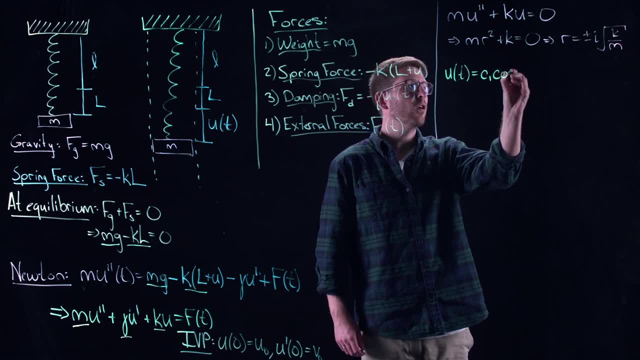 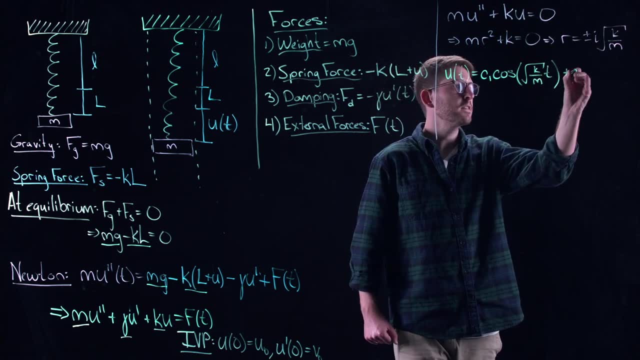 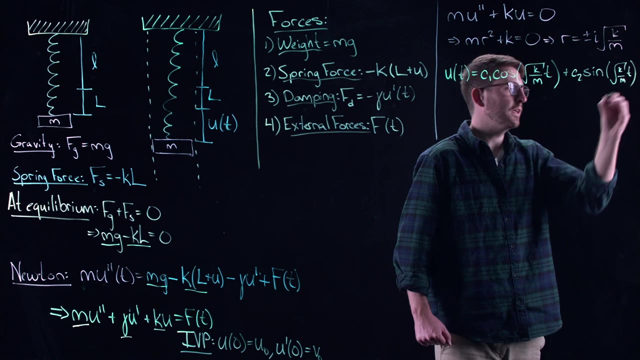 U of T is C1. Cos, The square root of K over M T Plus C2. Sine, The square root of K over M T. There's no exponential terms And that's because there's no real parts here. 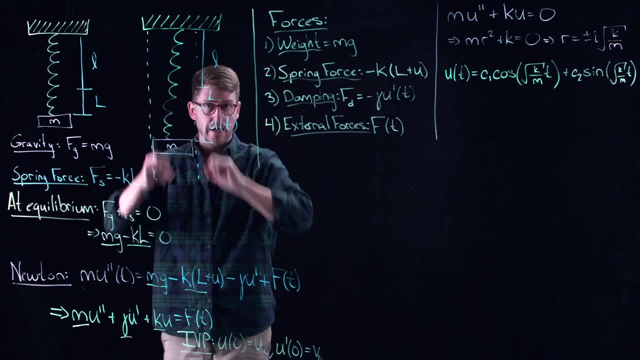 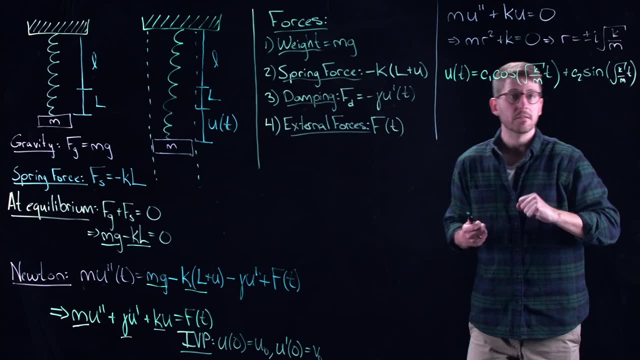 So let's think about what this means In the context of my mass spring system Right here. What does that tell me? Well, These things oscillate forever. Okay, There's no other dynamics taking place here. They never go to zero. 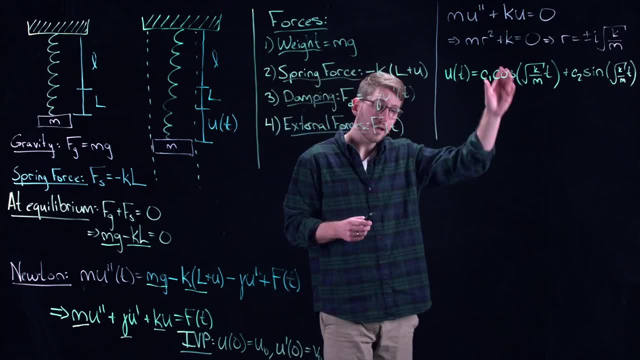 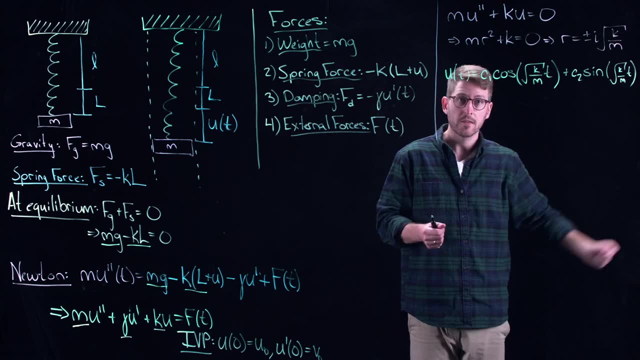 All they do Is just oscillate, Nice little sine and cosine waves added together, You know again, they just look like a little sine or cosine wave Up and down, That's it. So what does that mean here? Well, Once I put in my initial conditions, 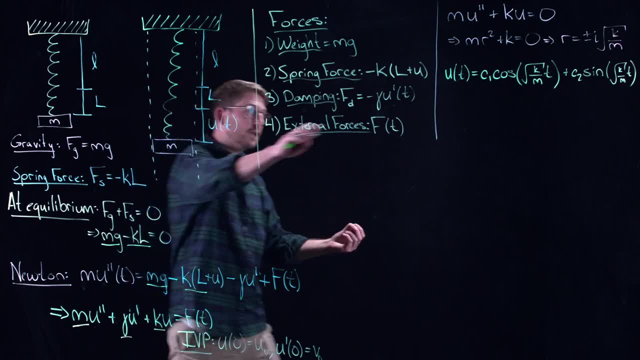 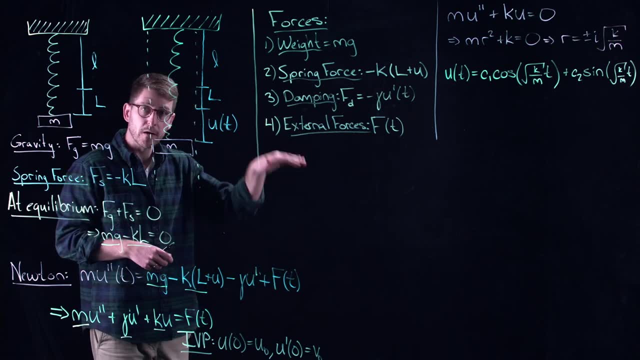 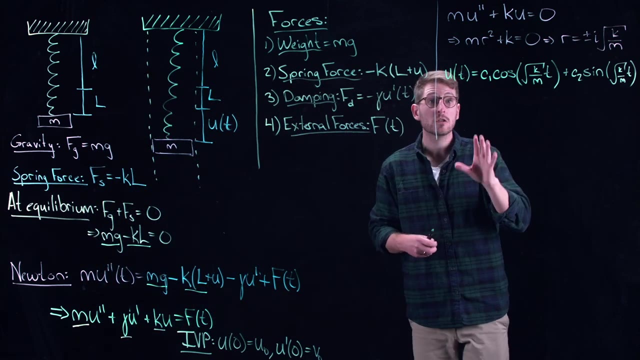 If I pull this thing down, U of T is just going Up and down forever. So what does the mass do? It just goes up and down forever. Nothing else, Right? And now you might be thinking yourself: Well, Jason, I can imagine doing this. 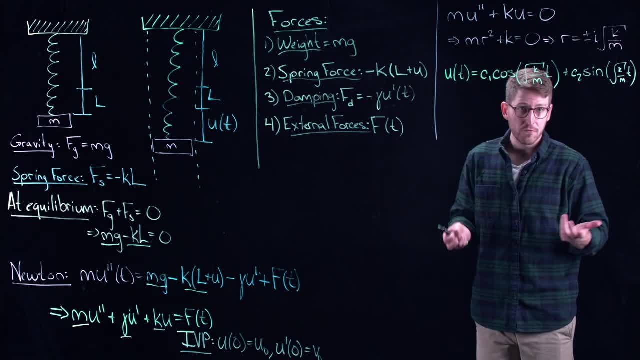 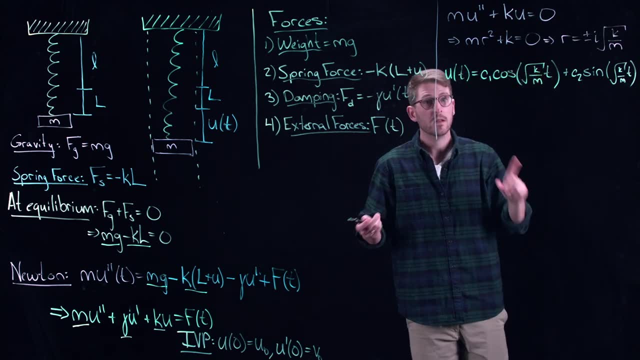 Right, Maybe I built this in my basement. It's not going to go forever. I know it's not going to go forever, Right? Eventually, you know, if I walk away for two days and I come back, It's going to settle down. 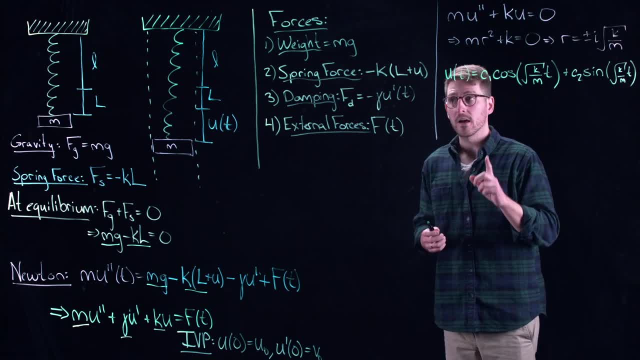 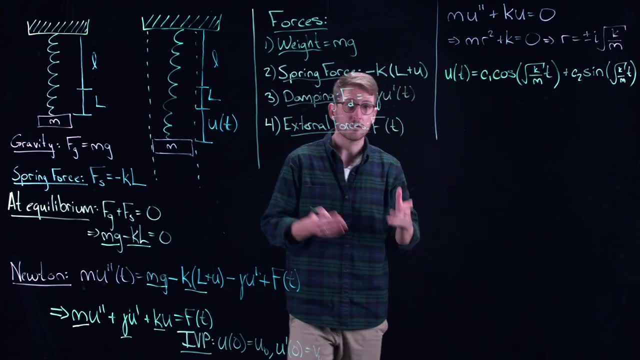 I agree, But we have done this in an extremely idealized setting. Again, we're doing it in a vacuum. There's no air resistance taking place here. It's the air resistance in your basement that you might be doing this. It's eventually going to slow it down. 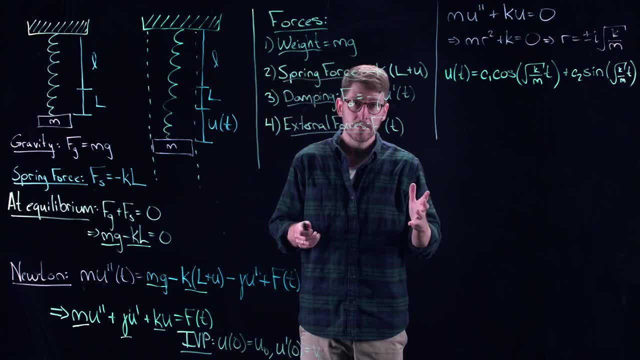 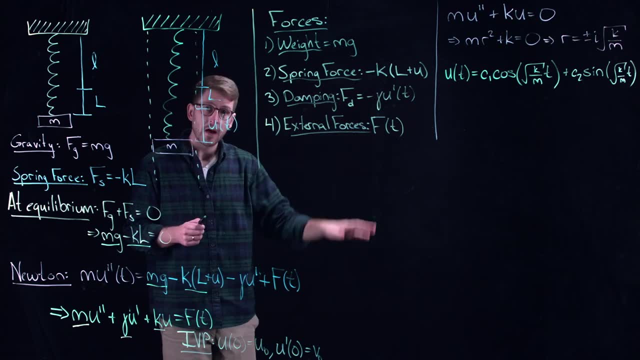 We're not accounting for that because we're not accounting for damping. So if you do this in a vacuum with no external forcing, What's going to happen? Just going to go up and down forever. It's going to be a nice little pendulum here. 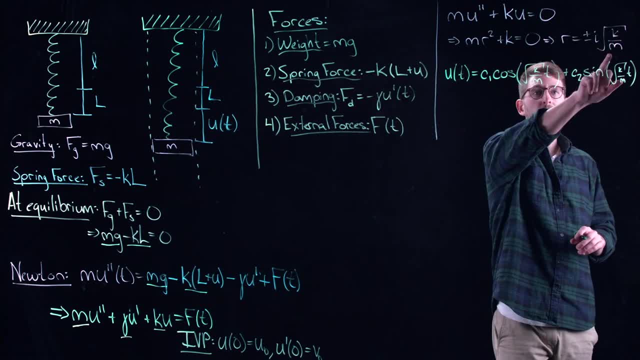 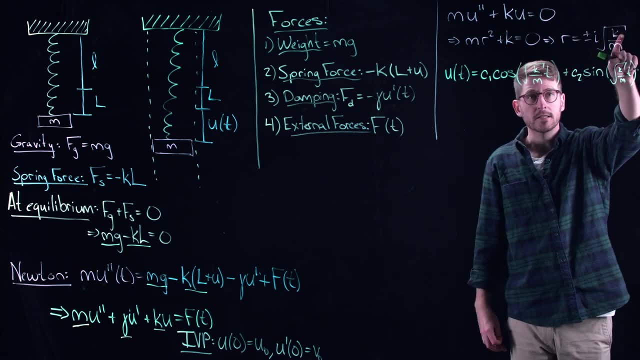 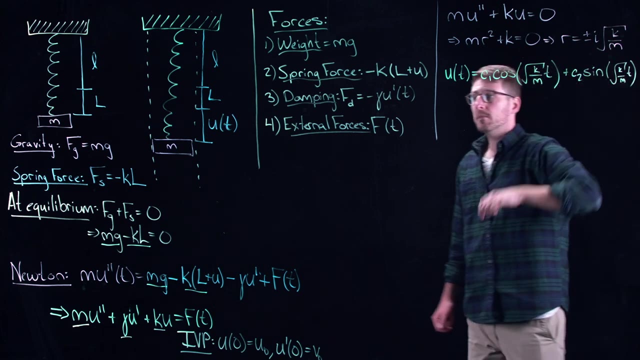 And what you can see is that we can account for the frequency of oscillation. It's essentially the sort of tightness of the spring, That's, a spring constant K Divided by the mass of the object. So if the mass is lighter, 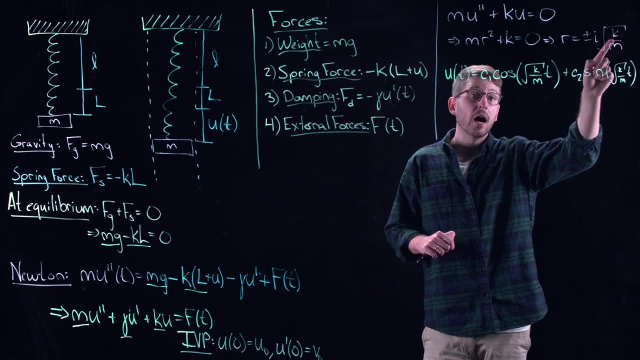 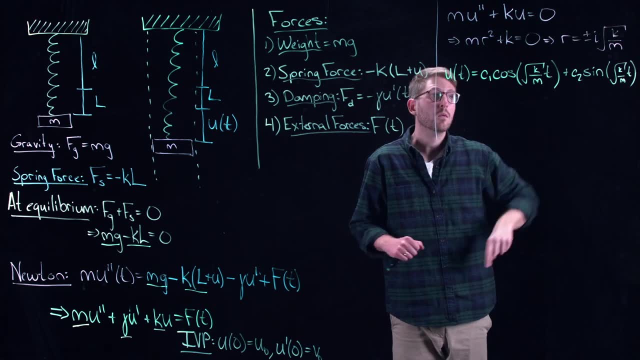 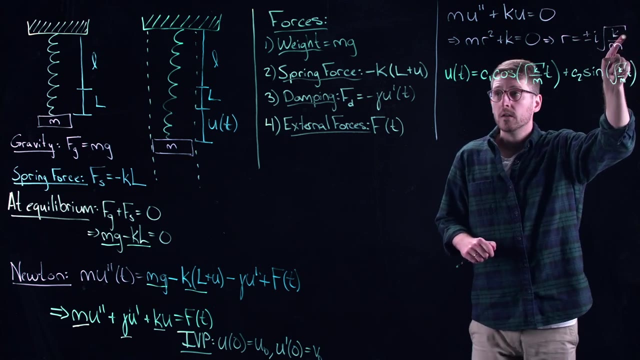 So if the mass is smaller, Then you have a higher frequency And you have a shorter period, So the oscillations are going to happen very, very quickly, Whereas, similarly, if you have a tighter spring, So if K is bigger- Then the frequency is going to get larger. 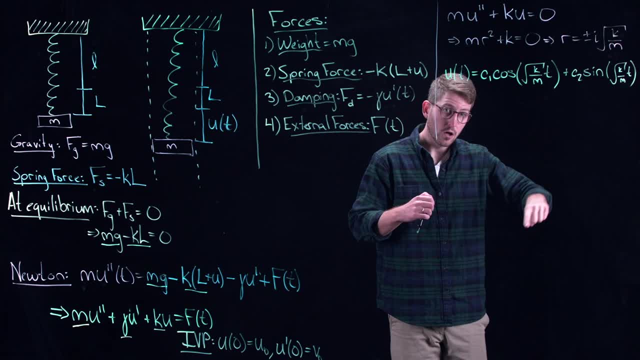 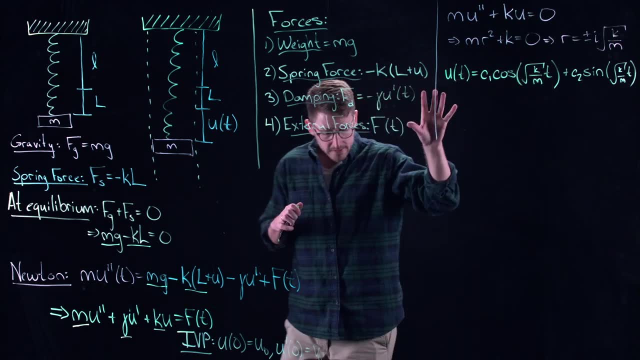 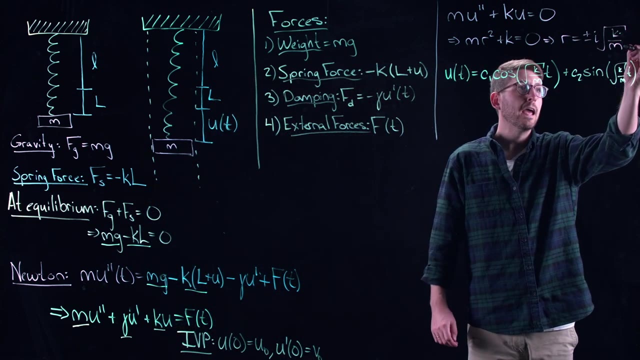 And that means that you are going to have long and slow oscillations. That gives you a longer period. So you can see that we can actually derive the sort of expected dynamics out of this thing, Just by knowing the spring constant and the mass of this thing. 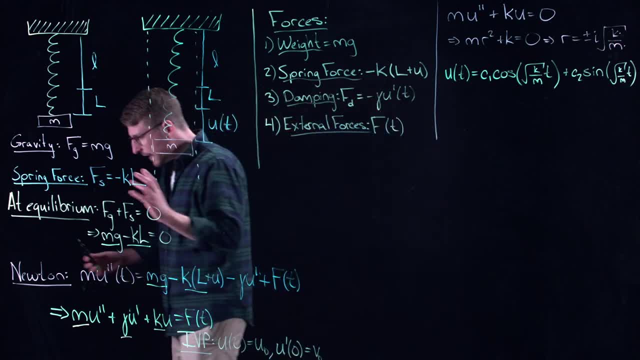 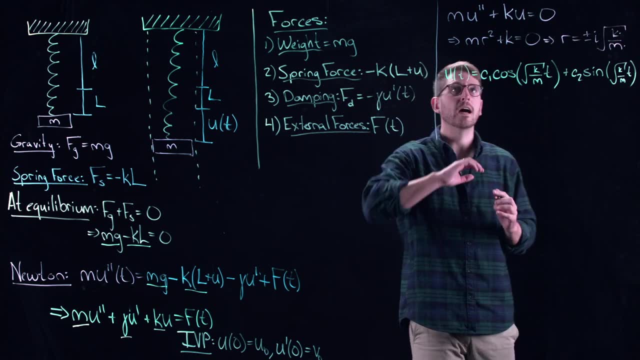 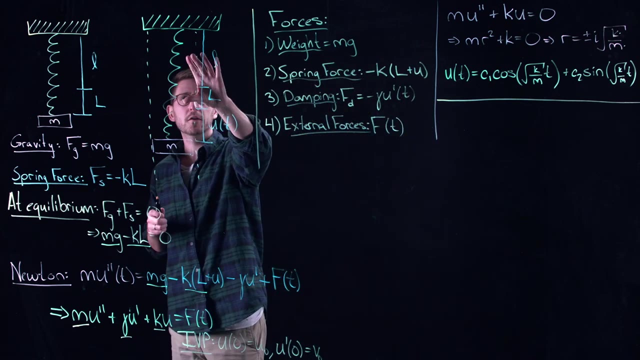 Now, of course, maybe you're not really that impressed. Again, you said, Jason, I do not have access to a vacuum, So I clearly cannot run this experiment, But I probably could go on Amazon or eBay And buy myself a spring And maybe, you know, attach some little weight to the bottom of this thing. 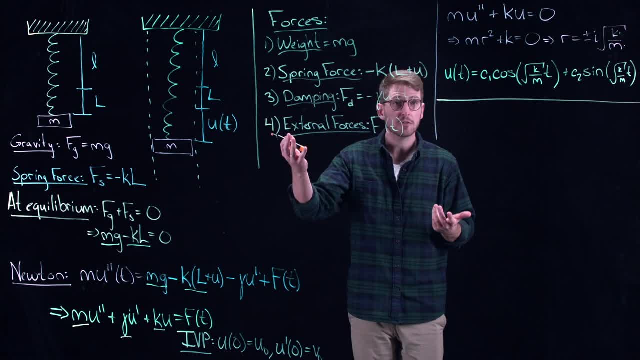 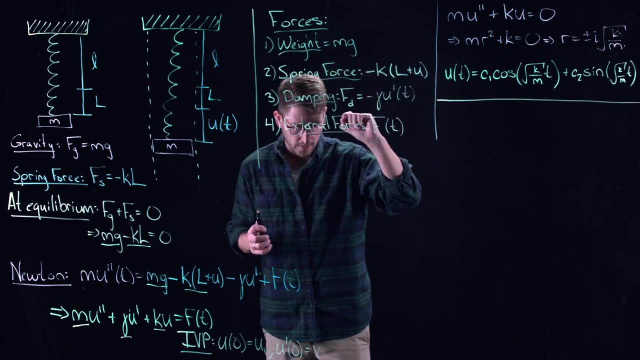 And so in theory, I could actually do this experiment right. This is probably a hundred dollar experiment at the very most. That's not what I'm going to see. What I'm going to see is some sort of air resistance in there. So let's look at another case. 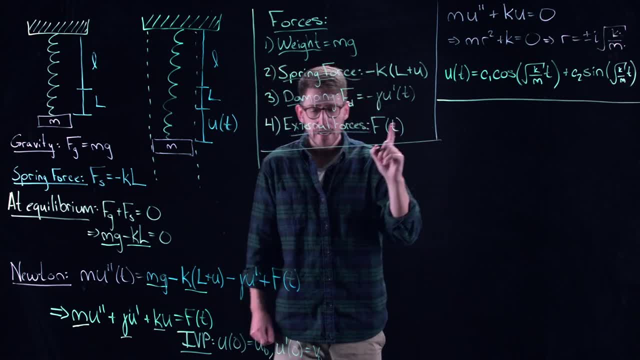 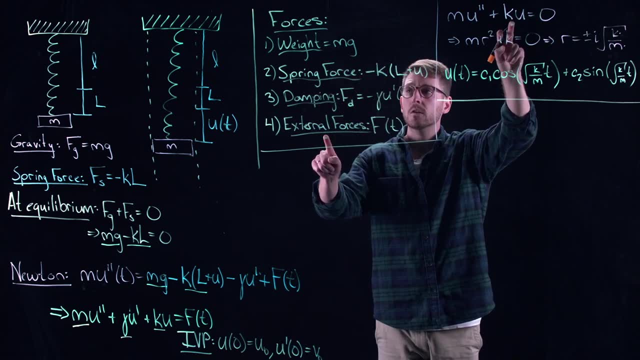 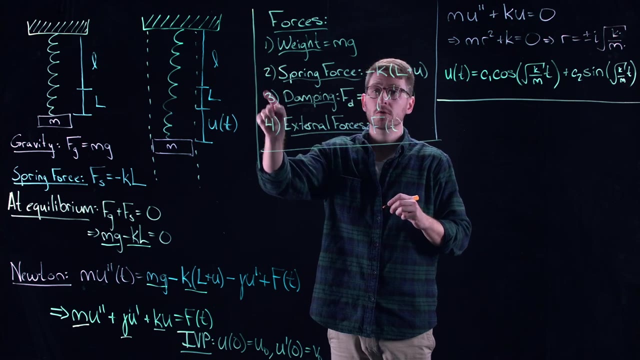 Let's look at the case of what are called damped free vibrations. Remember this was an undamped free vibration. Free means no external, Undamped means no damping. So if it's going to be damped but still free, That means I get one, two, three forces acting on this. 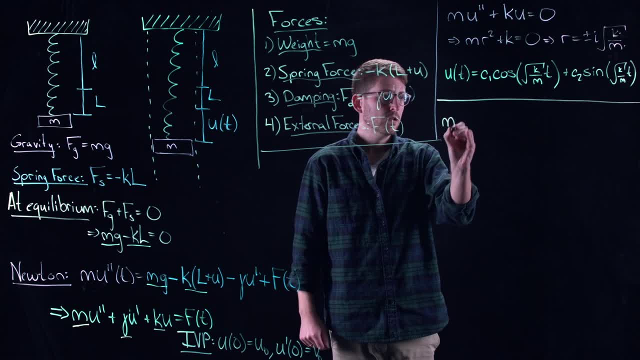 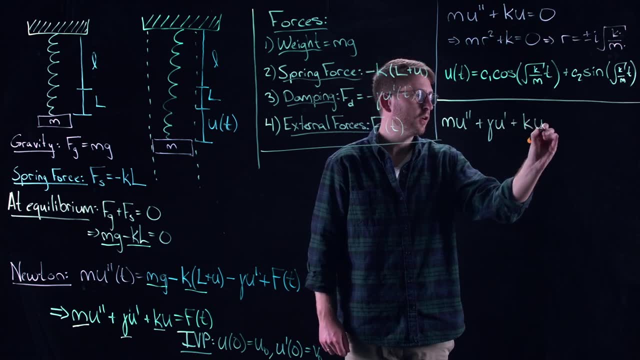 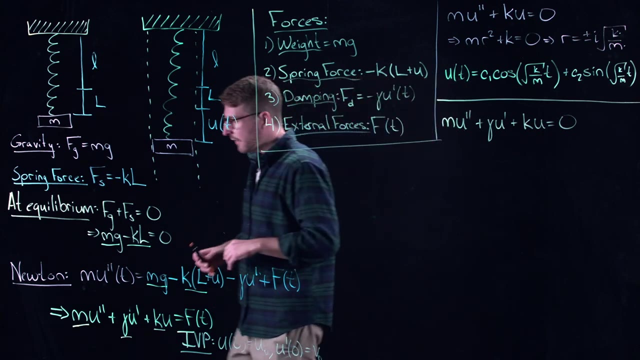 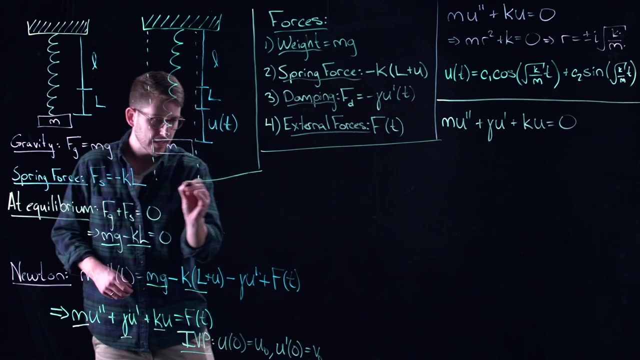 But not the fourth. So I get M? U double prime plus gamma U prime Plus K? U is equal to zero. Okay, Now I've got again a second order differential equation. I still have a characteristic equation. Let's take a look at what that characteristic equation should be. 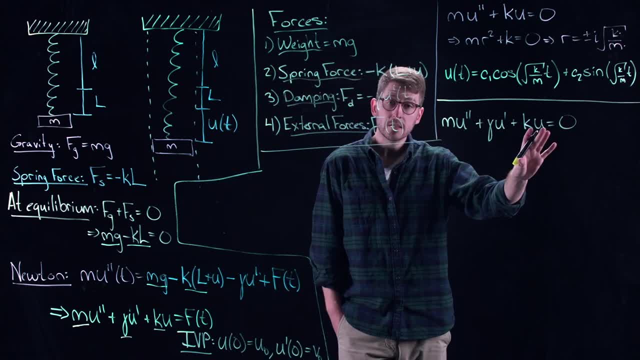 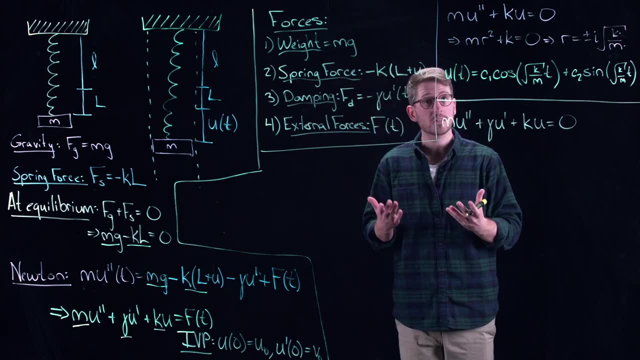 Again, just putting in E to the RT here. Nothing fancy, right? We've been doing this so much that you're probably sick of it. If anything, You could probably do this in your sleep. You might even have nightmares about it, But we can still do it. 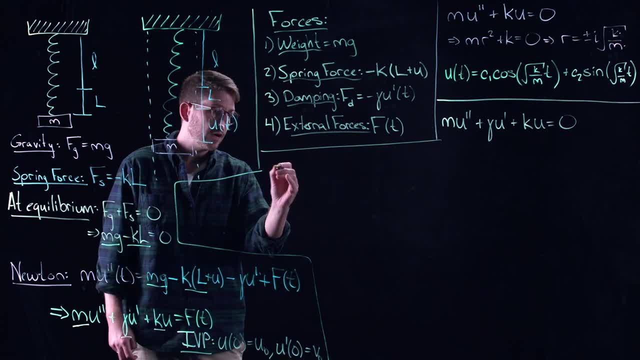 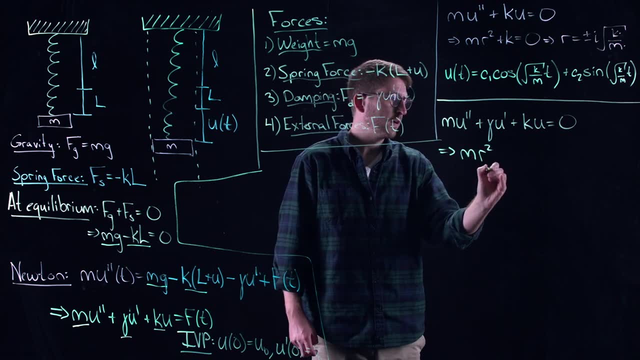 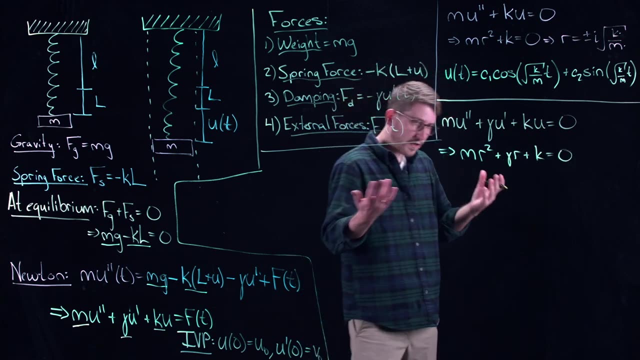 So we can still analyze this thing. So let's take a look. The characteristic equation here is going to be: So let's put it right underneath: M, R squared plus gamma, R plus K is equal to zero. Okay, So you know, it's got some annoying variables in here. 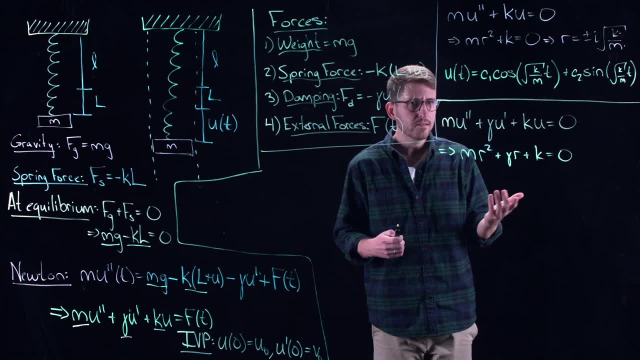 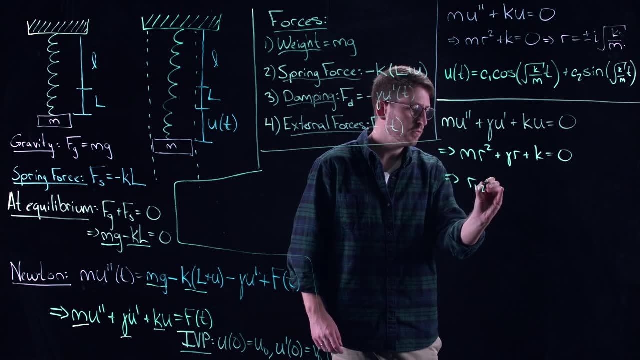 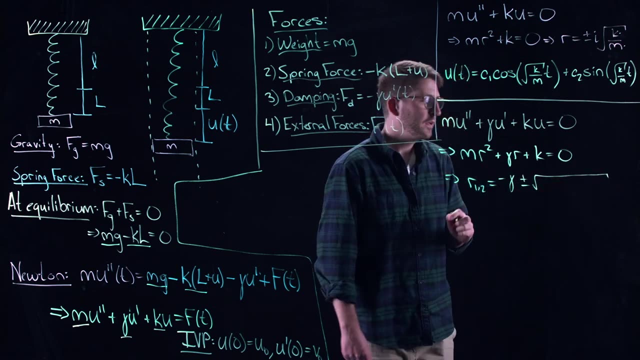 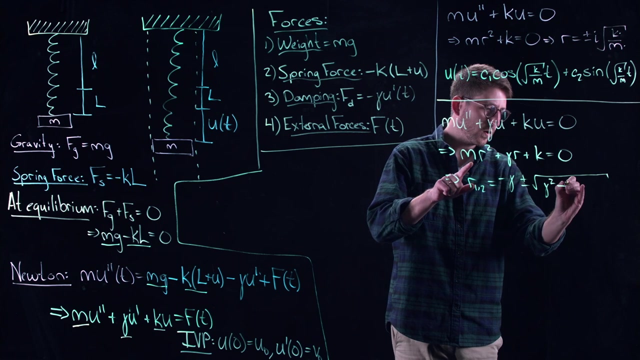 M, gamma and K. But other than that, I mean This is a quadratic equation. I've got the quadratic formula to solve this thing. So my two roots are given by negative gamma plus or minus the square root, And now I have gamma squared minus four M, K divided by two M. 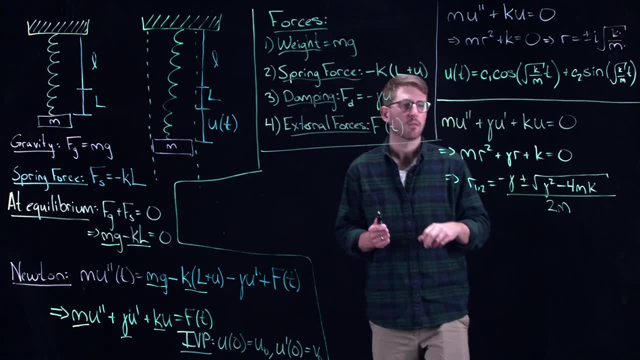 Again, That's just the quadratic formula. Replace your A, B and C by M, gamma and K respectively, And boom. There it is. That's all that you need. So clearly, Some weird things are going to happen here And, depending on, 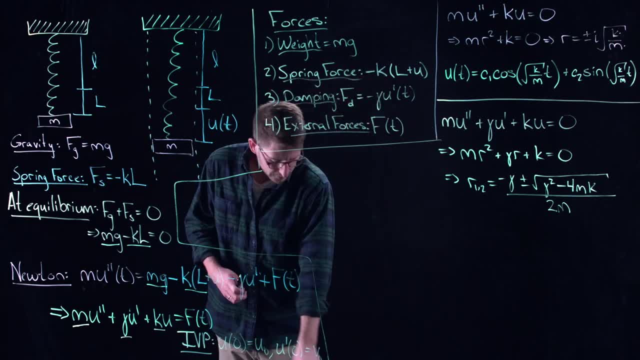 What is going on underneath the square root Right, Remember, this is exactly where We saw a lot of the discrepancies come up when we were analyzing the different cases of our characteristic equations. So What we're going to do Is we're going to. 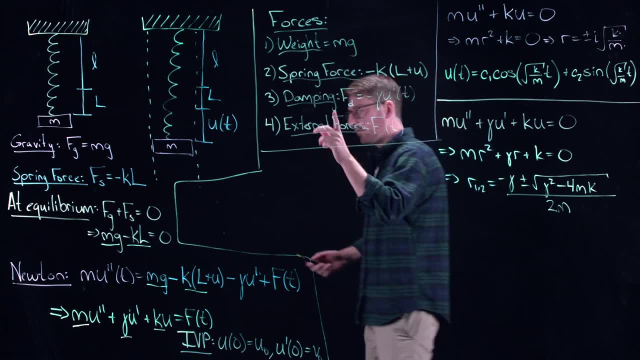 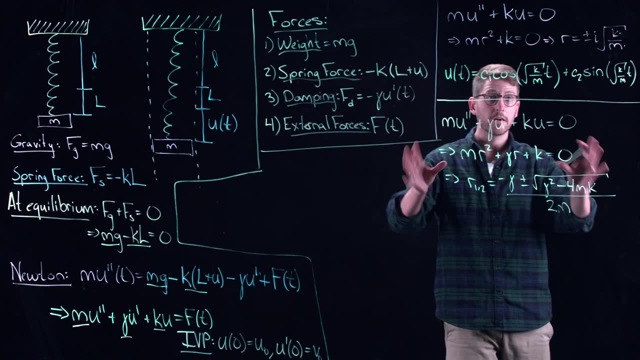 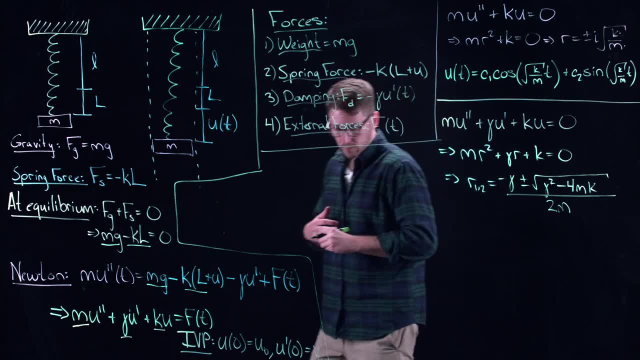 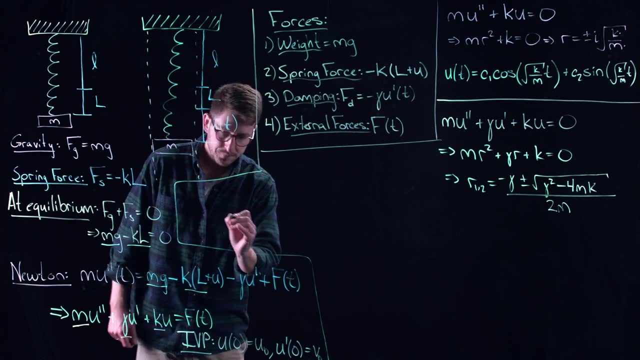 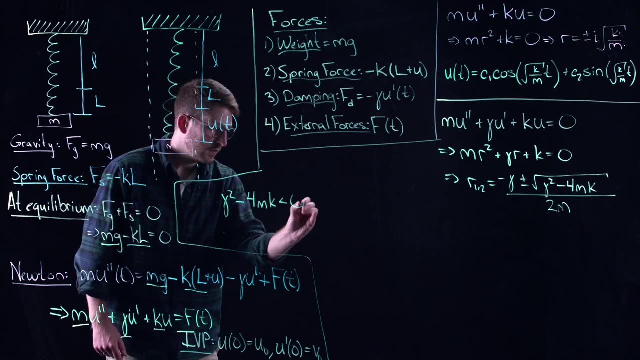 Dwarf Our characteristic equations. So Let's take a look. First thing First. Here's the one that We would be Expecting to come out of this. So this would be gamma squared minus four, M K Is less than zero. 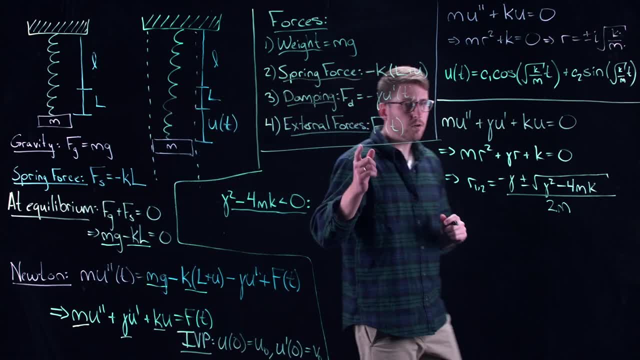 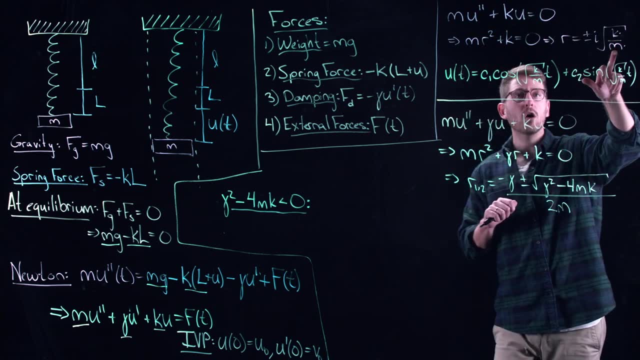 Now, Why am I starting With this one? Well, first of all, Let's think about what happens as we slowly turn gamma on. Okay, so we're going to fix K And M. all we're trying to do is update the undamped free vibration case from right here so we can. 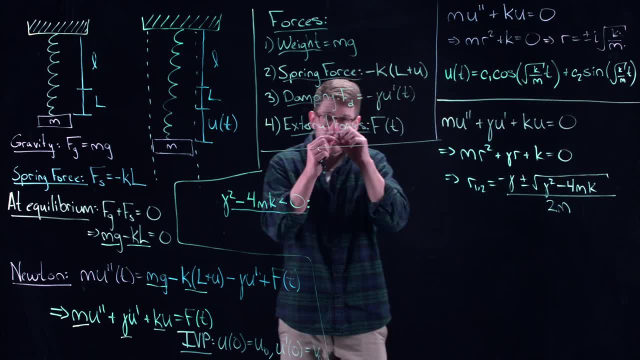 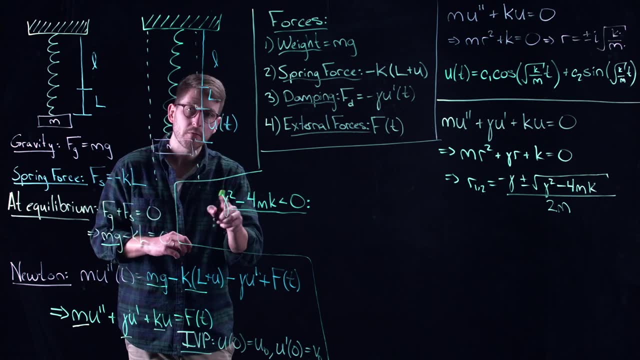 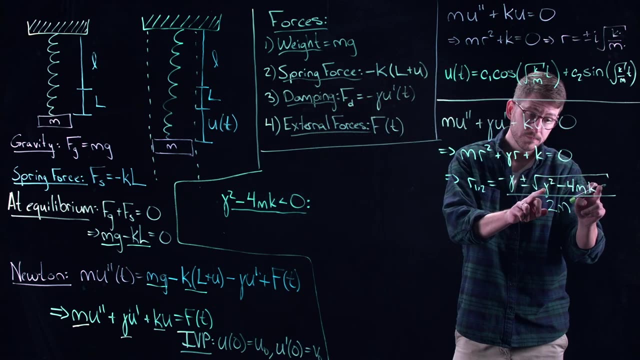 ask ourselves what happens as we slowly turn on gamma. right, so it slowly comes off zero. well, minus 4mk is less than zero. so at least for small values of gamma, this thing is going to be negative. that means that i'm going to have an imaginary part. right, because underneath my square, 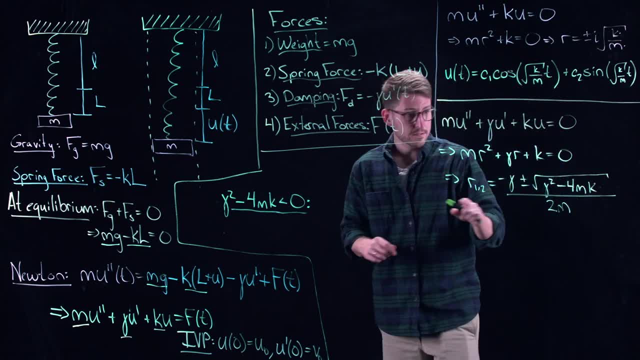 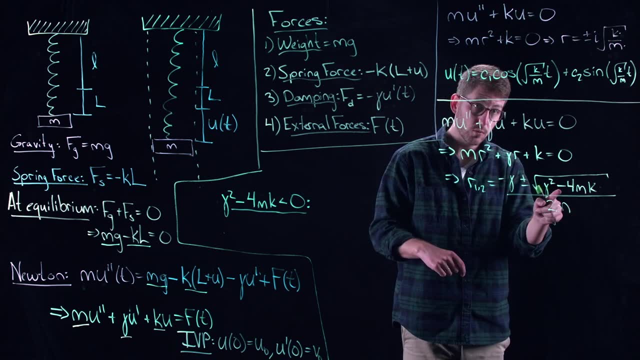 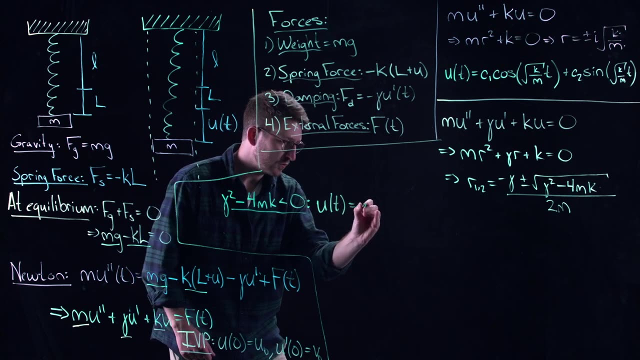 root is going to be negative, and so that gives me a real part of negative gamma over 2m, an imaginary part of 4mk minus gamma squared. let's write down what the solution is here: u of t is equal to c1e. now the real part minus gamma t over 2m. 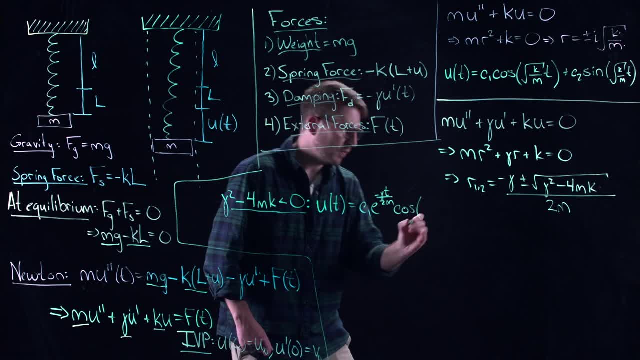 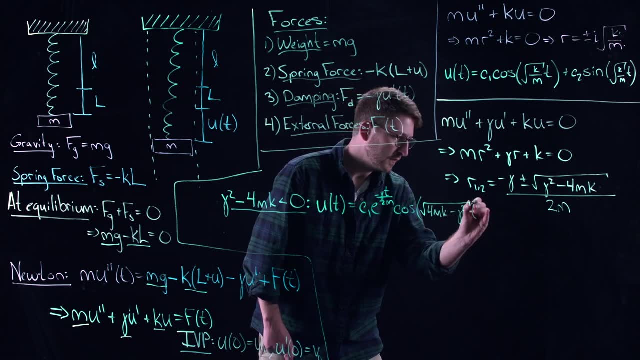 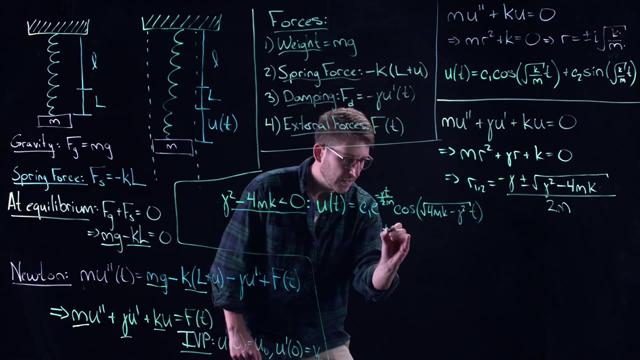 cos. now this, the imaginary orgasm. Sagittarius, part 4mk minus gamma squared t. Don't get intimidated by this. I know it looks daunting, but it's not right. It's just sort of taking care of all of the little variables here, right? 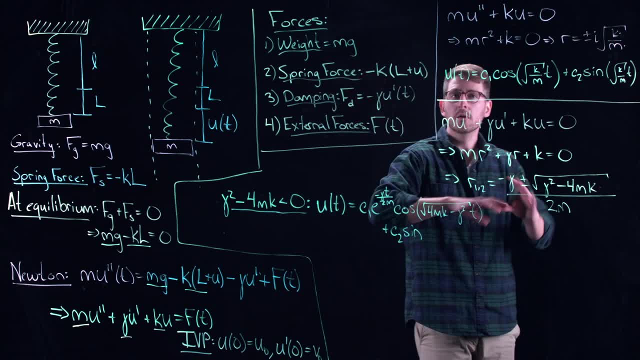 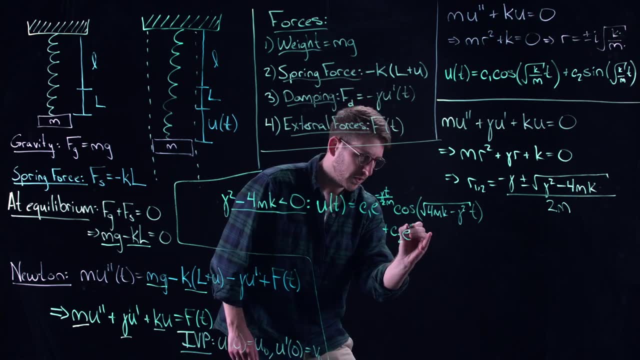 But if you put in numbers for these- maybe 1,, 2,, 3, then you'll see what I'm talking about. right, All of this will work out. So then I have the exponential part here: 2m sine. 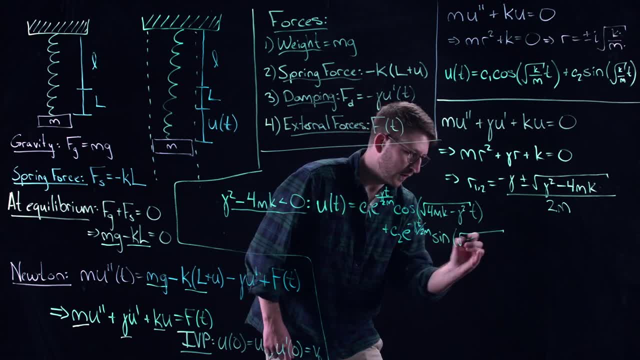 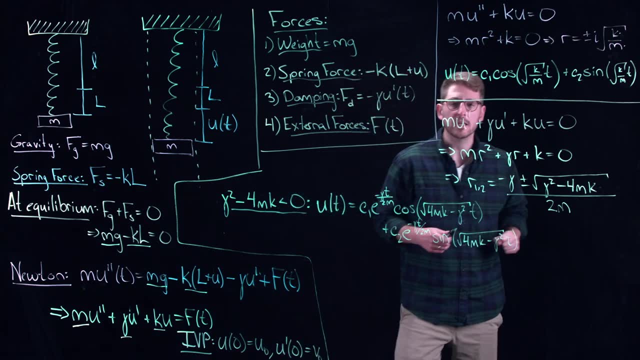 and then the square root of 4mk minus gamma squared t. And so what's happening here? Okay, let's just analyze this case. Sines and cosines still getting oscillations, right, But what's happening to those oscillations? 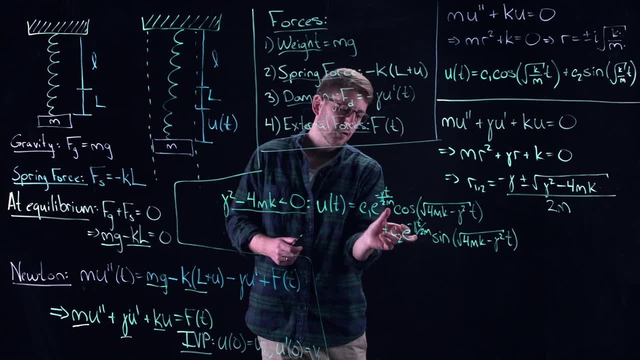 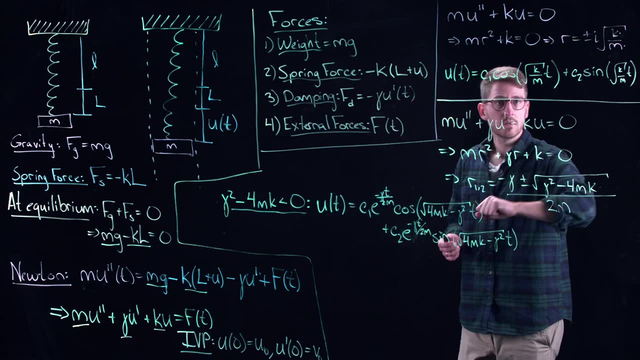 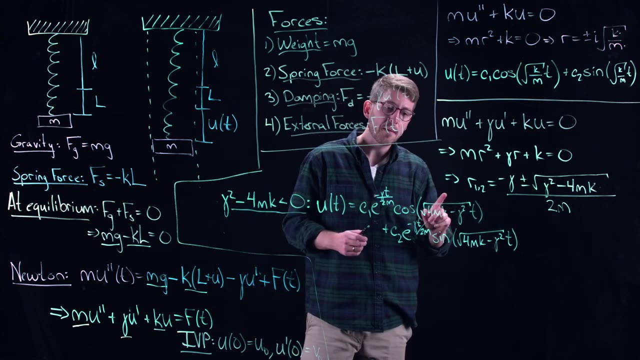 They're being sunk right. They're getting this exponential term multiplied into them, Because gamma and m are positive, this is a negative exponent on the exponential and that thing is pulling it into zero. So what's happening? We're getting what are called 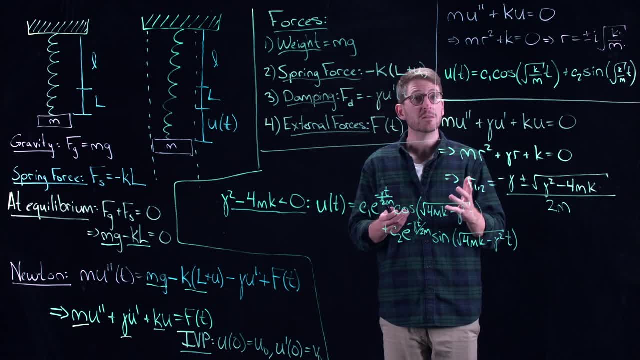 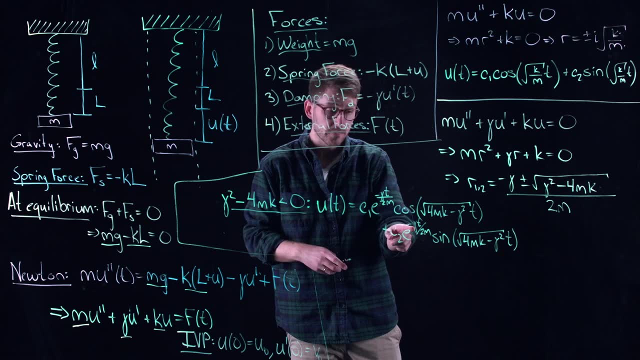 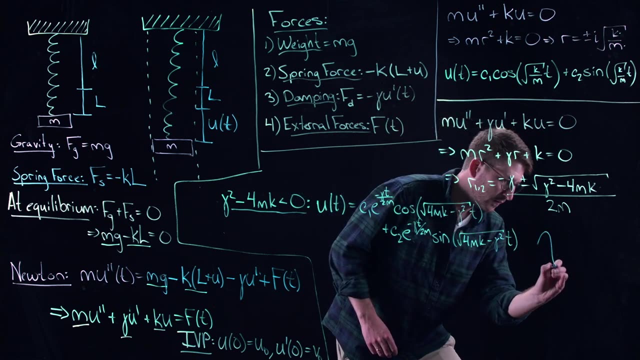 damped oscillations. Now, it shouldn't be a surprise that we call these things damped oscillations, because they are due to the damping right. It's the gamma that's causing this in here. So what do these things actually look like? Well, roughly, they would look something like this: 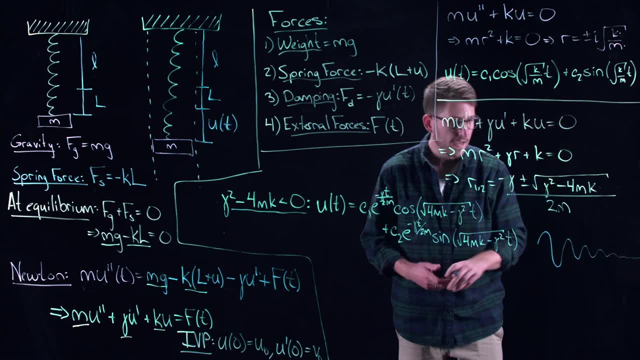 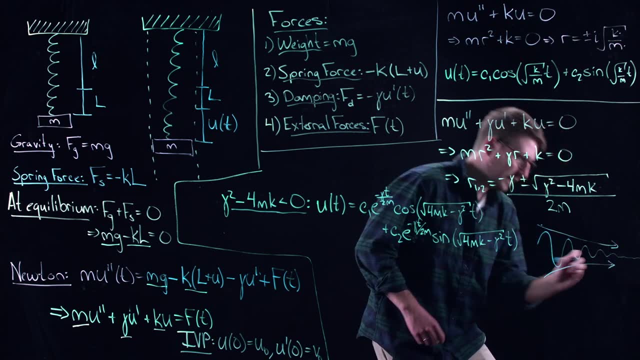 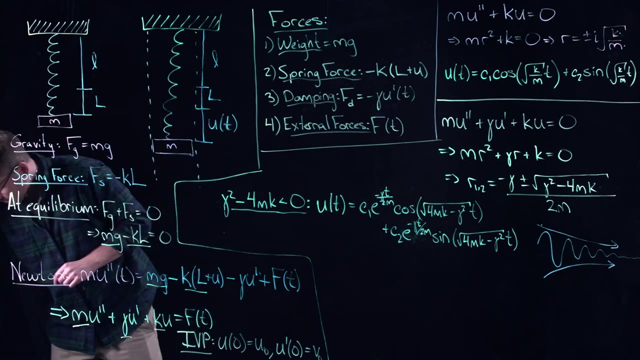 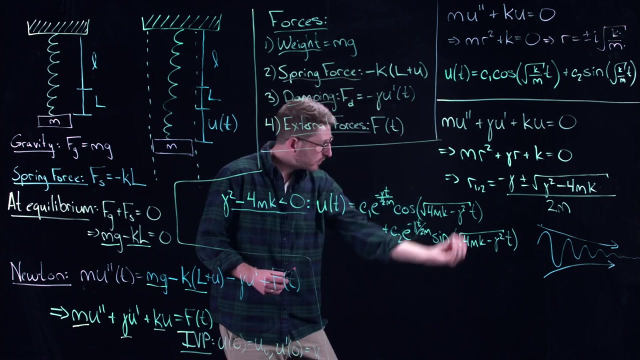 So they are slowly, slowly, slowly decaying oscillations. We can see here that we get this decay in these terms, and that's coming from the exponential. So what does this represent in terms of my spring mass system? Well, now I've got a little bit of air resistance. This is the case where you pull that mass down. 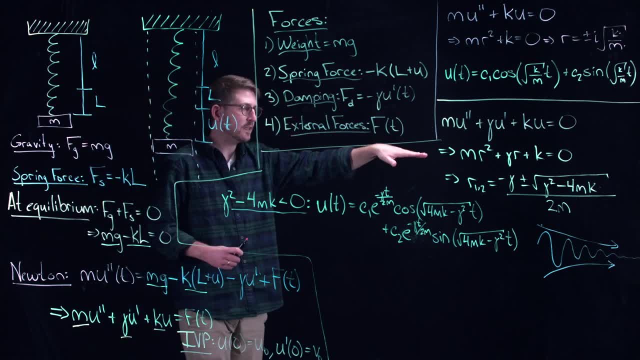 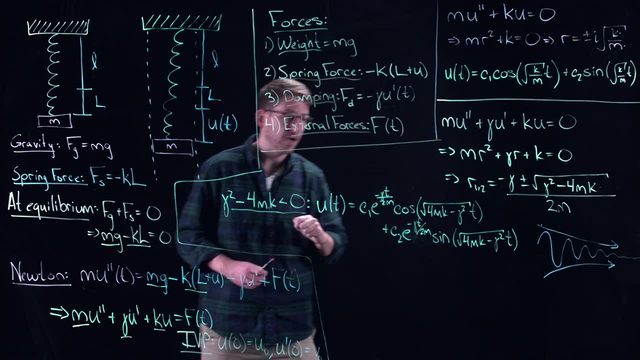 maybe I leave the room. I come back in two days and I see that it's balanced at the equilibrium, right? That's what's happening right here. right That in-between period, it's going down and it's coming up, but not as high as it was before. It's going down. 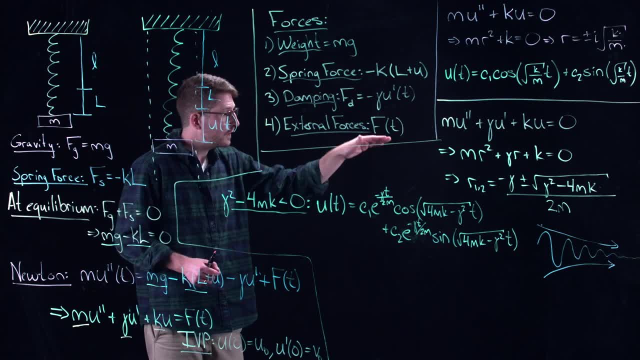 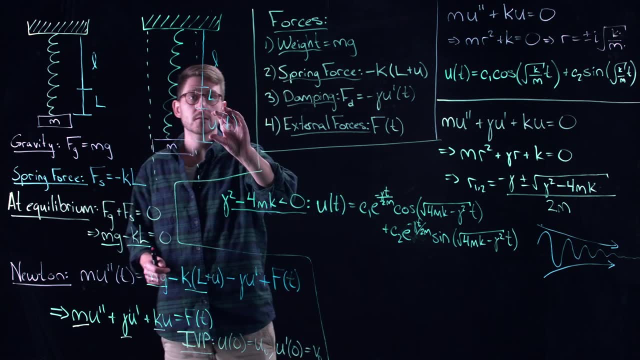 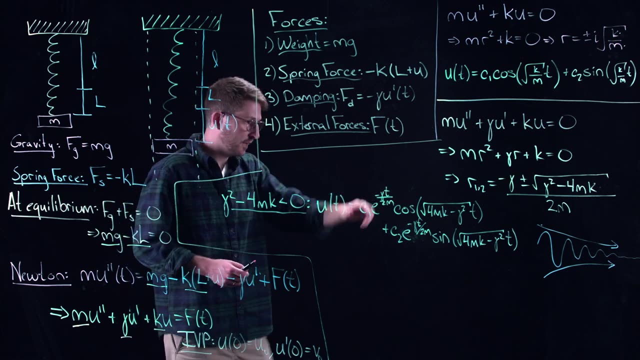 but not as low as it was before, And it's slowly, slowly, slowly wiggling into zero. Remember u, equal to zero represents us being at equilibrium here. So this thing is being pulled down and then sort of wiggling ourselves in. That's what this wiggling right here is, This tiny, tiny little wiggle. 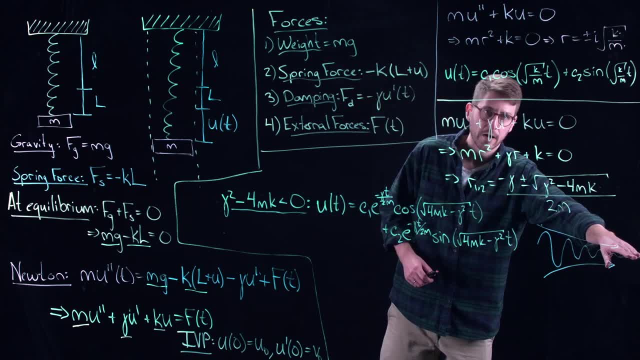 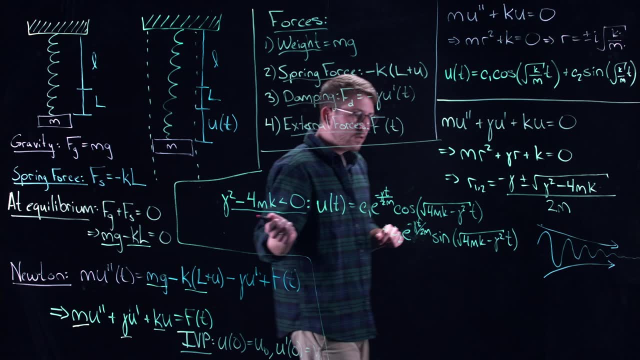 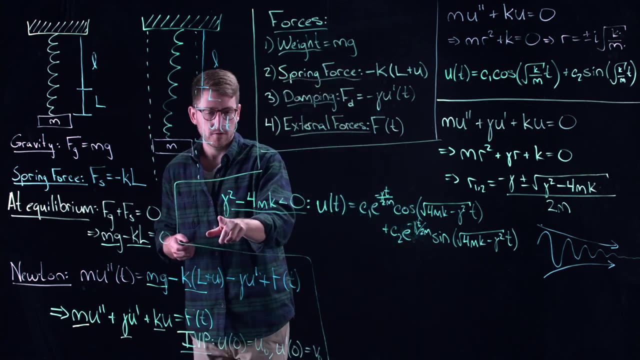 that's left is wiggling into zero. It's sort of a death rattle as you go into equilibrium here. Okay, that's one of three cases. Now you can imagine- let's just imagine here- that we're sort of increasing the damping, right? Well, what's going to happen is if damping gets bigger and bigger. 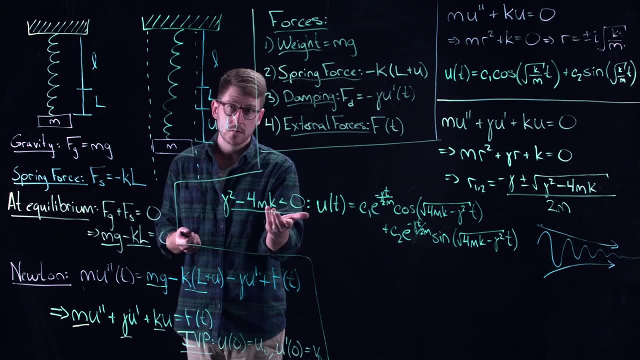 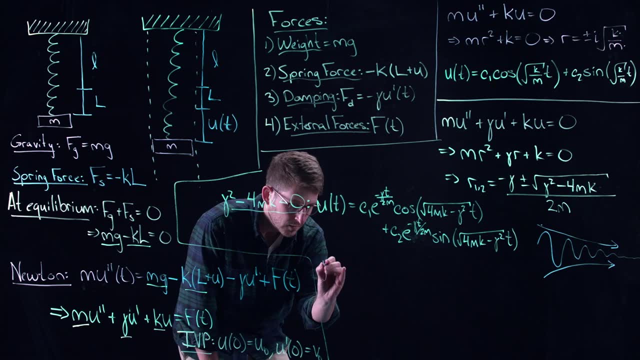 eventually this thing is going to hit zero. This is a continuous function, And so eventually I can make this big enough so that it's equal to 4mk. Let's look at that now. Gamma squared minus 4mk is equal to zero. 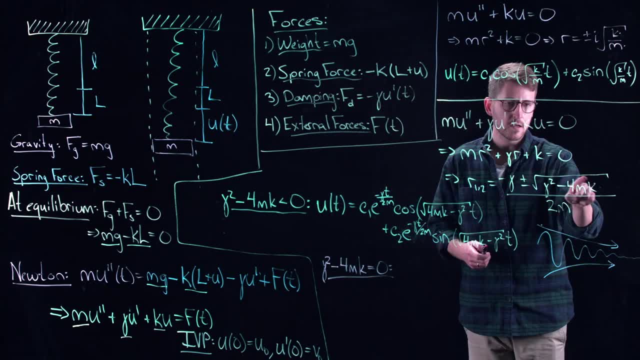 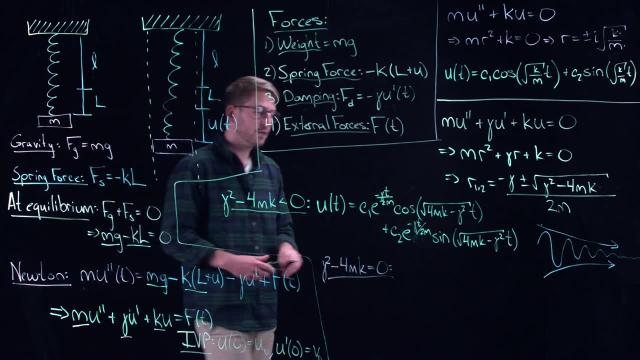 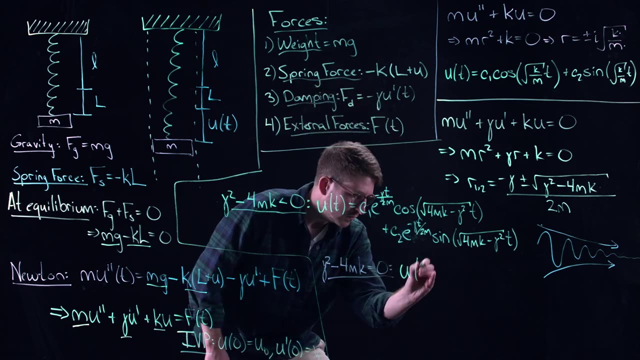 Now I've got a damping, Now I've got a double root, because this whole piece underneath the square root is equal to zero, And so, therefore, what I'm getting is a double root to this characteristic equation which we know very, very well. This leads to: u of t is equal to well, actually. 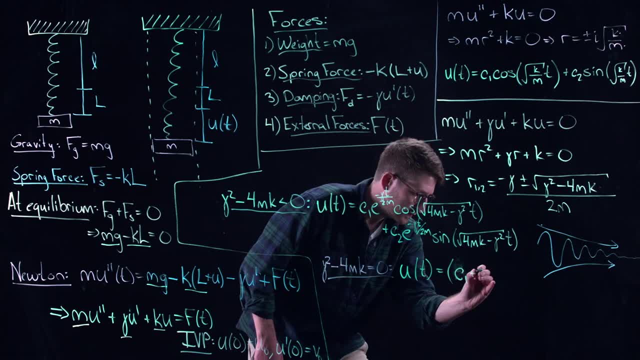 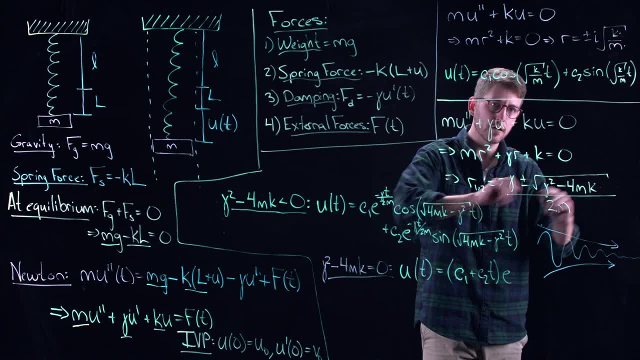 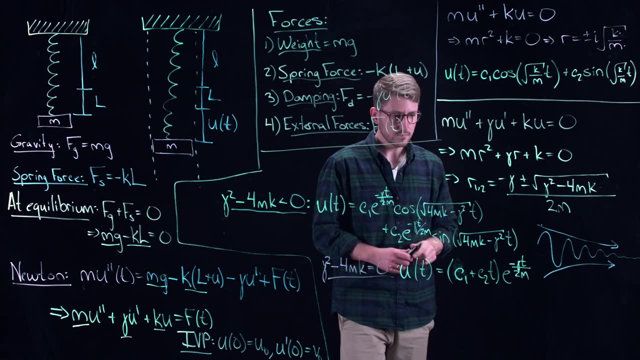 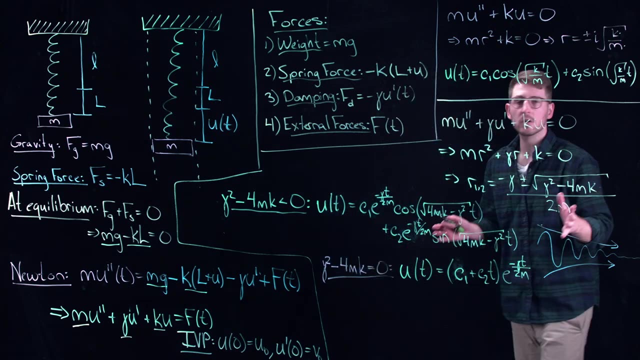 I've got a double root, I've got a double root, I've got a double root And I'm just left with minus gamma over 2m. Remember, this is zero underneath the square root, So minus gamma t over 2m. Now, what is this guy doing? Well, no more oscillations, no more sines and cosines. 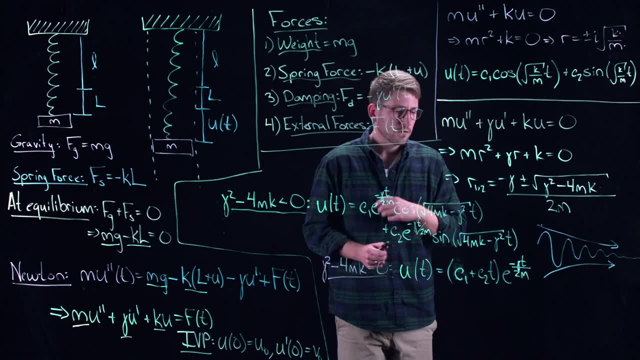 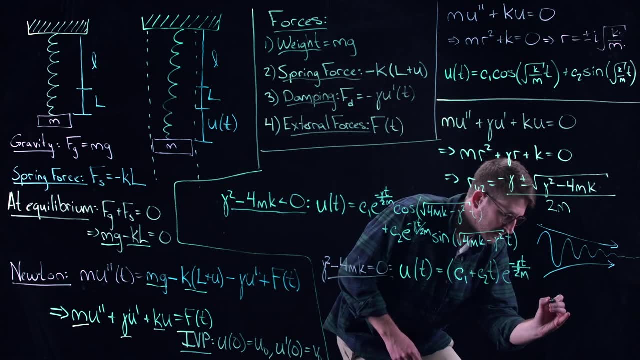 So I'm going straight into zero. right, I might get a little bit of a jump here, But in general, you should expect something that looks like this. So because of this t right here, I get a little bit of growth at the beginning, potentially So. 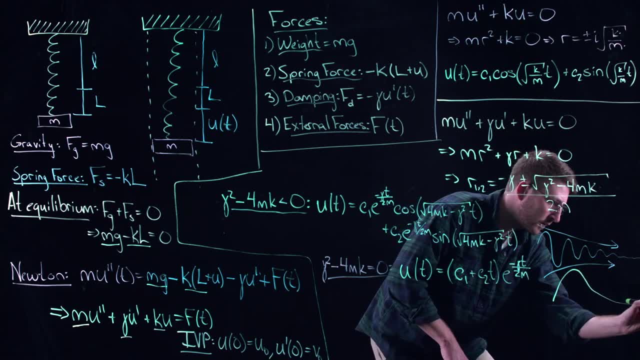 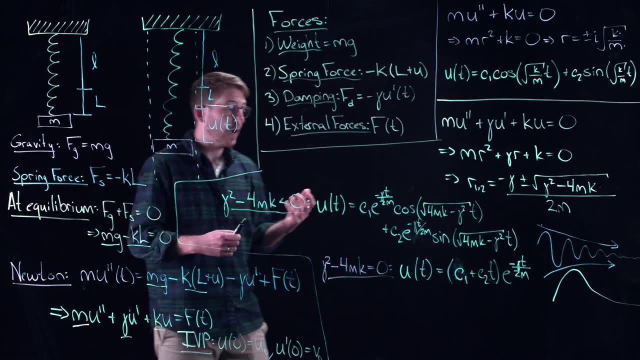 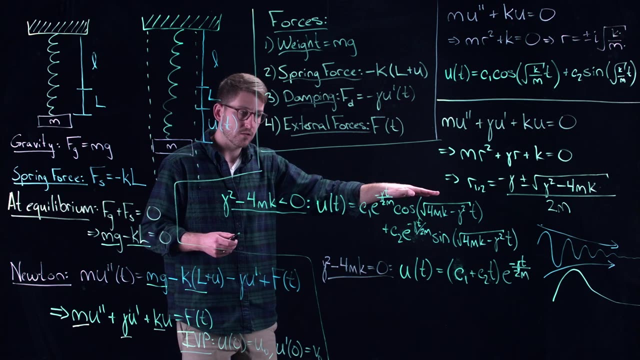 you'll get something that goes up and then goes, like an exponential, right into zero. So what's happening here? This is a case where you have a lot of damping, So I pull down my m. It goes whoa, and then hits right back into the zero case, right? So again I pull it down. 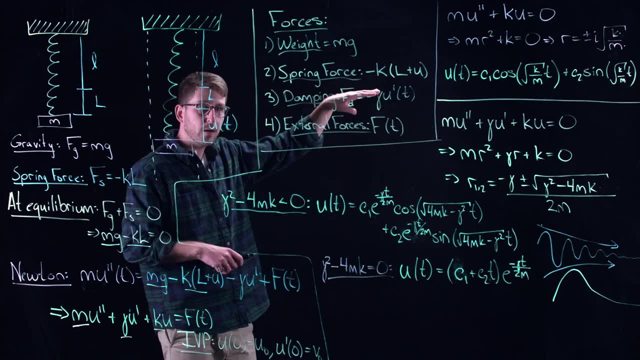 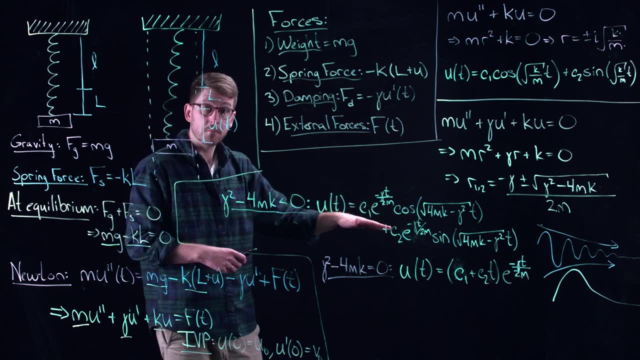 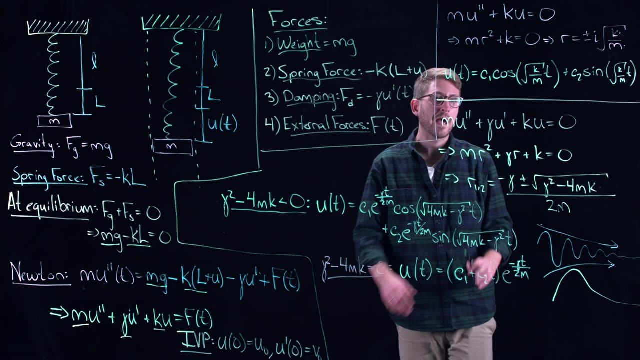 This initial little burp, here is it flying? It just goes right about. Might be starting back up in response to me pulling it down, And then it's slowly settling into its equilibrium point. That's what's happening here, right? And this is a perfect balance between damping and the mass and the spring constant. 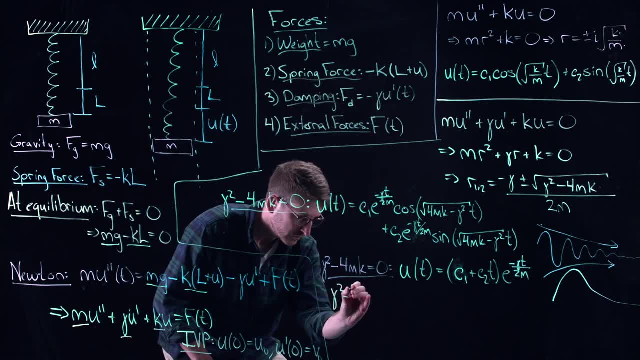 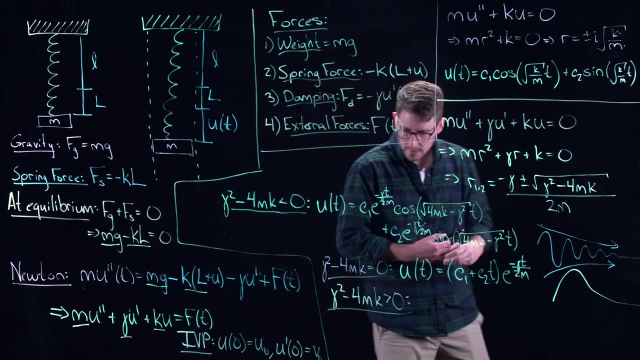 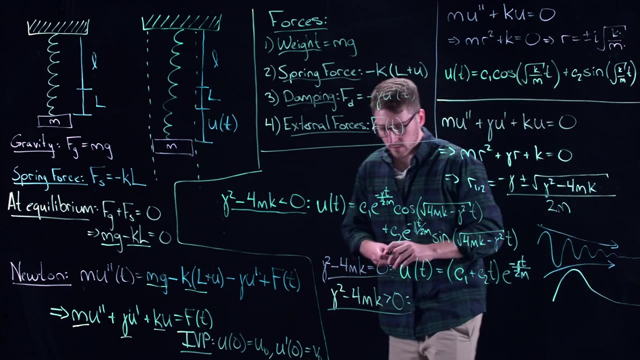 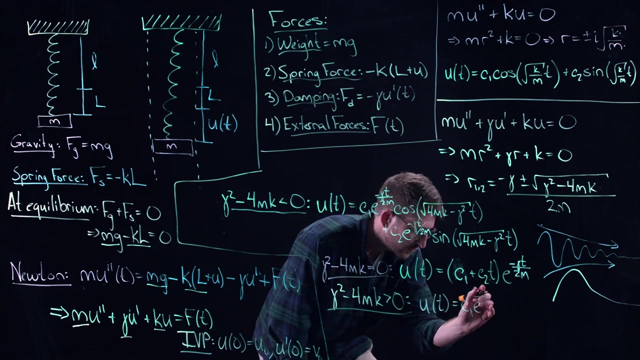 So this is something you probably would not expect to see in reality, But what you would expect to see is, the last case, positive. now, this is positive. you get two real roots to this equation, right, So let me just write them down. The solution is: u of t is equal to c1 e to the. let's do r1 t plus c2 e to the r2. 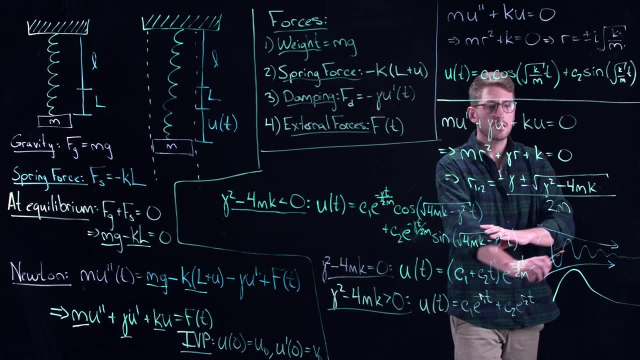 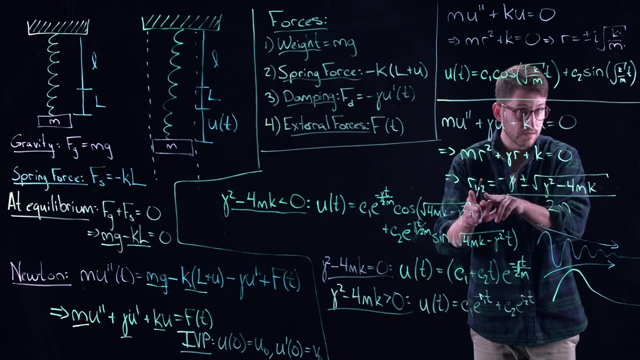 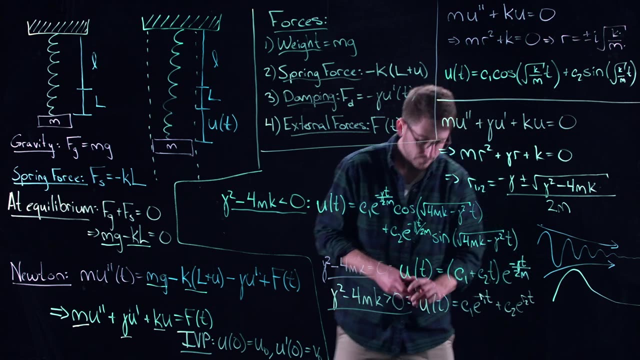 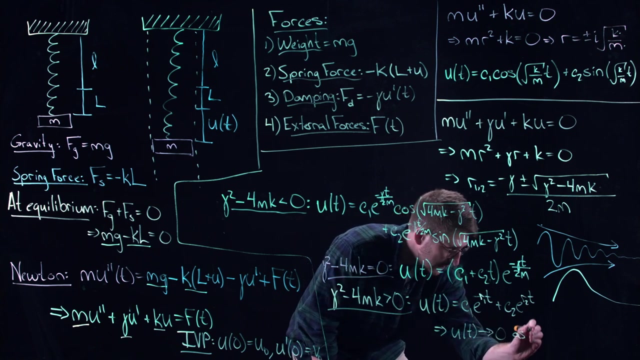 t. Now, in this case, you can actually show that when this thing in here is positive, both of the roots have to be negative. So that means that this part goes to zero and this part goes to zero. So this gives us u of t goes to zero as t goes to infinity, right? So I don't 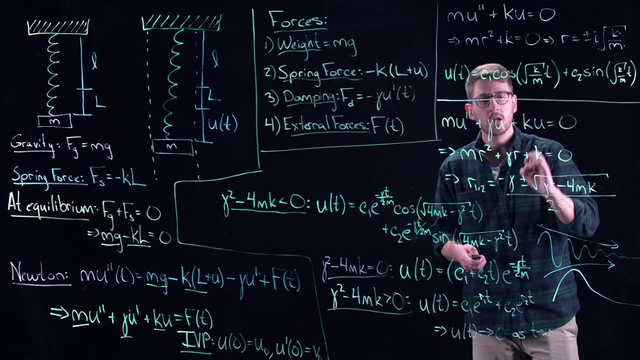 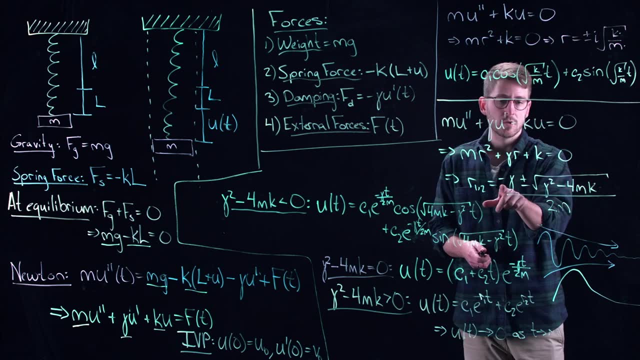 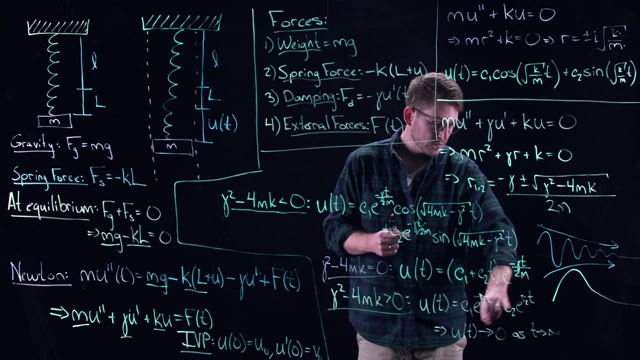 want to go too much into the depth here of why that's the case. Maybe you should pause the video and try and show this with a nice little inequality. You can show that this piece right here is less than gamma, which means that the top is less than zero in the plus case. But that tells you that you have two negative roots. 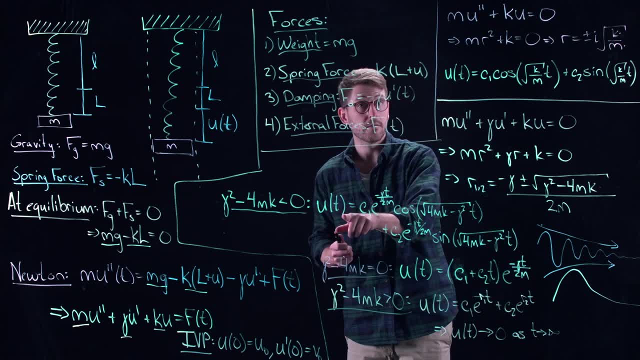 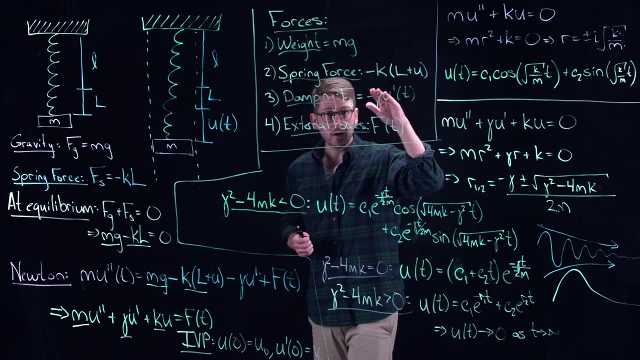 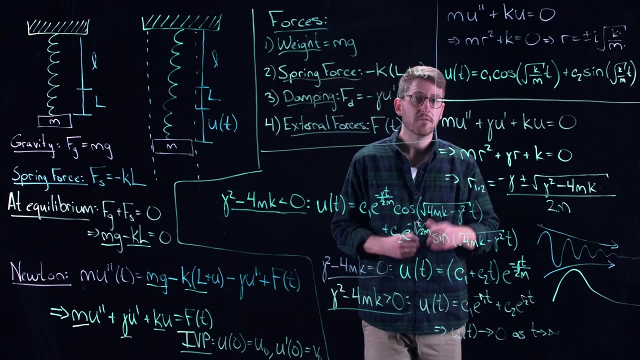 That tells you that u is going to zero. All three cases gave us that u is going to zero as t goes to infinity. So what do we see here? Damping causes us to sort of die out, to peter out, But the amount of damping causes very different ways that we do this. If damping is very, very 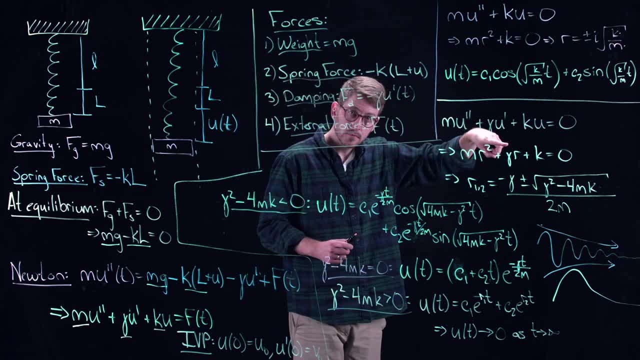 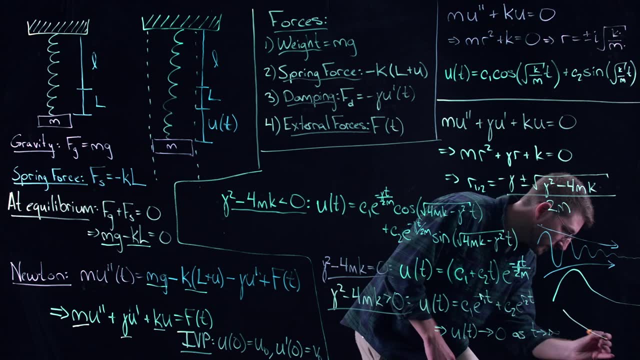 small, I get to wiggle, I weigh in, Whereas if damping gets bigger, I go straight in right. So now these are just exponential decays, That's it. There's no, there's not even a burp. There's no wiggles, It's just. 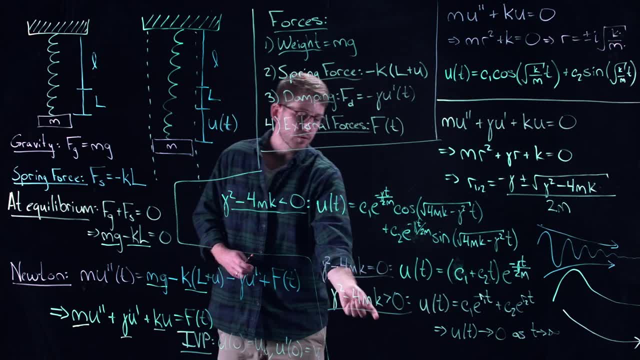 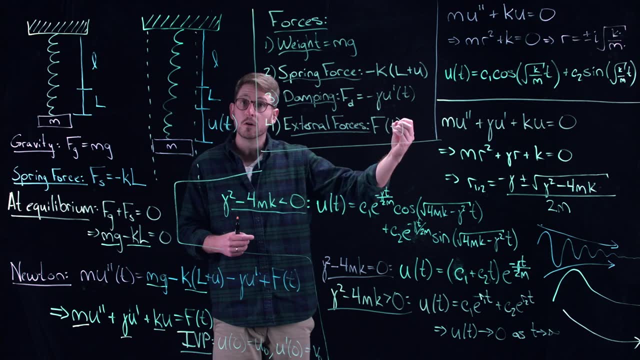 straight in. Think about this last case. Where would I encounter this? Take my bucket of honey. Do the experiment in the bucket of honey. Now you can close your eyes. You can imagine this. Pull the weight down and let it go. What's going to happen? 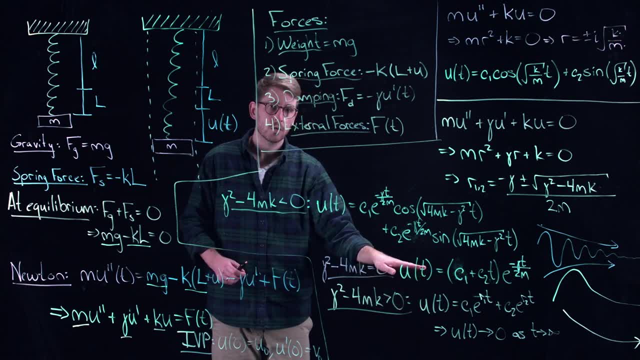 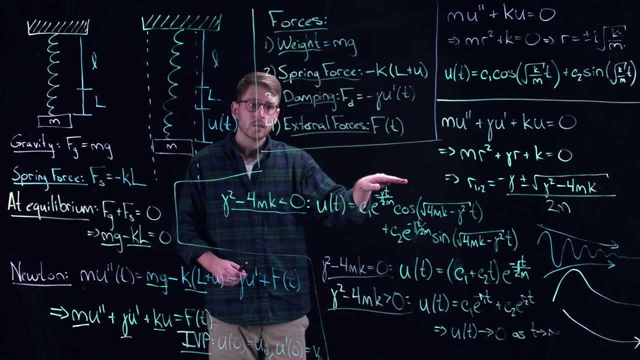 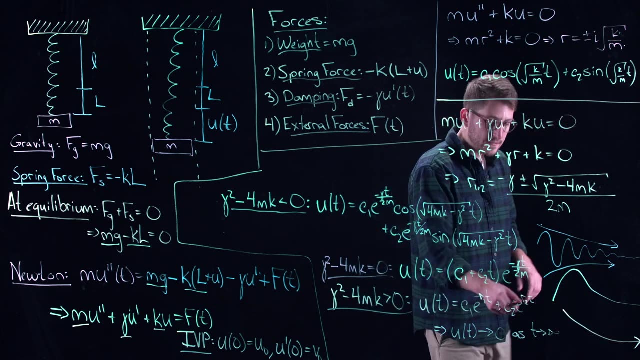 So, so slow. right, It's coming so slow It's just going to fall into the equilibrium. It's not going to go over the equilibrium, It's just going to go in and settle down. That's what you're seeing here. You just get a monotonic decay. 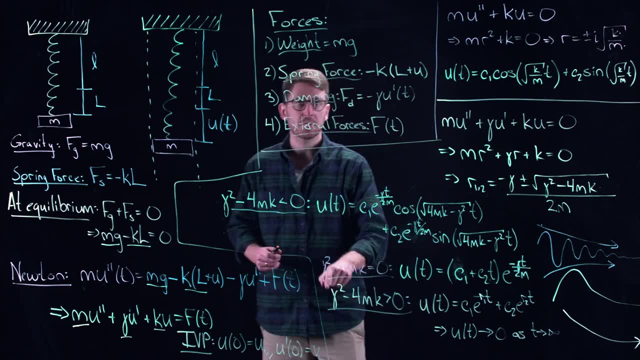 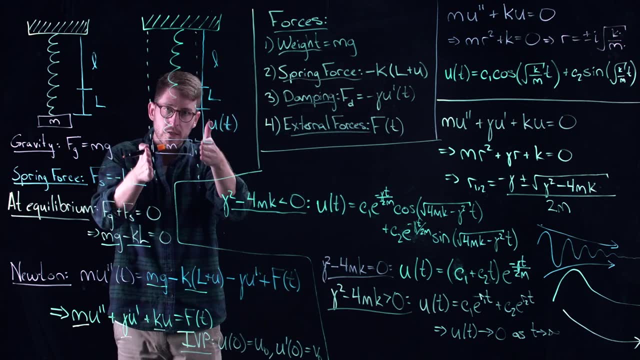 into zero, And that's because you are so damp. There's so much resistance acting on this thing. Same thing. If you put up guardrails on the side of this and they really, really squeeze in, So you have tons and tons of damping, You're going to fall into the equilibrium. It's just going to. 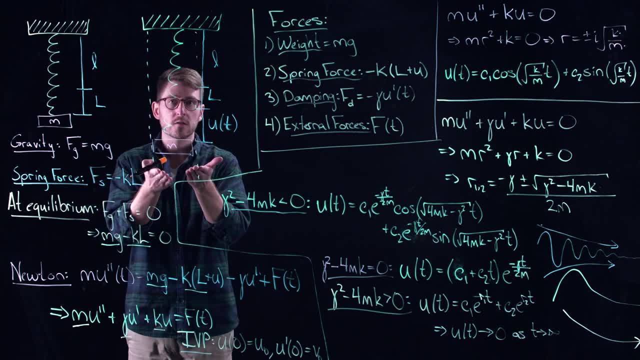 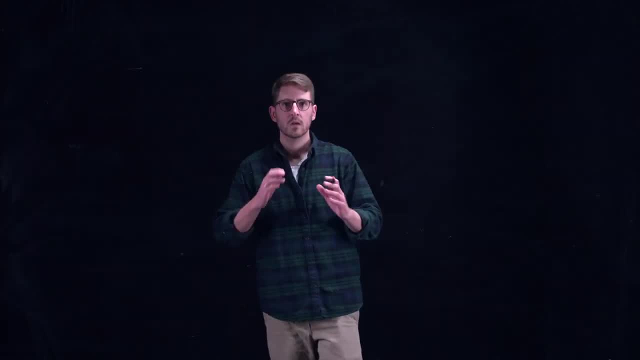 be tons and tons of friction that's being generated here. Well then, this thing is just going to really, really, really, really slowly just die off and go into zero. Okay, So now let's look at what happens when we start putting external forcing on these things. 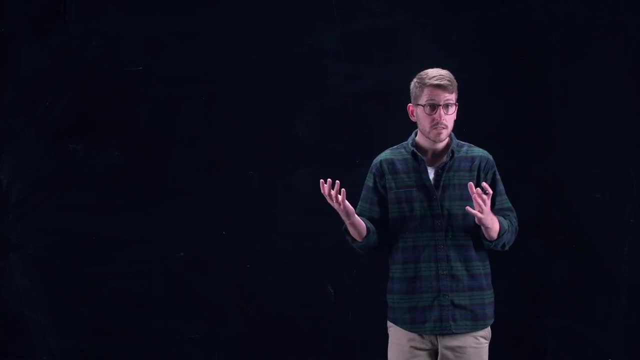 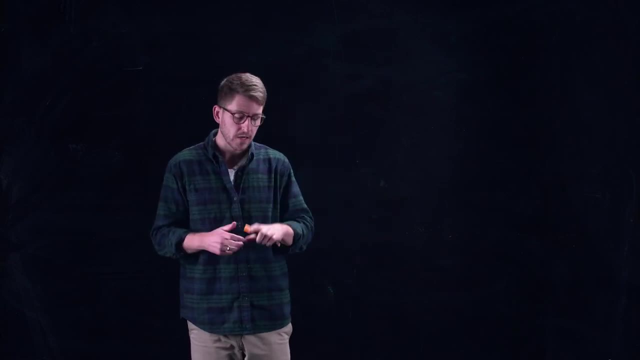 Now, unfortunately, understanding all external forces is just too difficult of a task. You have to use variation of parameters to solve that. So we're going to restrict ourselves to a very specific scenario, And this is a very common one that you would find in engineering and 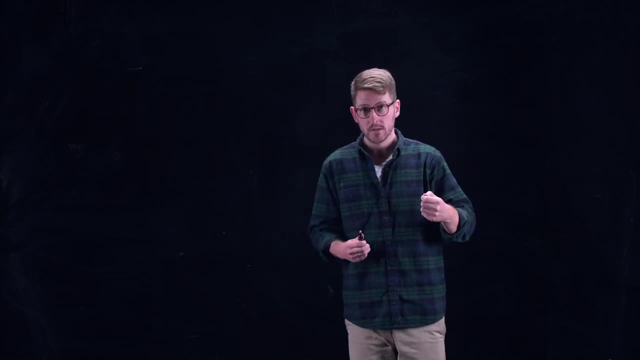 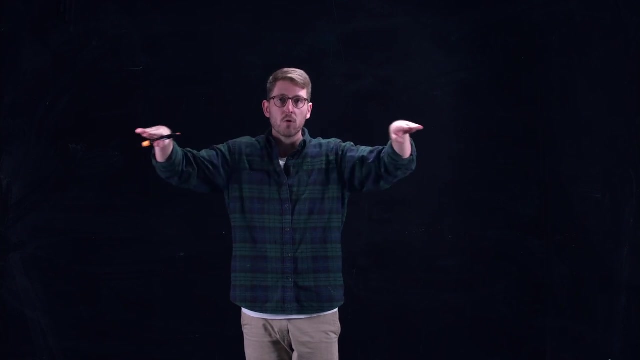 physical applications And that is a periodic forcing. So, for example, you can imagine that maybe, if this is, if your spring mass system is sort of bolted into maybe a board or a rod, you can imagine that there's something sort of lifting and shaking this board or rod. 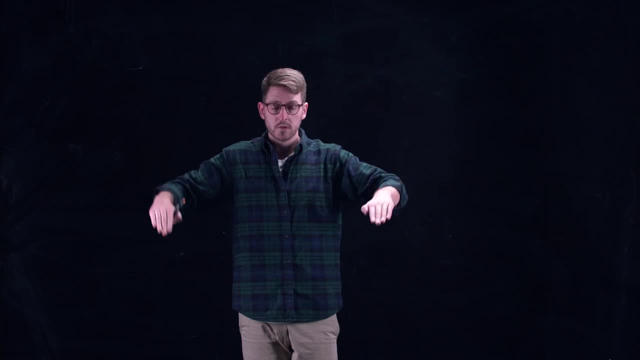 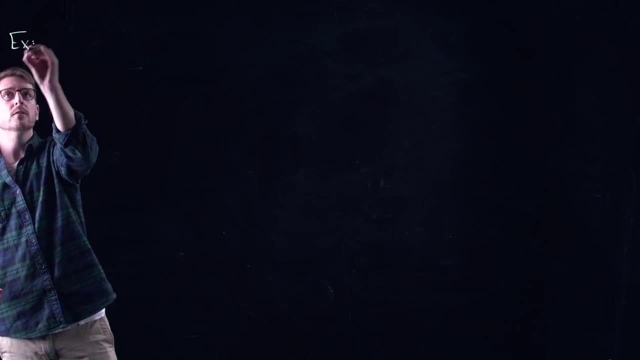 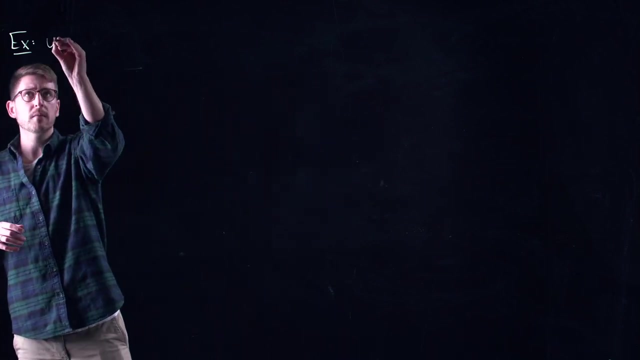 at a periodic interval. Okay, So let's take a look at this, Let's do this sort of by example, And again, I don't want to have to use M gamma and delta every, or M gamma and K every single time. I'm just going to use real numbers here. 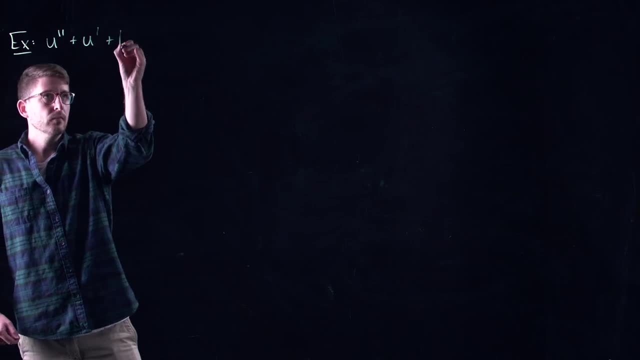 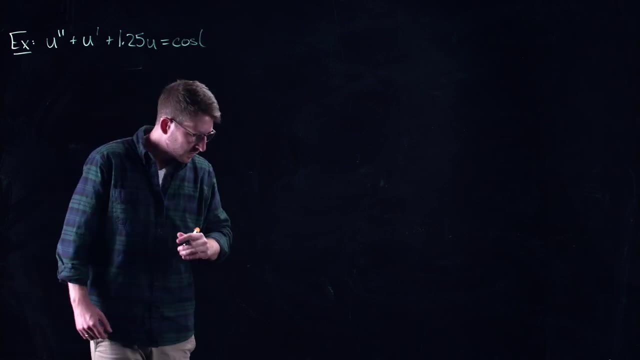 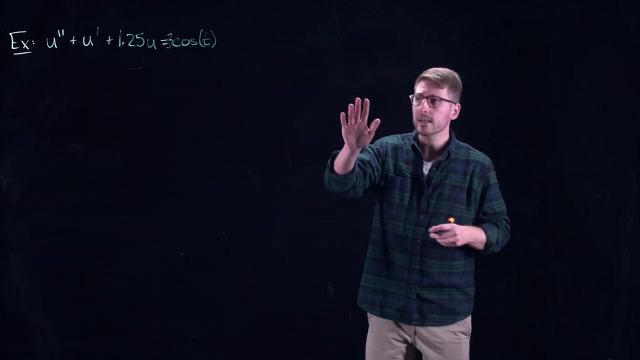 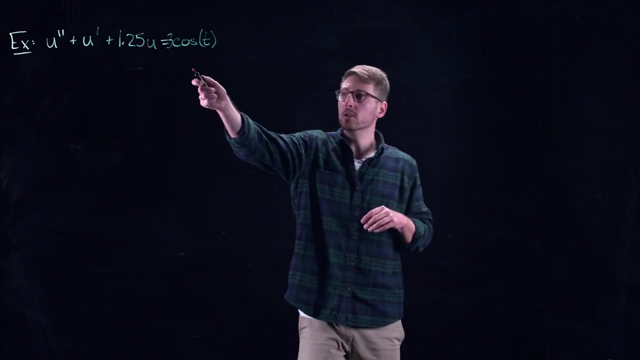 make my life a little easier. So let's do, let's do three cos T, Okay, So this is a perfectly accessible problem to you, having watched the videos leading up to this right. This is a linear constant coefficient equation. The external: 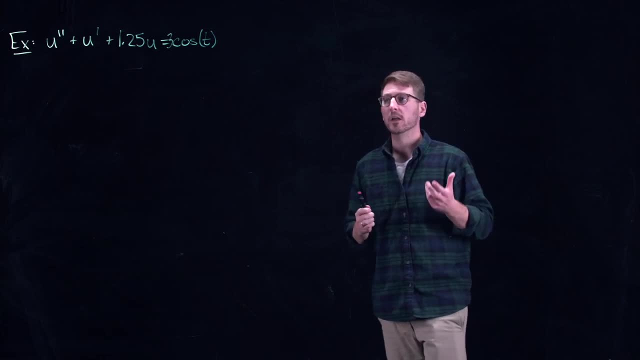 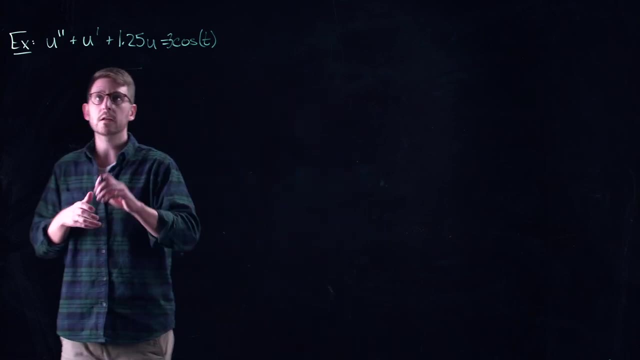 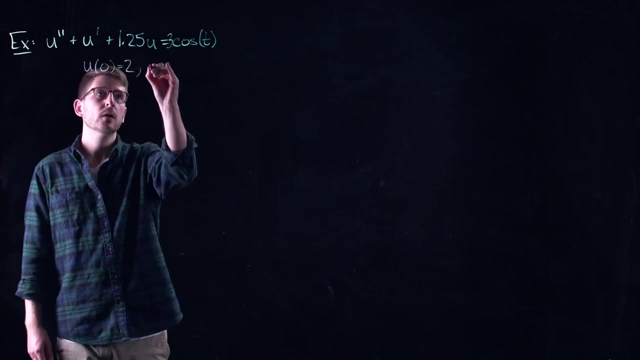 forcing here can be handled as we described in the video on non-homogeneous equations and solutions to those equations. We can even include some boundary condition or some initial conditions here. Let's do U of two. U of zero is equal to two, U prime of zero is equal to three. These 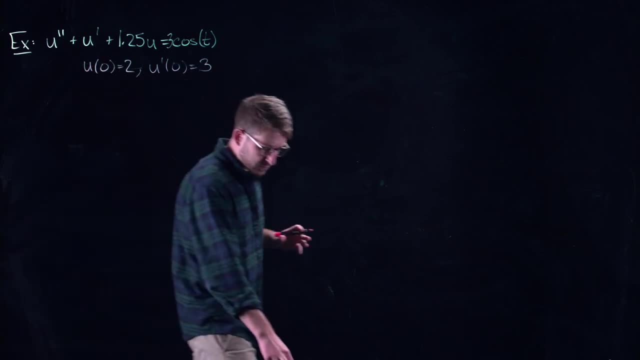 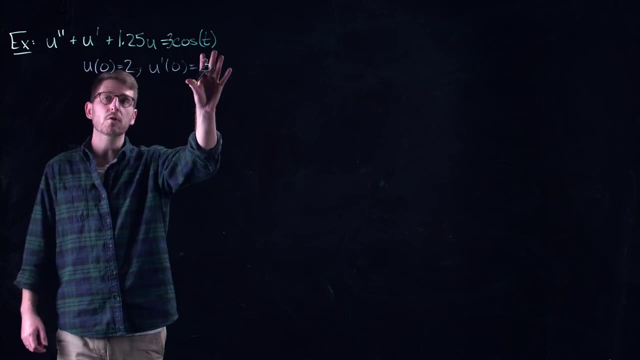 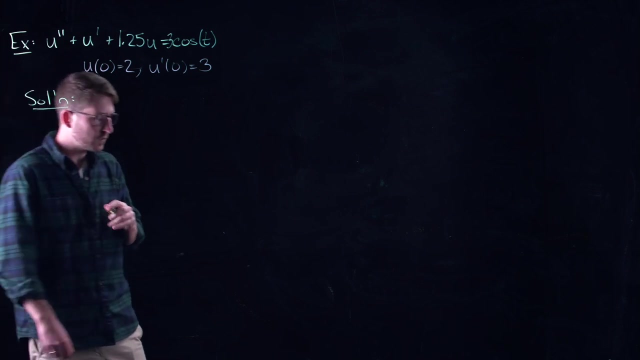 are somewhat arbitrary, mostly just for exposition. Okay, And here's what I want to do. Well, we know we can sort of go through all of the methods here and we can get the solution to this thing, So I'm going to skip all of the fun. I'm going to leave this for you as an exercise, but this gives me. 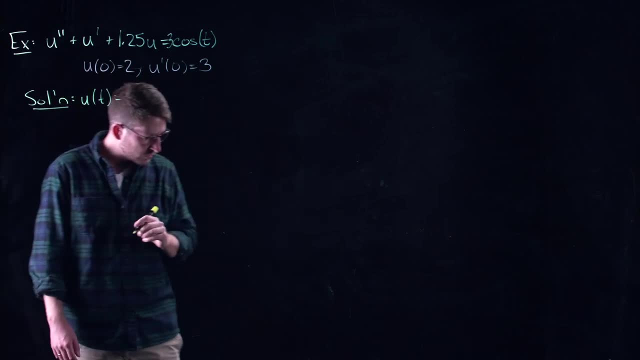 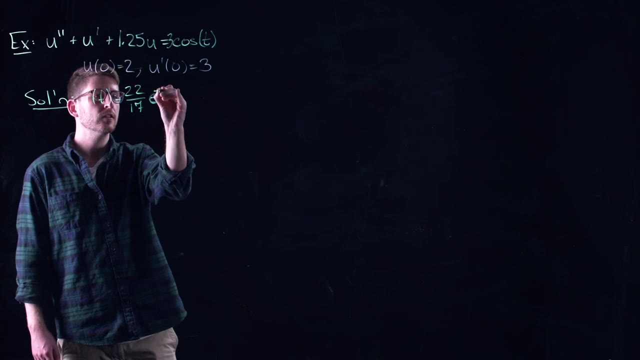 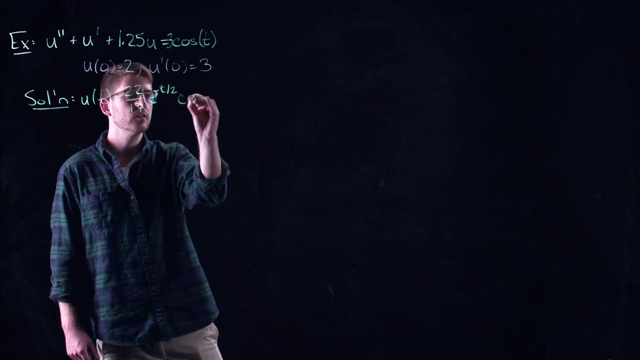 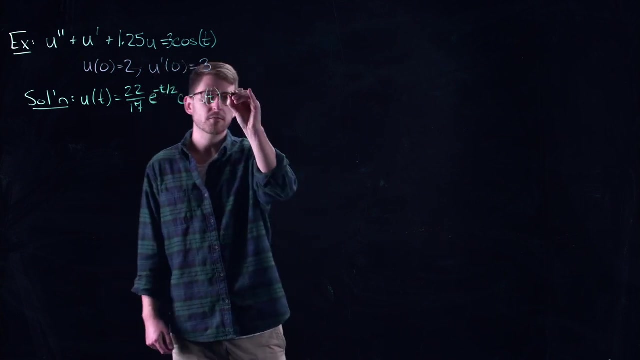 let's take a look: U of T is equal to okay, I got 22 over 17 E to the minus T. and then, sorry, T over two, pardon me, cos, And inside of the cos is just a T term. And now plus 14 over 17 E to the minus T over two. 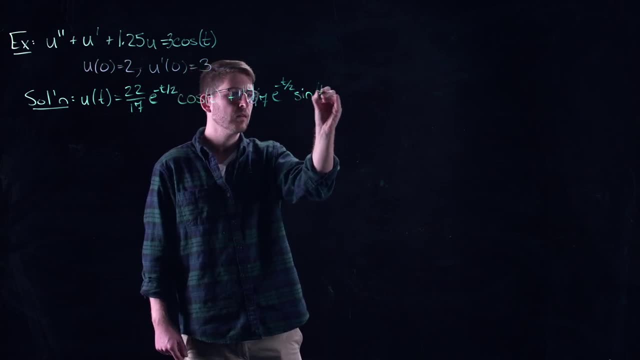 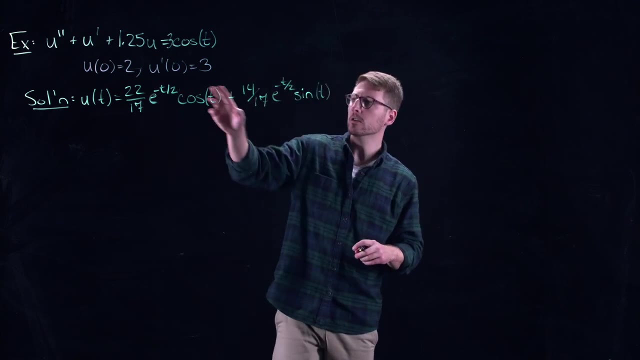 sine of T And then plus. so this is the homogeneous solution. The C1s and C2s have already been found using my initial conditions. That's why I gave them. And then let's put the specific part in, So I get plus. 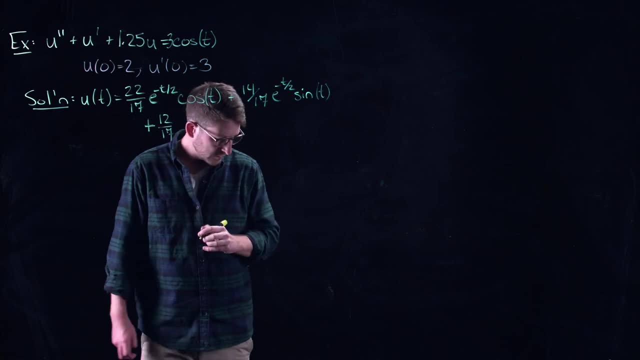 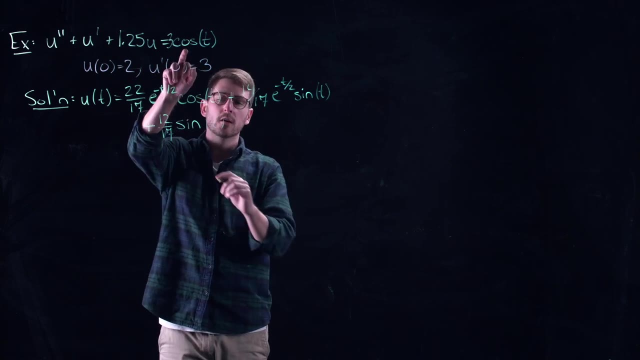 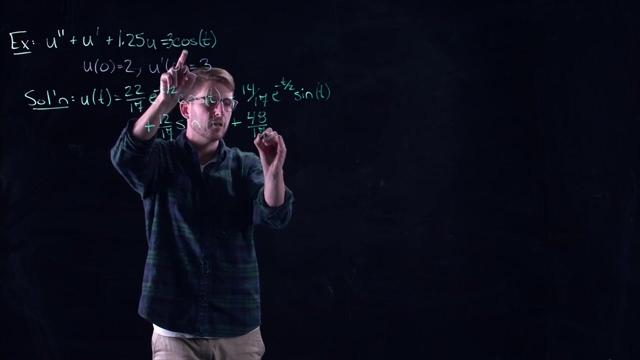 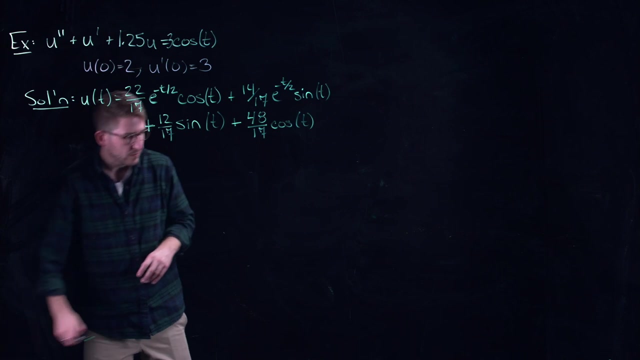 12 over 17.. And this is going to be sine of T. Remember, the specific part is going to be a constant times sine plus a constant times cos. Identifying those constants is the name of the game. So I got 48 over 17, cosine of T. Okay, Now let's take a look at this. Let's sort of examine this out for a 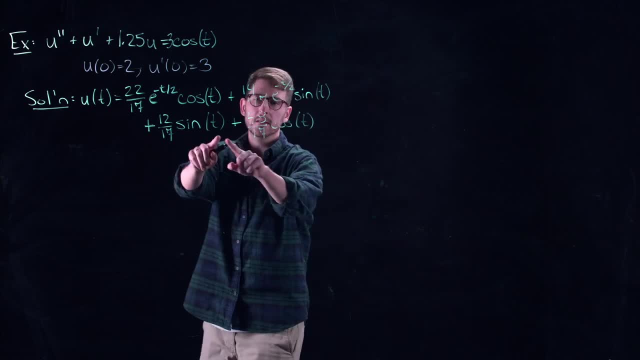 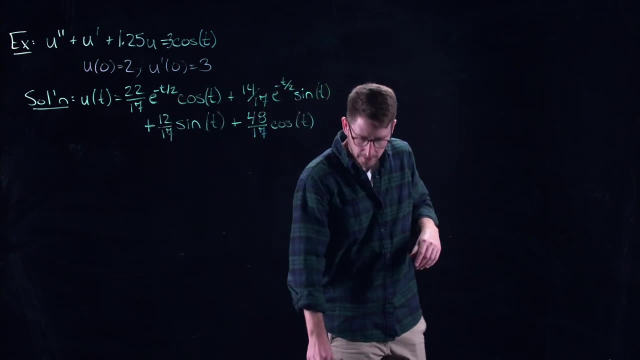 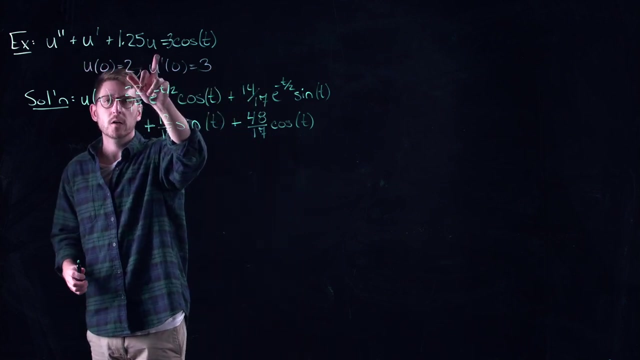 moment. What's happening here? Okay, So remember, this is the specific part. It is due particularly to this external forcing, this periodic forcing that's being applied here. This is the homogeneous part. The homogeneous equation is a damped vibration equation. right, It's damped because there's a gamma in here. 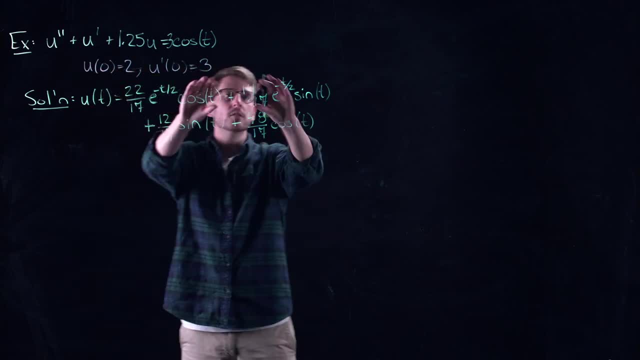 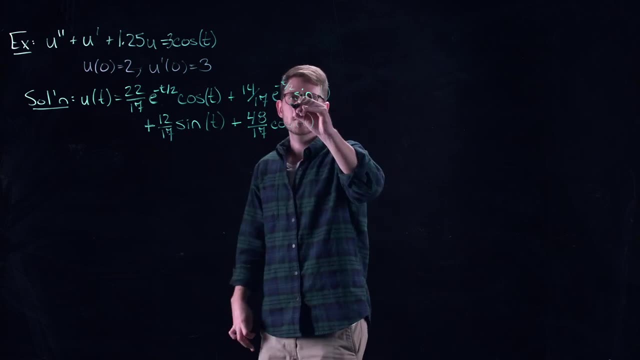 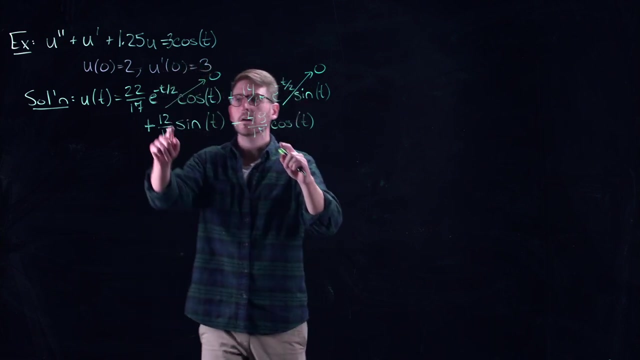 There's gamma equal to one, Then you can see, just like we covered in the damped part, these damped oscillations from the homogeneous part are dying out. So let me just write it like this: Going to zero, going to zero. Now I'm taking time to infinity here. That's because of the 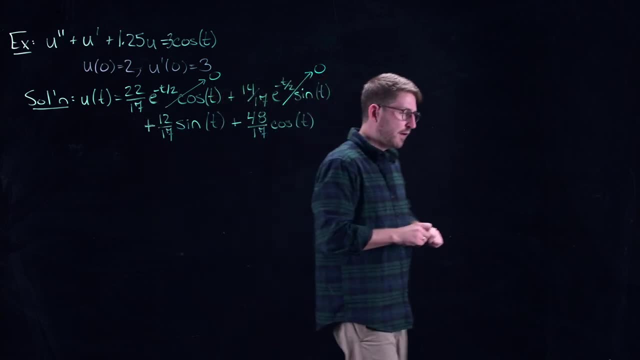 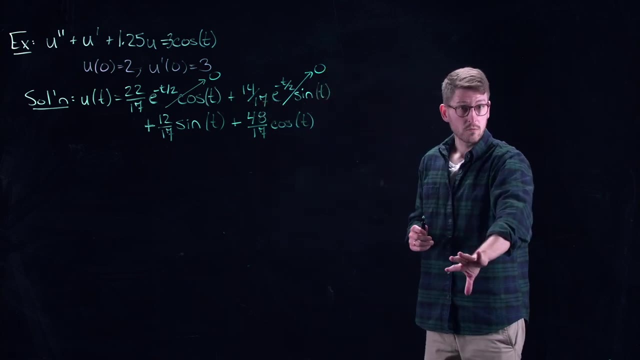 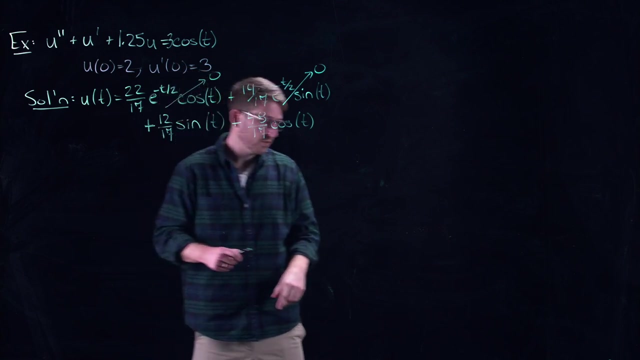 exponential terms. So what happens after a while? These homogeneous parts, these damped oscillations, they die out, just like they were doing with the last piece down here. What are we left with? Constant periodic motion? And what is the period of that periodic motion? It's exactly the. 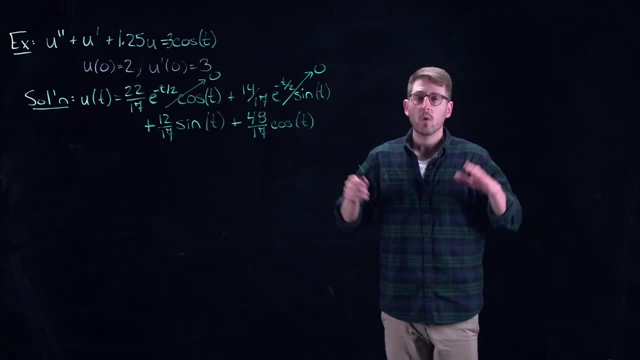 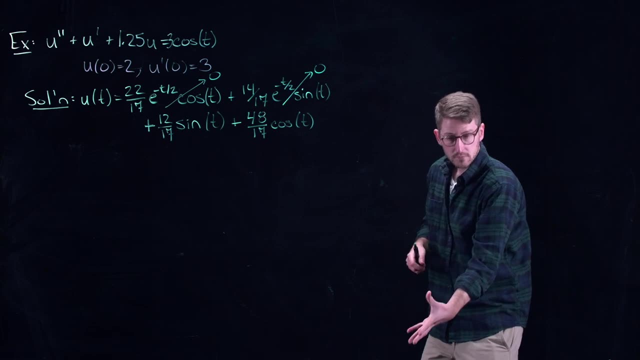 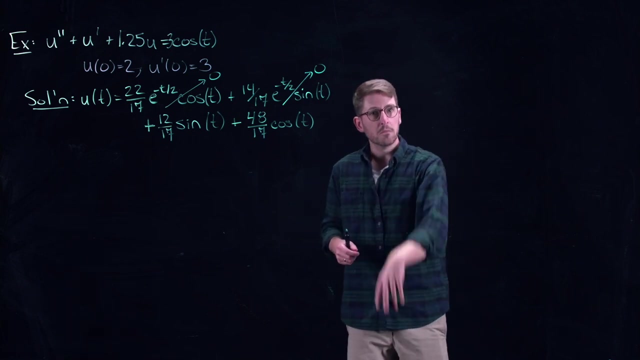 same as the period of the forcing here. So what's happening? I'm shaking this board up and down, Then I take the weight or the mass and I pull it down. I let it fling up and do its thing. Well, initially, from me flinging it, there's a little bit of a transient with this damped. 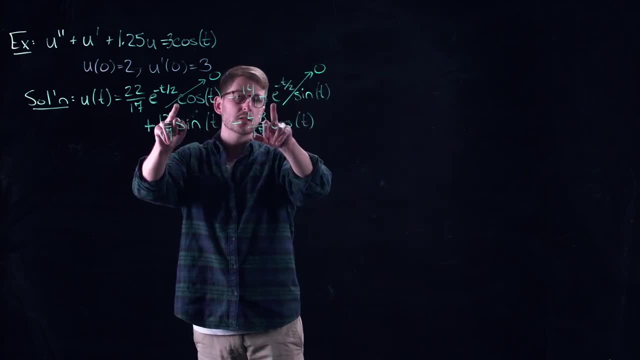 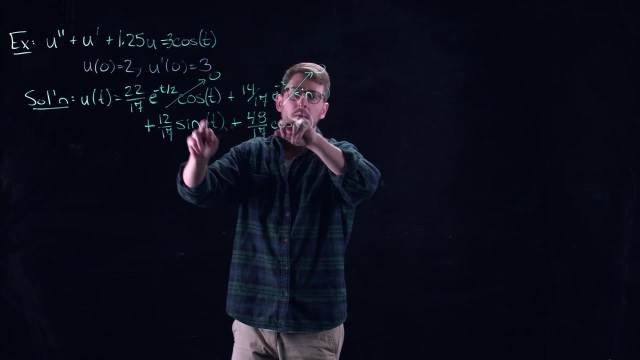 oscillation, but eventually the wind resistance kicks in, or the air resistance, the water resistance, whatever it is, the friction kicks in and it kills that oscillation, But you're still shaking this thing. So eventually, what this does is it synchronizes up with the 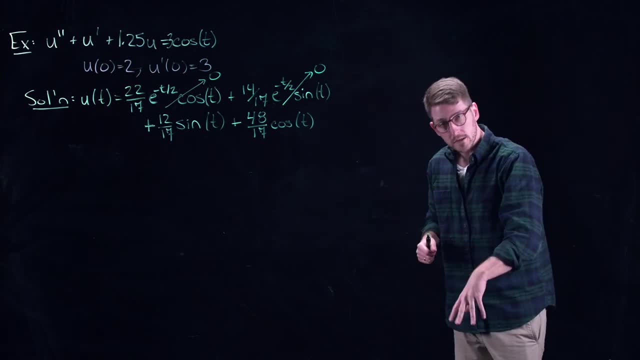 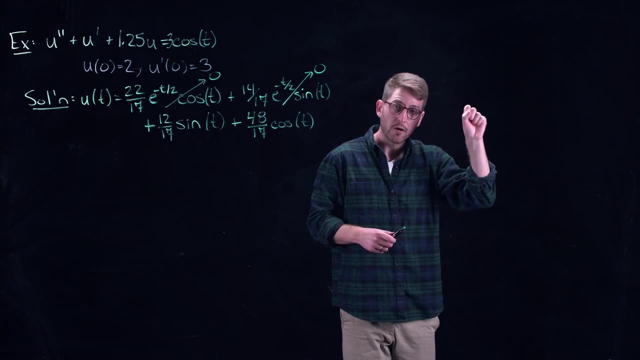 shaking that's going on up here. So this is sort of like a yo-yo, right? That's exactly what's happening. The periodicity that I am throwing my yo-yo at the ground, the yo-yo is going up and 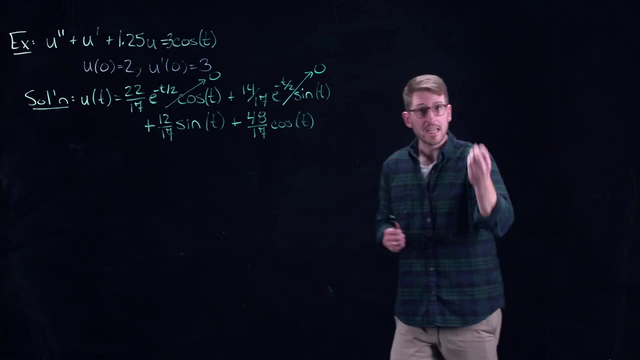 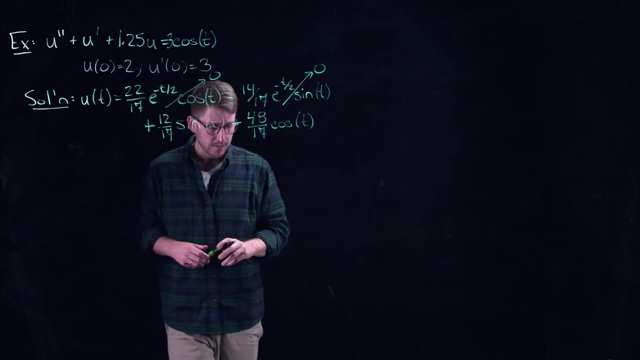 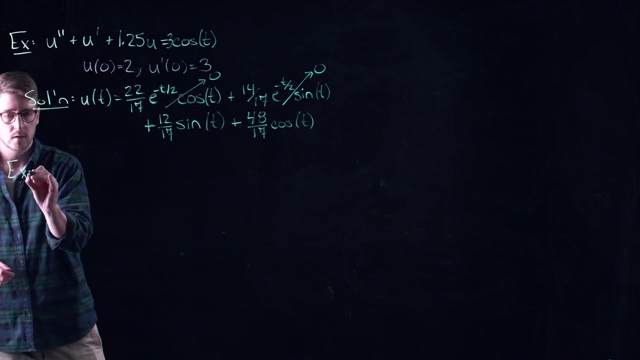 down with that same periodic motion. That's the same thing that's happening with my mass and my air. Okay, let's see another example. Let's see what happens if I do this in a vacuum, So I don't put any damping on this. Let's do u double prime plus u is equal to. let's say cos I'm going to. 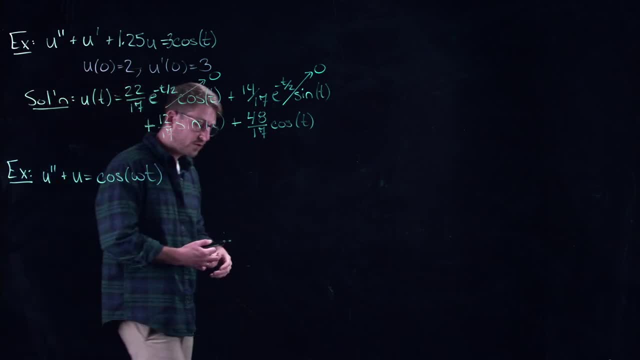 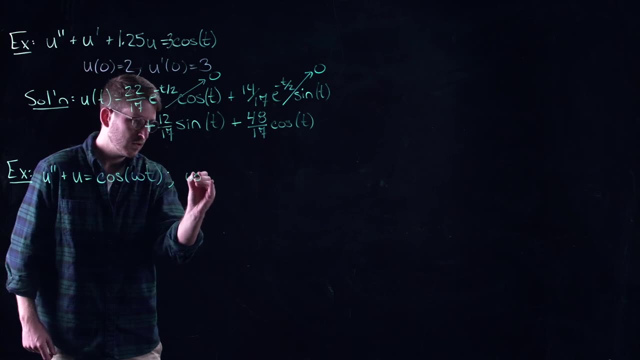 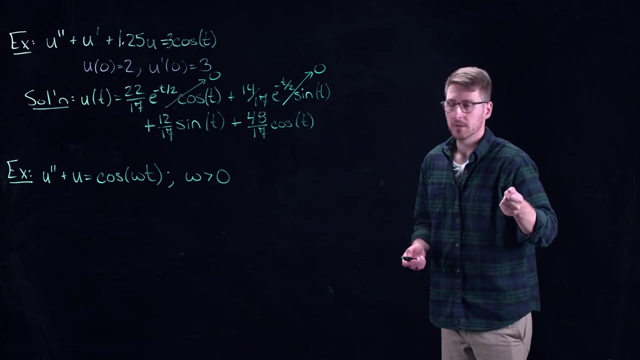 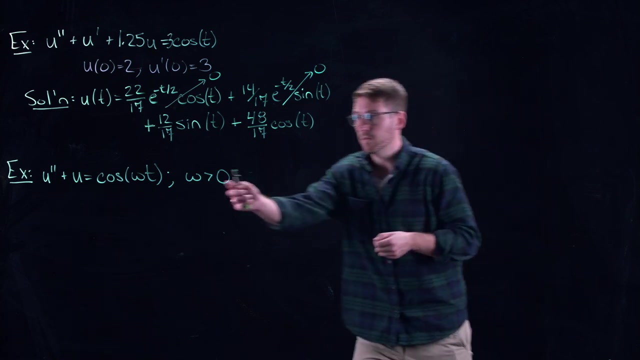 use omega. This is the sort of standard parameter that people use for the frequency. So in this case, omega is a positive number. Basically, you can imagine that I've got a dial on my system here and I can choose what the frequency I'm going to force this thing with. Okay, that's what my omega 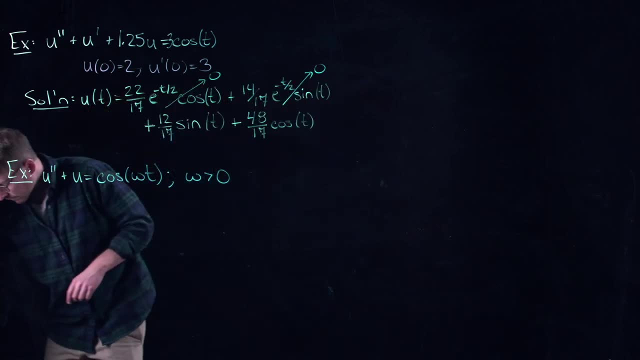 is Okay. well, let's take a look at something right away. So first, if omega does not equal to one, well, if omega is not equal to one, then we don't have any problems with that. So we're going. 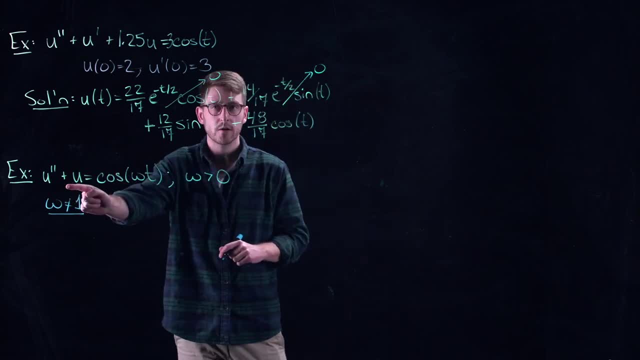 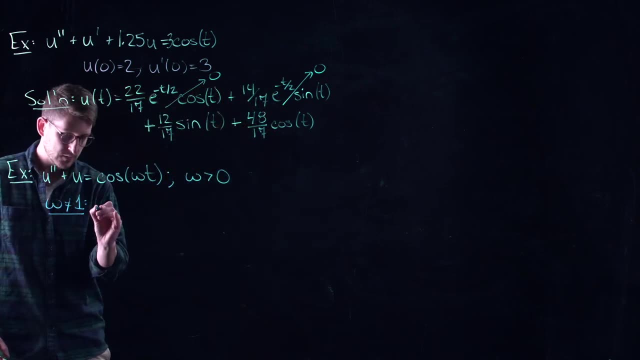 to start with the homogeneous equation right, Because the solutions to the homogeneous equation are cos and sine, And so this gives me solutions that look like this. Now I'm going to write this in the following way: So I actually get u of t is equal to, now I get c1,. 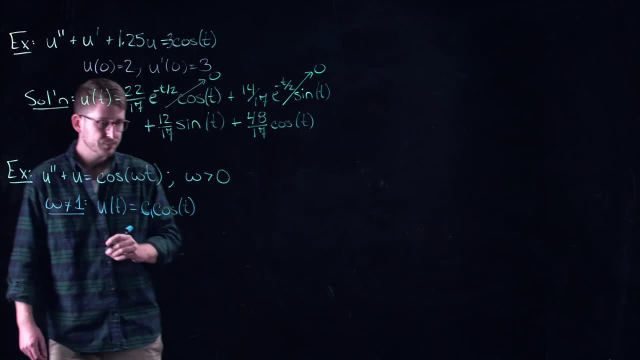 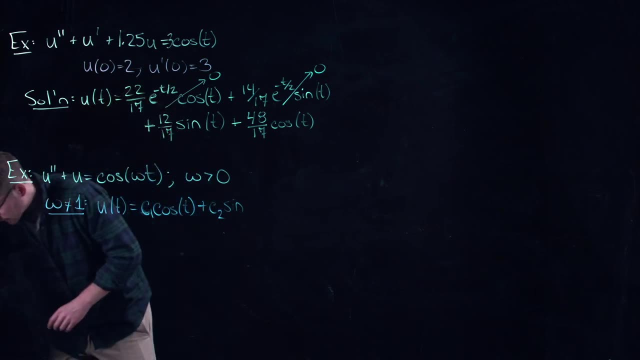 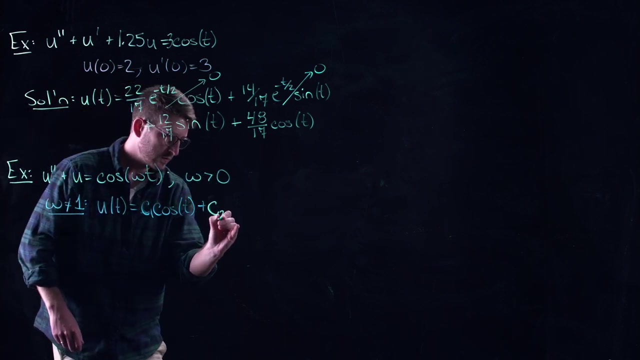 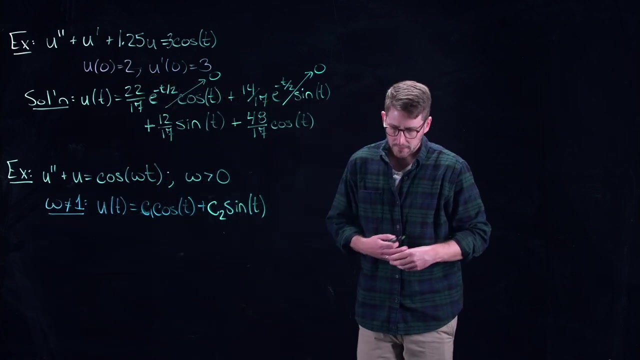 cos of t and then plus c2 sine of t. Sorry, the marker is not cooperating here, So let's do this, Let's go back to green- plus c2 sine of t, And then I have this specific part. you can very easily check that, in fact. 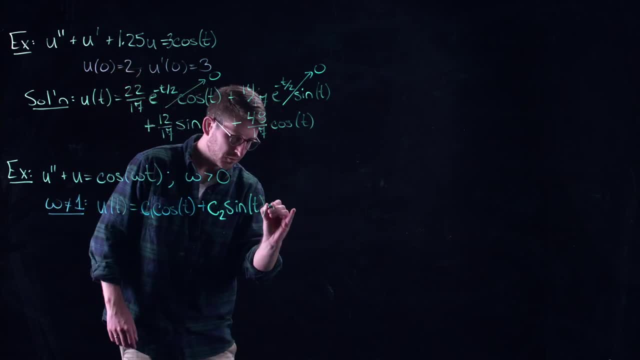 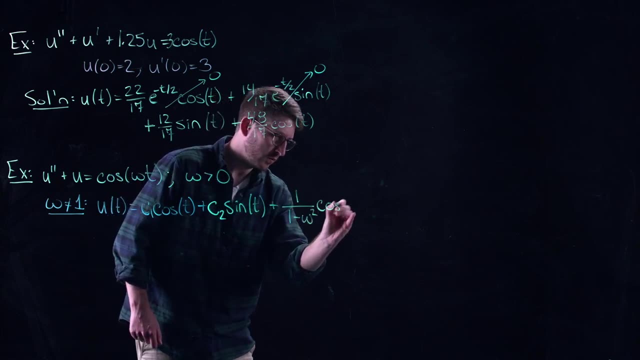 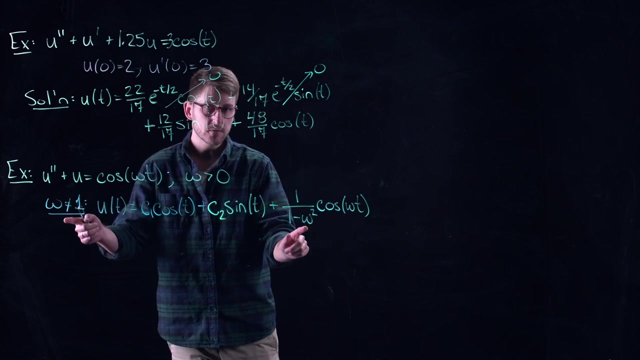 only the cosine comes through, And it comes through in the following way: One over one minus omega squared cos of omega t. Now you can see where the condition omega not equal to one in here comes from, because then I can make sure that I'm not dividing by zero. And so what's? 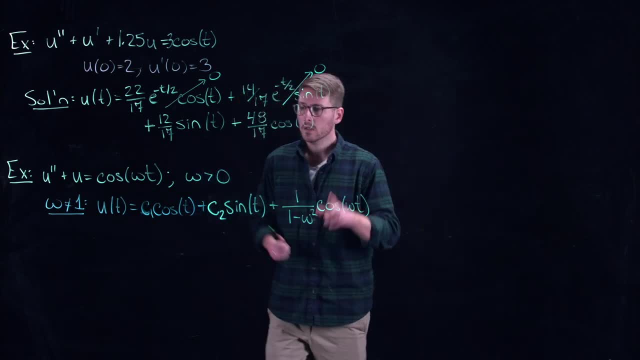 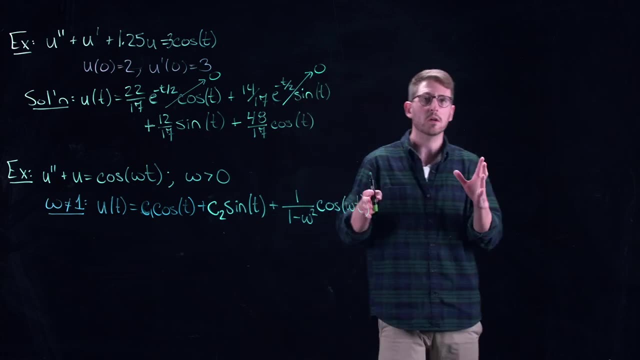 going on with this thing. Well, let's take an x position, okay. So what I want to do is I want to pick something that's not equal to one, So I'm going to pick this thing and I'm going to pick specific values of c1 and c2 so that you can see what's going on. okay, Now, this is actually. 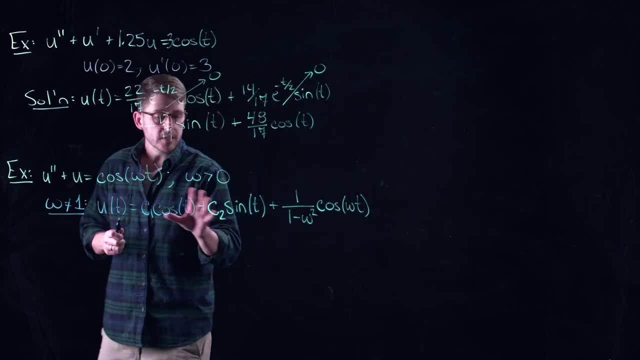 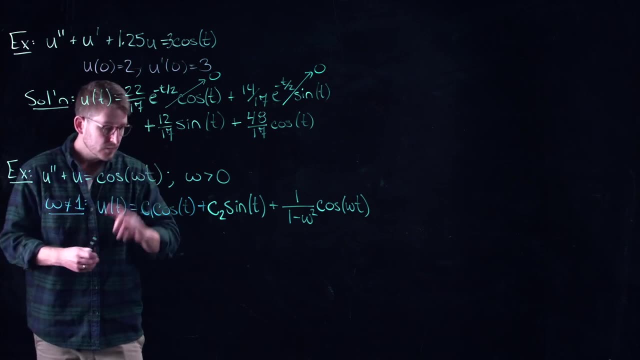 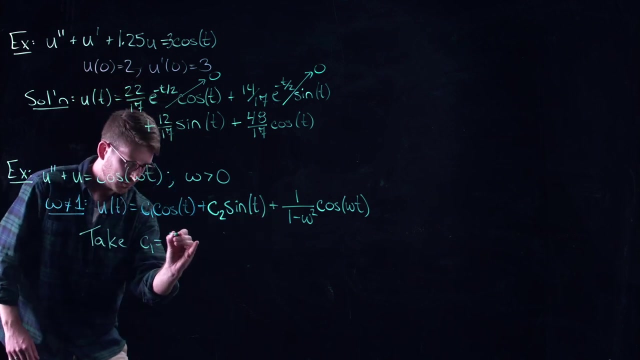 going to hold more generally for any values of c1 and c2, but this is at least going to allow you to sort of understanding what is happening here. for omega not equal to one, So let's take c1 is equal to the negative of this thing. So minus one over one, minus omega, squared. 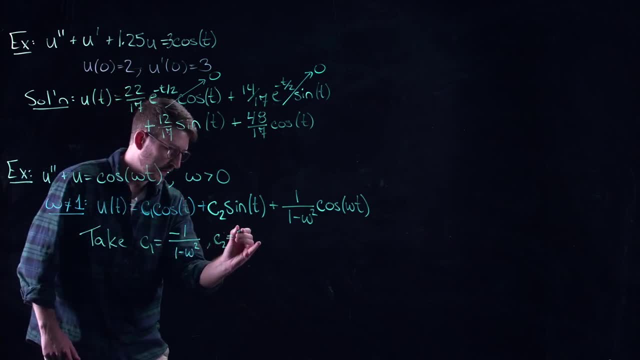 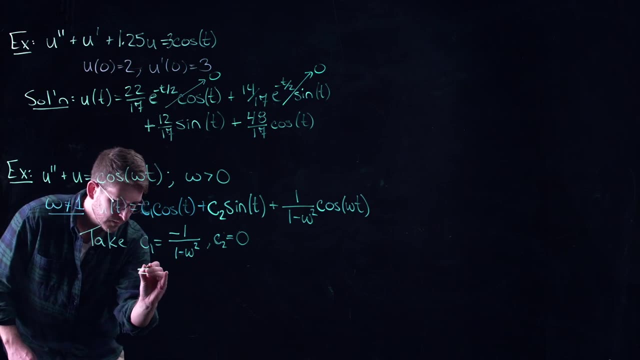 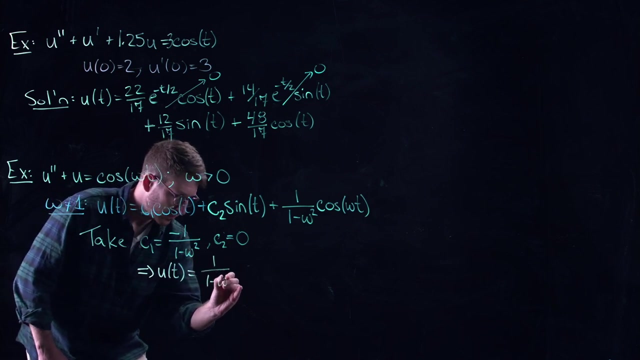 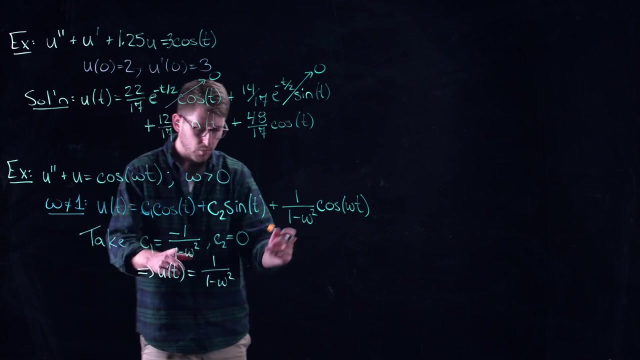 And let's take c2 equal to zero. Okay, so in this case then, u of t becomes one over one minus omega squared. I can factor that out because that's coming from the c1 now and it's coming from the specific part. That's why I wanted to choose those in. 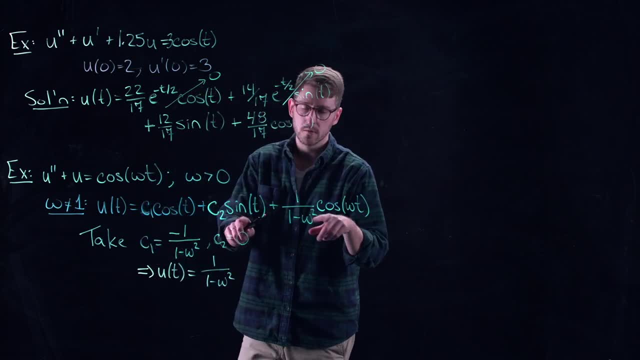 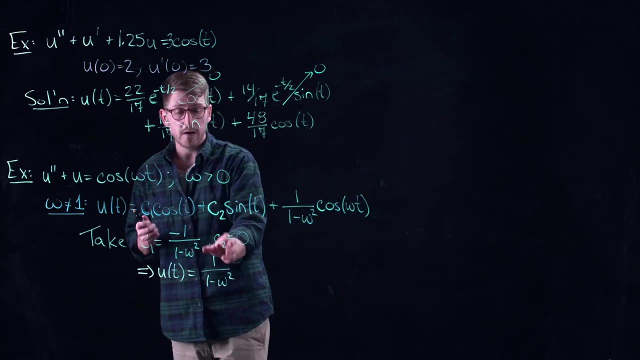 that way. I also wanted to just choose two cos's. I didn't want to have a sine mixed in there. Now we know sines and cosines are just the same functions, right? So that's what I mean about: different values of c1 and c2 are going to give the same basic results here. But I just 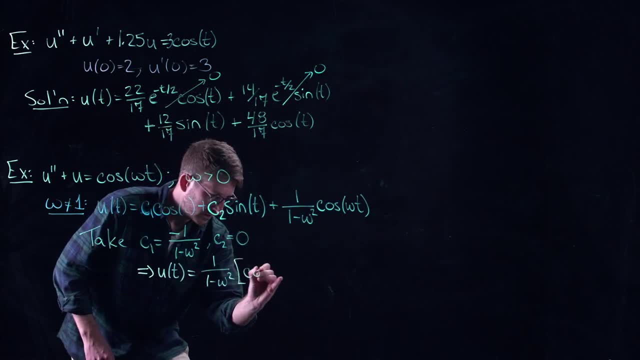 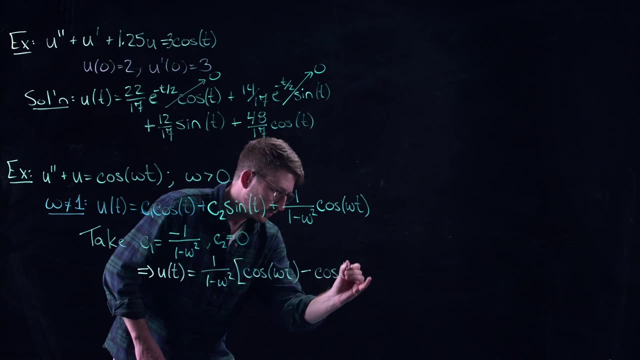 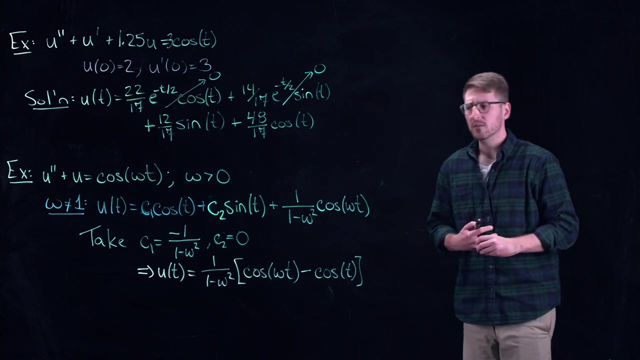 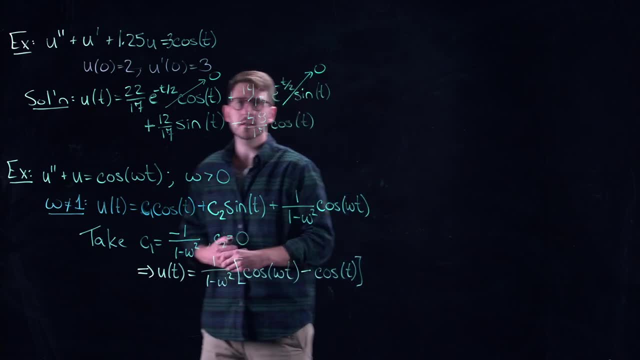 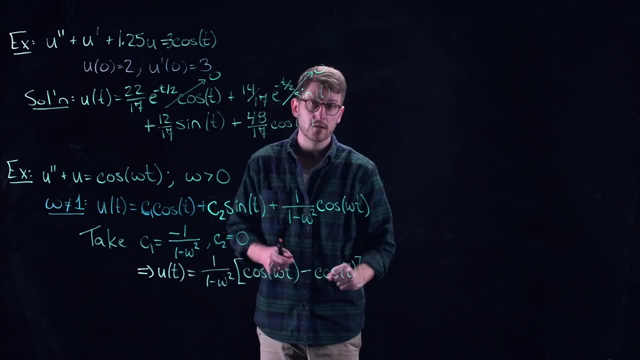 know, Maybe it looks a little better to you, but it's still not completely illuminating. Here's what I'm going to do: I'm going to use a trigonometric identity. right, There's a way, there's a trigonometric identity that tells you the difference of cosines. 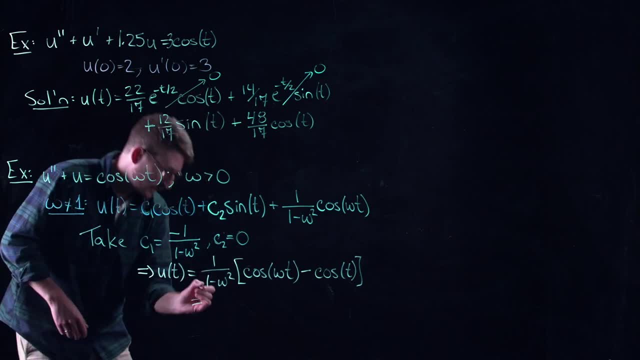 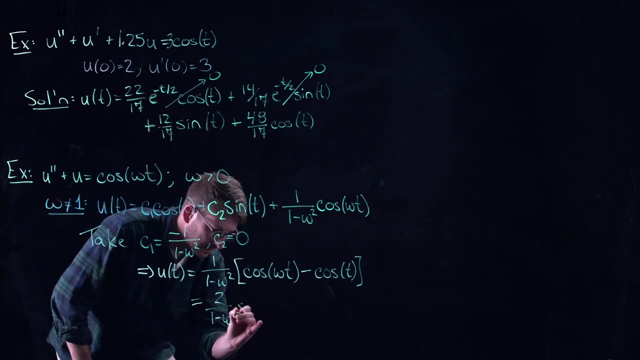 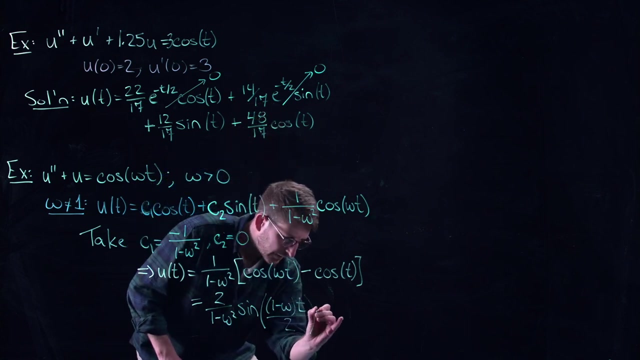 You can write this as the product of sine functions. So in fact this becomes two and then one minus omega squared and then sine. Now let's do this properly: One minus omega two and then one minus omega squared, Omega t divided by two, and then sine, one plus omega t over two right, So there's two frequencies. 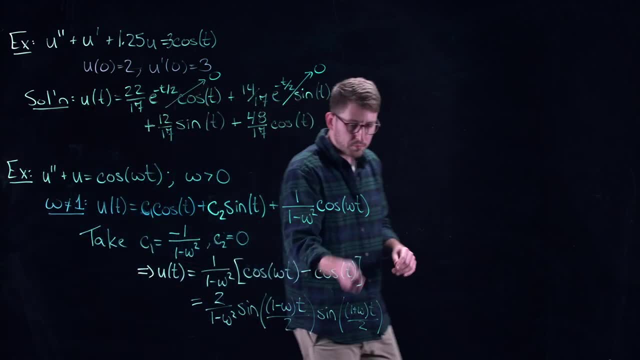 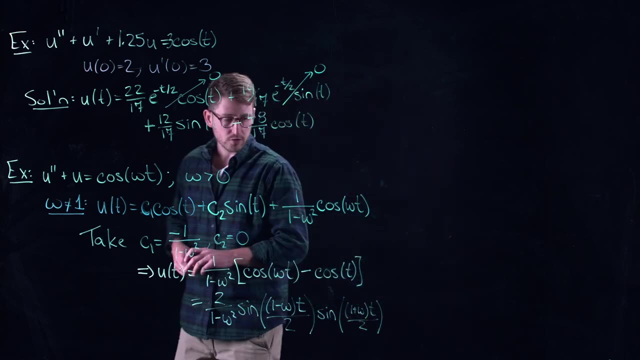 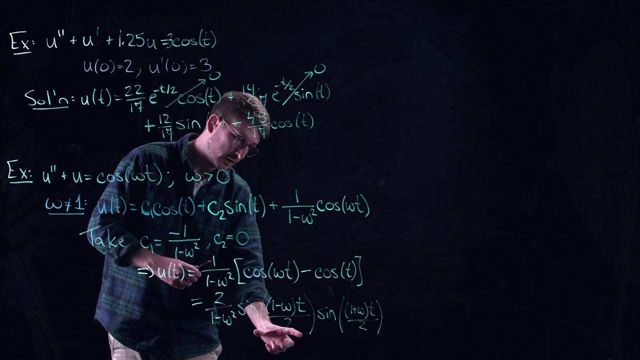 in these sine functions: one minus omega and one plus omega. Actually, technically, it's one minus omega over two and one plus omega over two. But what does that actually look like? Well, one way to interpret this thing is to think of this as the amplitude of oscillation and to think of this as the envelope of oscillation. 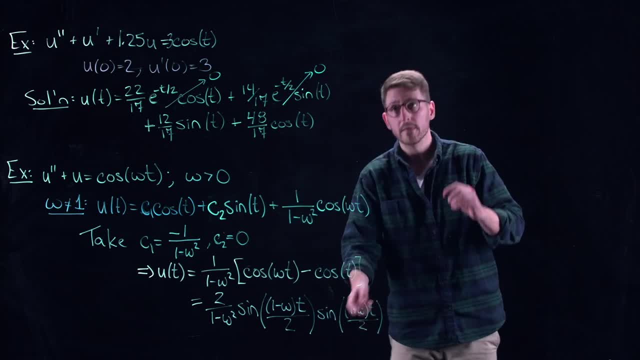 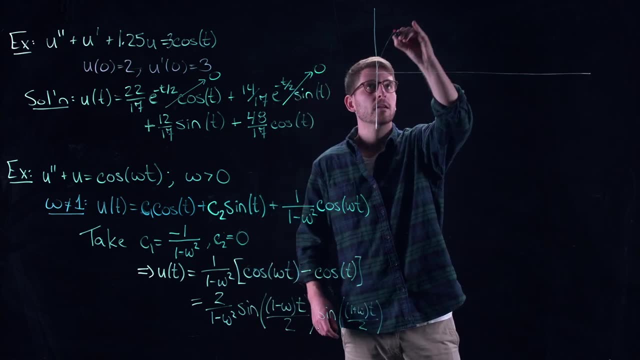 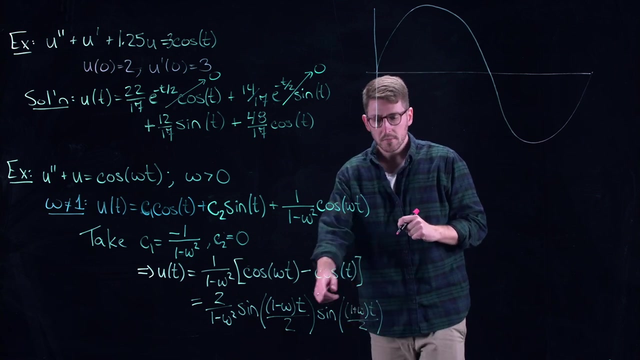 So what does this really look like? Well, if I just plot this thing, so let's do that first, That is going to look like just a nice sine curve, right? Similarly, if I plot the negative of that, so let's maybe put it like this: 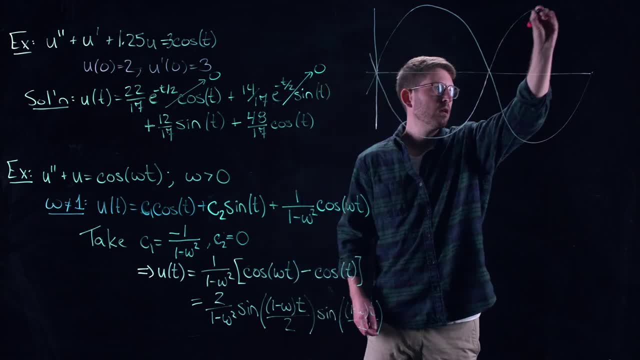 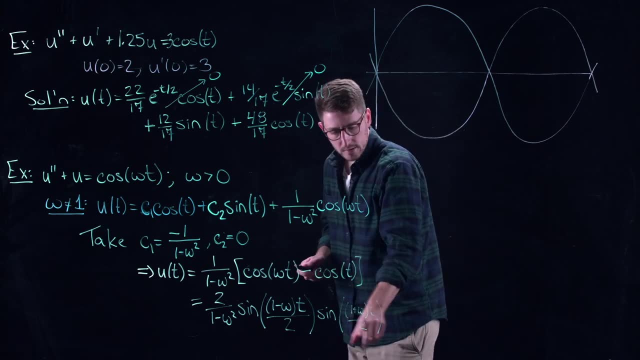 So if I plot the negative, I get this. Now, this is why I called it an envelope, because this thing tells me how big I can be in terms of oscillation. That's, assuming this piece is equal to one right Or negative one. 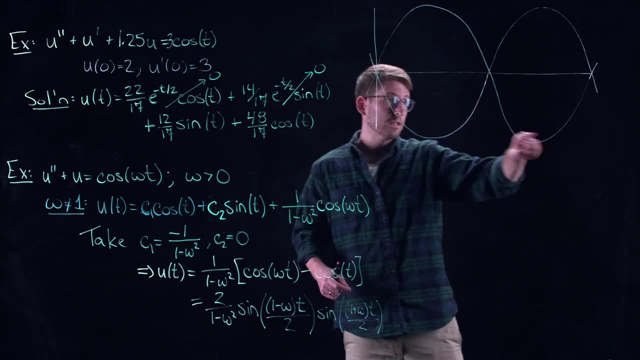 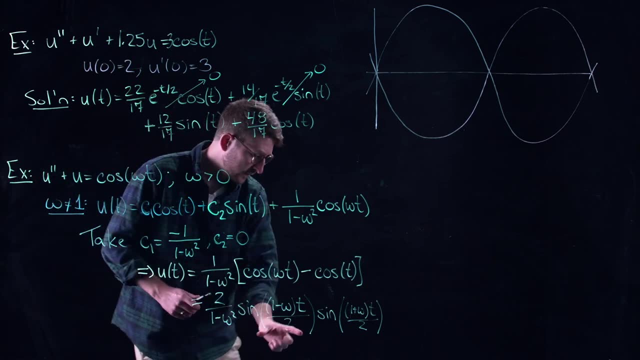 At the very worst right. I'm going to get this thing on the tops and bottoms. Now, what that piece right here is giving is it's giving an amplitude modulation right. The amplitude of this thing is not always one or minus one. 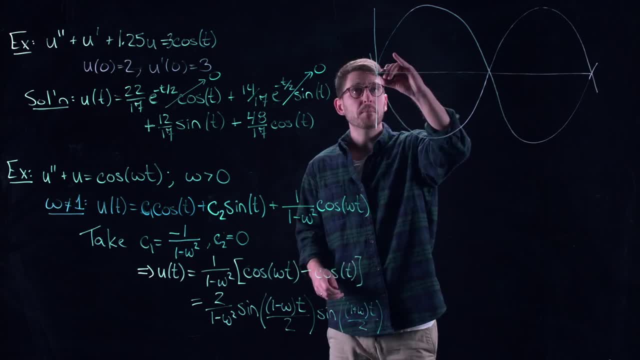 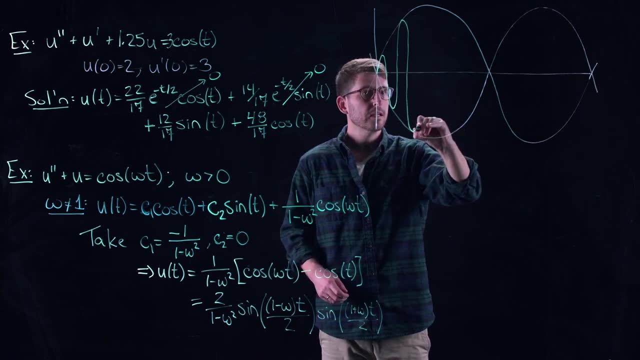 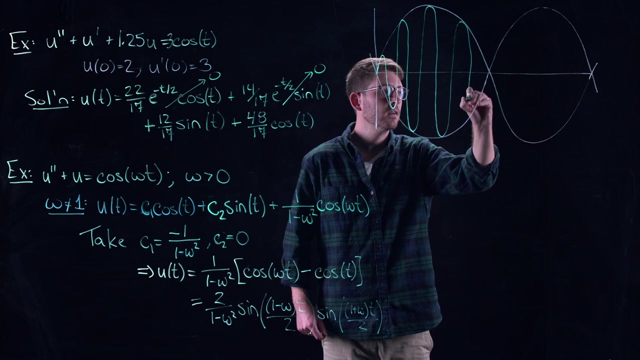 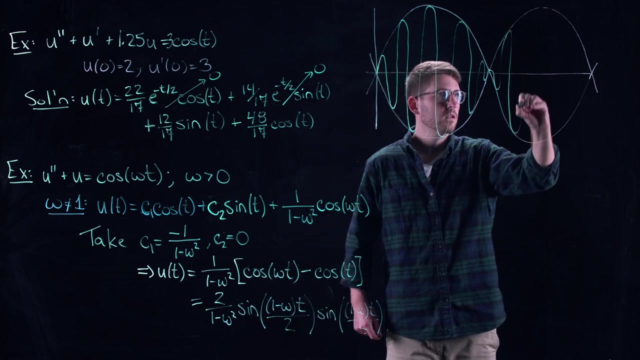 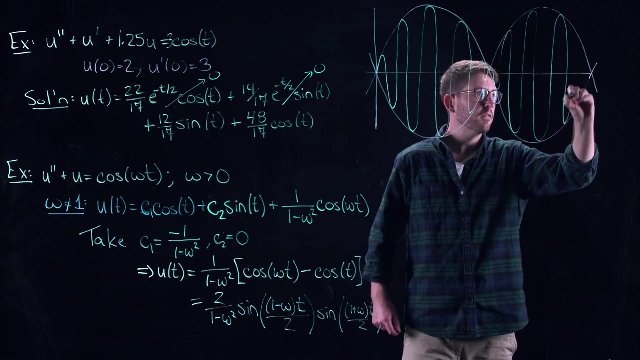 That's the biggest it could possibly be. So what happens is you see that you can only bounce around inside of this little envelope. So this in green here is actually the signal that I'm getting out of this thing. Okay, so it goes all the way up to the envelope edges. 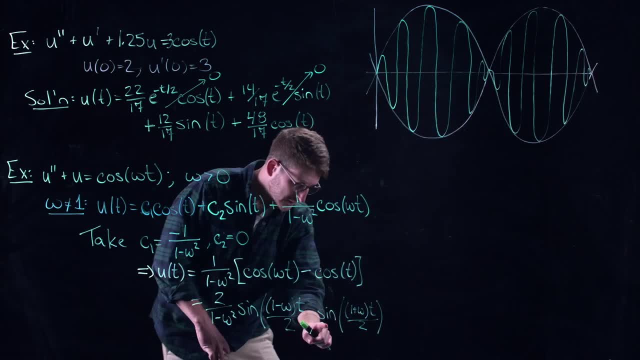 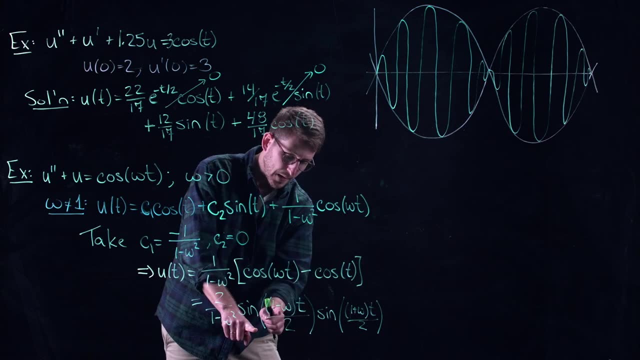 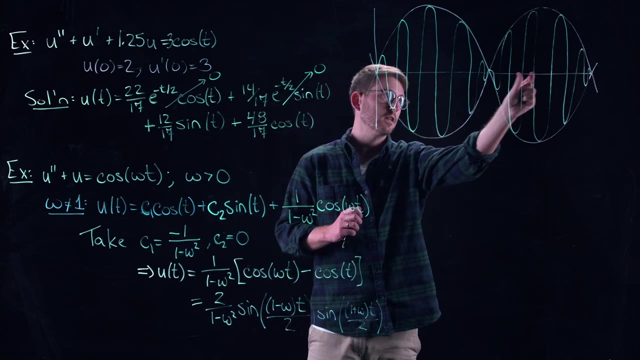 Okay. so what's happening is that when this thing is equal to plus or minus one, it's major in extremes right, Which is happening quite quickly because of the one minus omega being smaller than the one plus omega. That's why there's quick little tight oscillations inside of this. 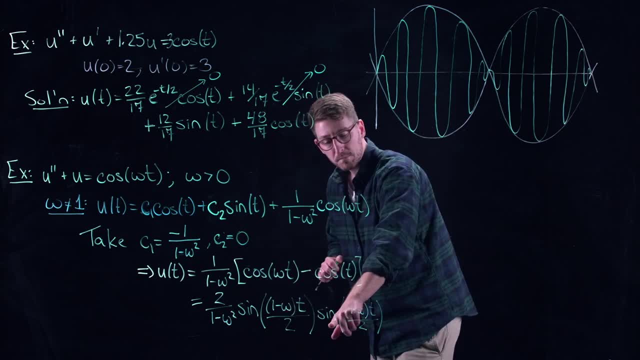 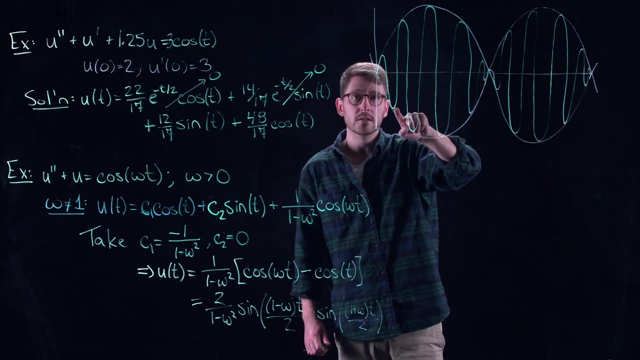 It's bouncing between the two. So if I plot this thing I'm going to get this thing on the tops and bottoms. It's bouncing between plus or minus one, which means it's bouncing between the values of this thing. That's why I go all the way up until I hit the envelope and then all the way down until I hit. 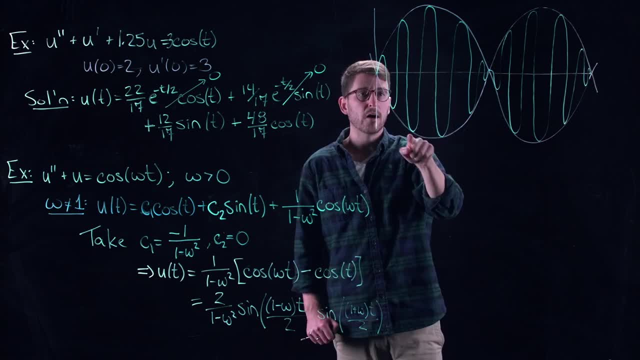 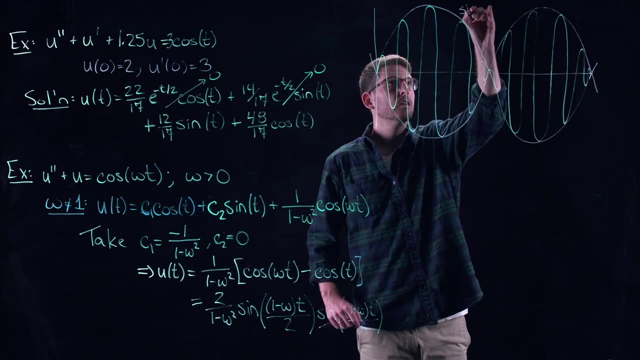 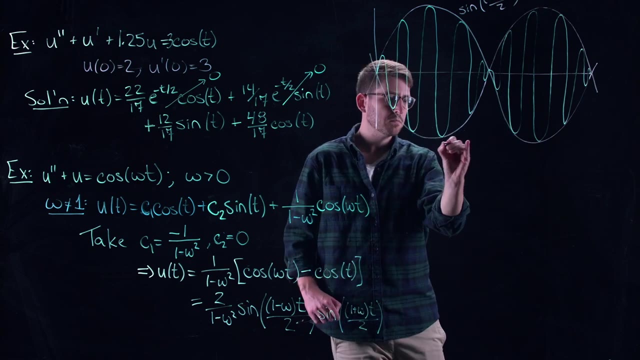 the envelope all the way up until I hit the envelope all the way down. The envelope, remember, is given by the outer function. So if we do sine of one plus omega t over two, right, And this is minus sine of one plus omega t over two. So if I plot this thing, I'm going to get this thing on the tops and bottoms. 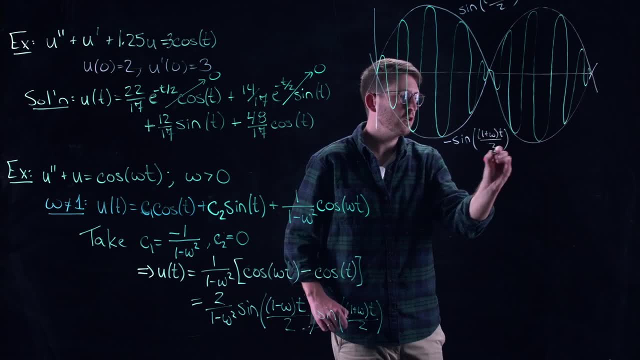 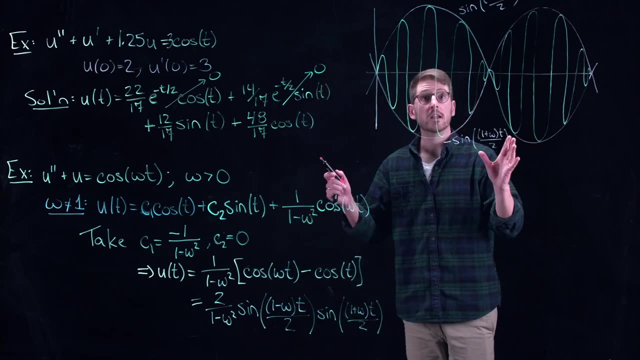 One plus omega t over two. Now I've completely disregarded the two over one minus omega squared, just because it's not helping us. It's just a number, right, It's just going to stretch or compress this thing. I want you to understand the oscillation that's happening here. 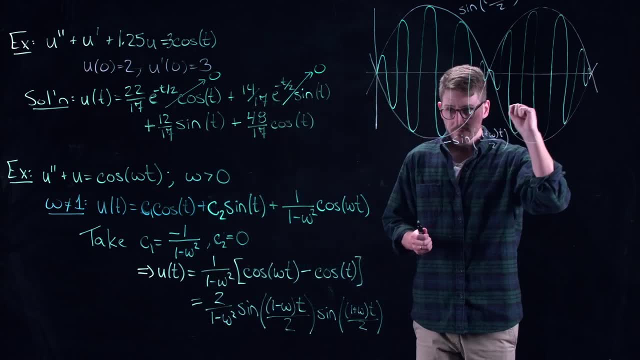 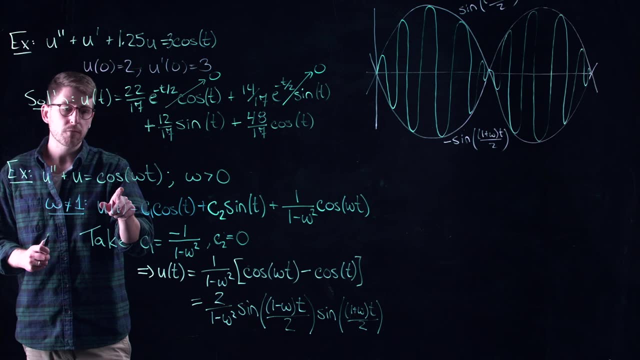 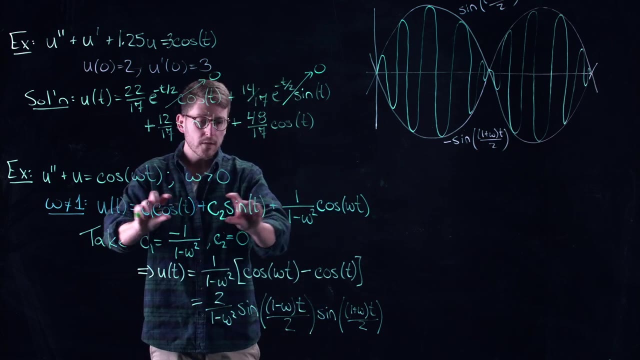 This is a modulated oscillation right. So essentially what's happening is it wants to fall into its own oscillations, but you are forcing it into oscillations that are sort of incommensurate with what it wants to be, And what I mean about that is that it wants to be. 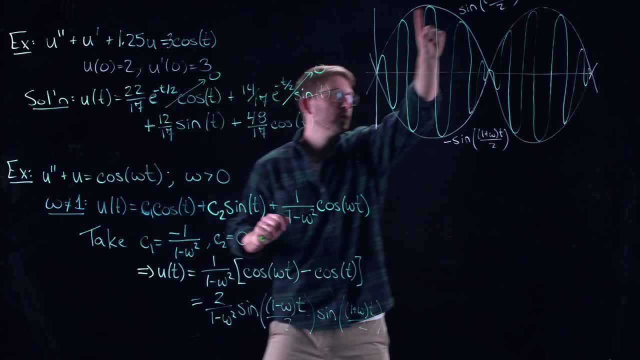 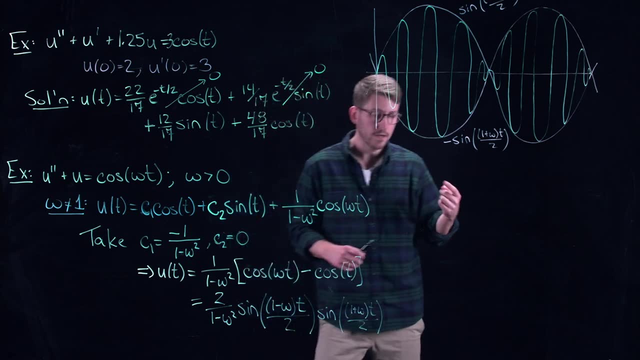 sine of t and cos of t, just the sort of outer oscillations here. But you're sort of pushing it at something that doesn't sync up with it right. So you can imagine, you know you and I are. 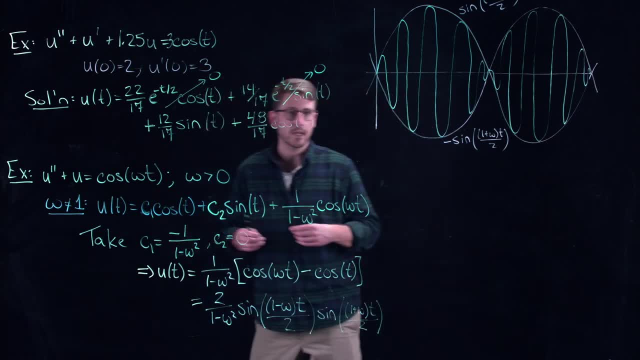 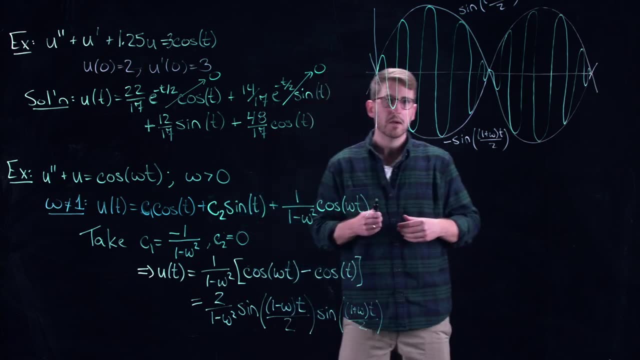 walking side by side. Every time I take two steps, you take 2.3 steps or something like that right. So we're sort of have this weird incommensurate period to our stepping right After I take one step and two steps. 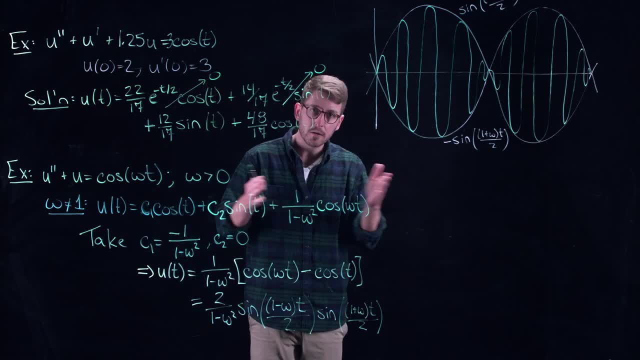 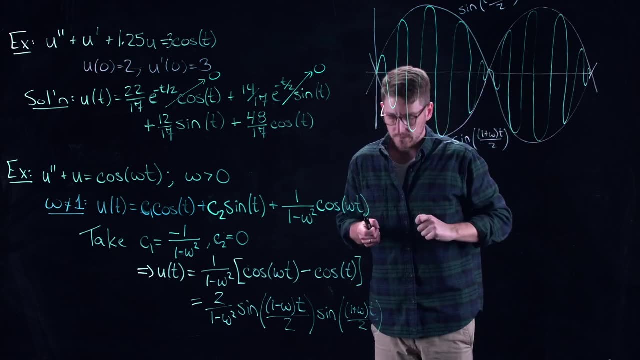 you've taken maybe 2.3 steps, right, So we're going to be off, We're not going to be synchronized. That's what we're seeing here, And this is where you're getting this modulation that's coming in right here Now. the last case here, of course, is what happens when 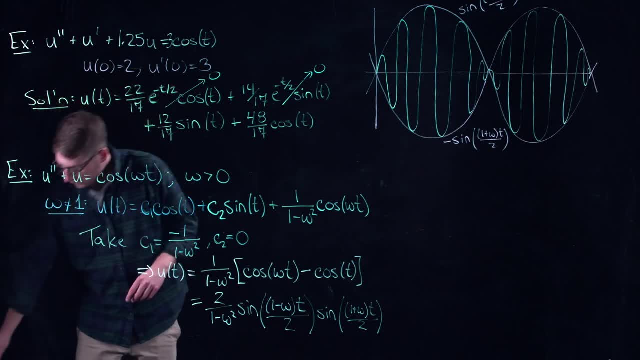 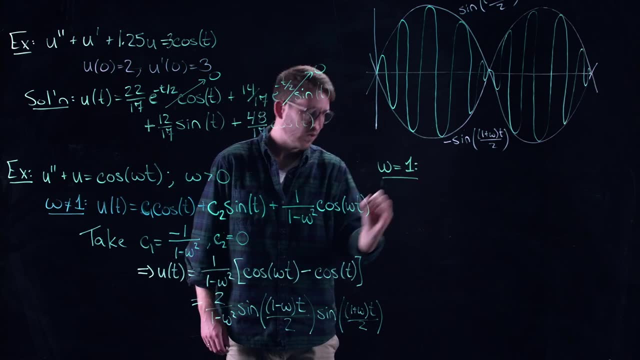 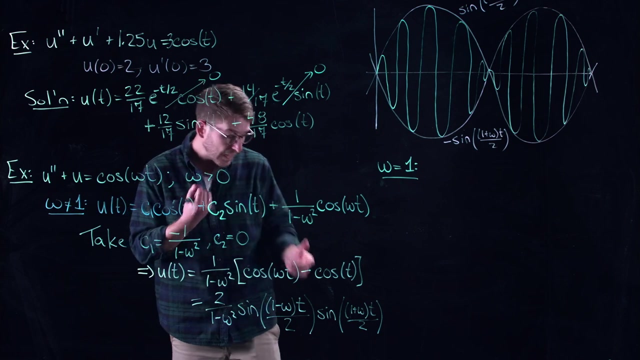 omega is not equal to one, So let's take a look at that before we wrap up. Sorry, Omega equal to one now. Well, that means that I'm forcing it at the same frequency that it wants to be at right, And so now I can get the exact solution out of this thing. 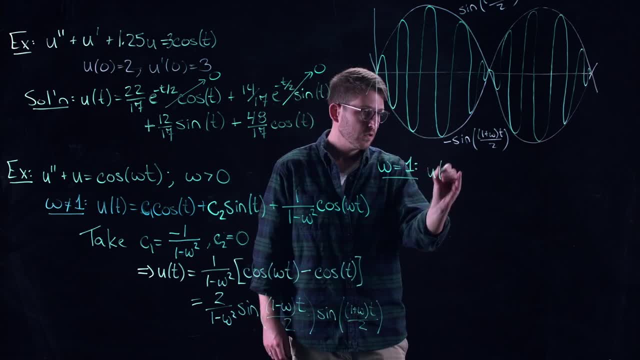 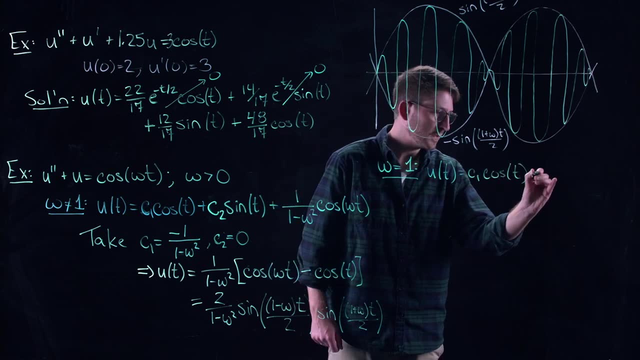 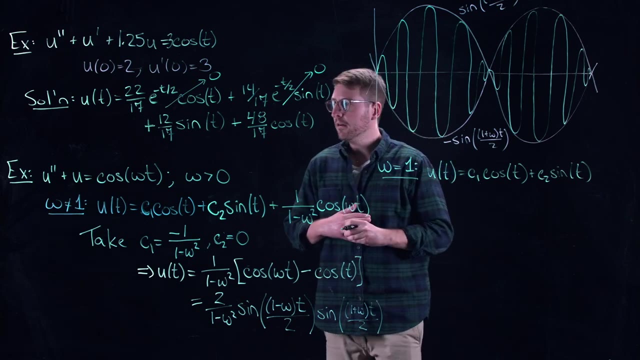 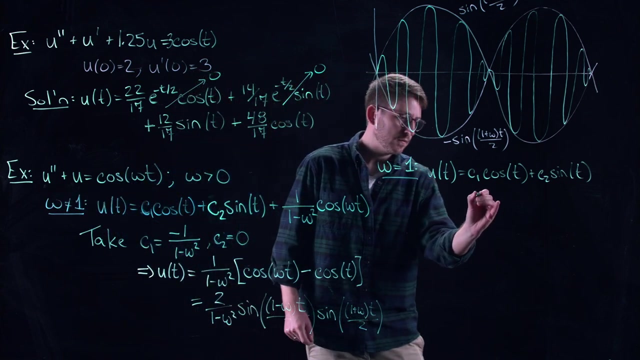 And this is going to be: u of t is equal to: so c1 cos of t plus c2 sine of t. The homogeneous part never went away. And then I have: well, I'm going to get an a here, I'm going to get an a here, So I get. maybe I'll just call it. 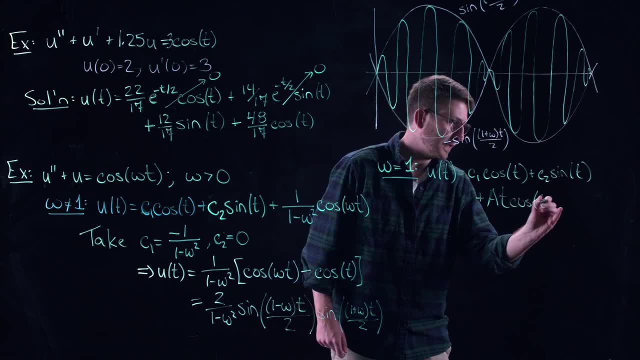 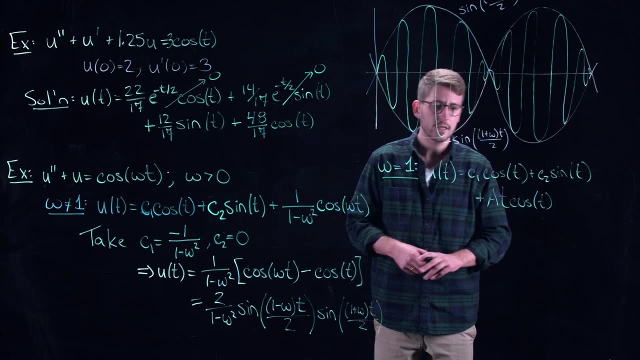 At cos of t right. So again, you can. you can compute out the a Again. it's only going to be a cosine that comes through. It's the sort of same thing that we saw right here. But here's the point. I get a t now. All right, I get a t. 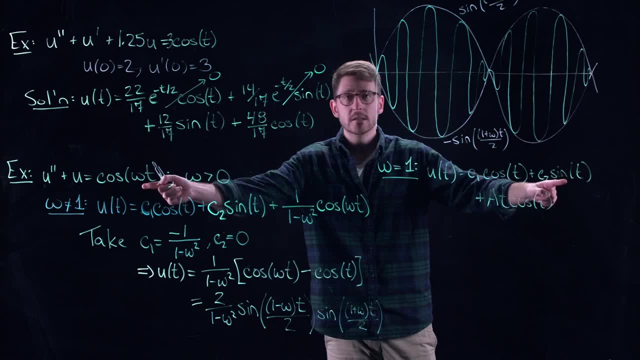 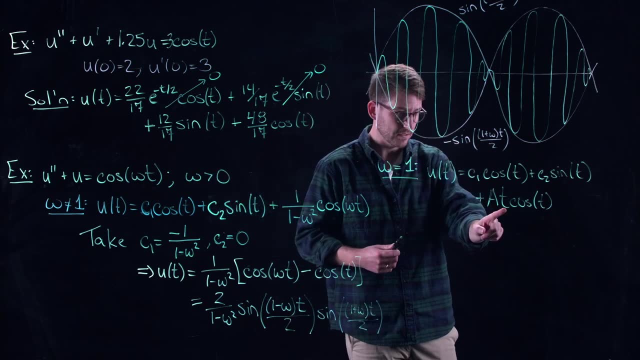 because the homogeneous part is already covered And the forcing is the same as the homogeneous homogeneous part. So we've seen this before, right. This acts like a repeated root. It means I get a t in here. Now this is interesting, right, Because in this case I never grew. I was always sort of 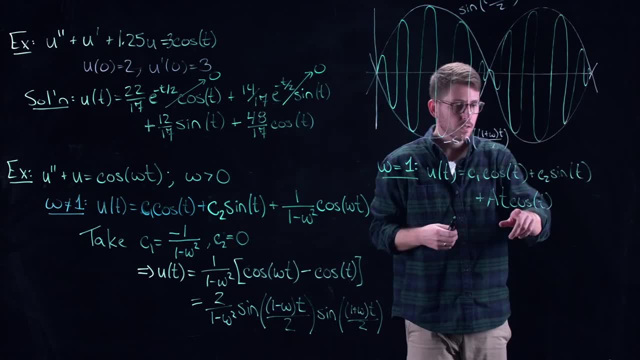 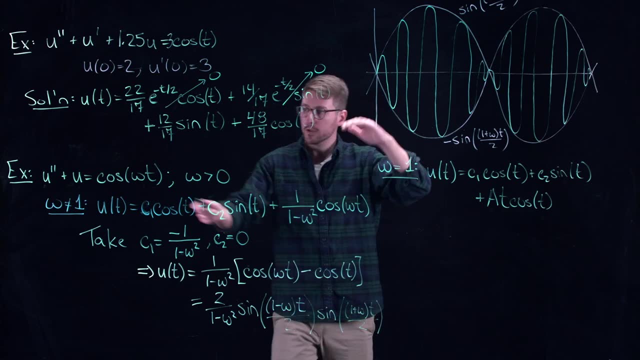 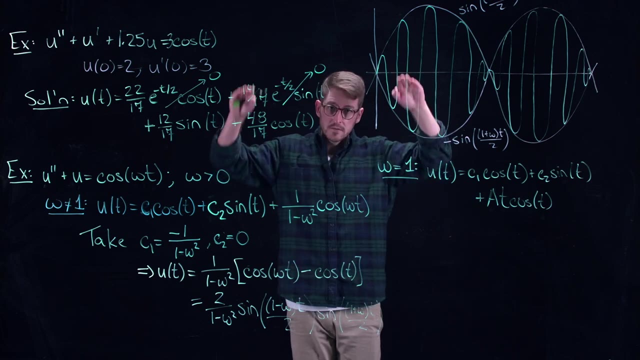 stuck between, say, minus one and one. What's happening here? Well, whatever the natural period that this undamped, free vibration, so this u double prime plus u falls into, I am forcing it at exactly the same period, right? So every time it goes to its lowest extreme, I am also going to. 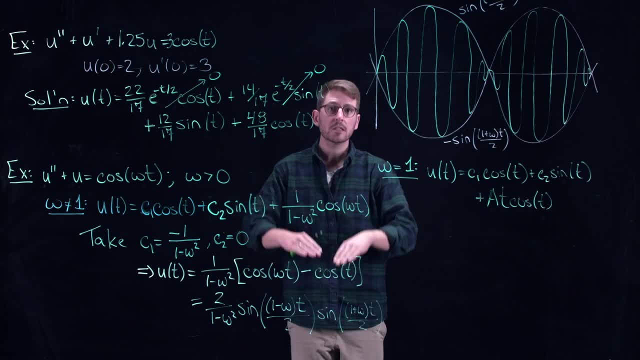 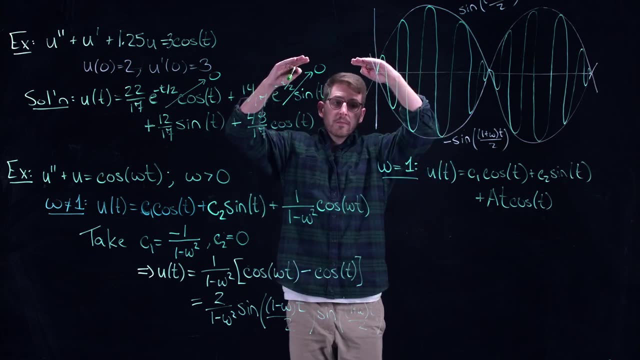 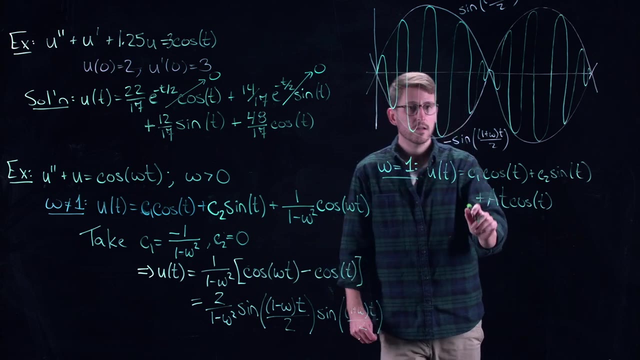 my lowest extreme and I'm pushing it down further, And then every time it comes up to its highest extreme, I am also going to my highest extreme with the forcing and pulling it up even further. So what you're getting is: you're getting growth here, right. You're sort of skyrocketing Now you. 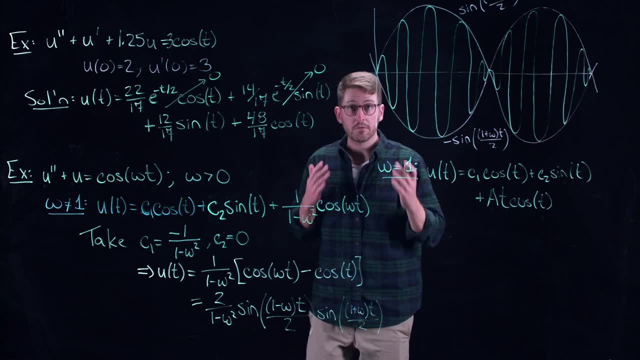 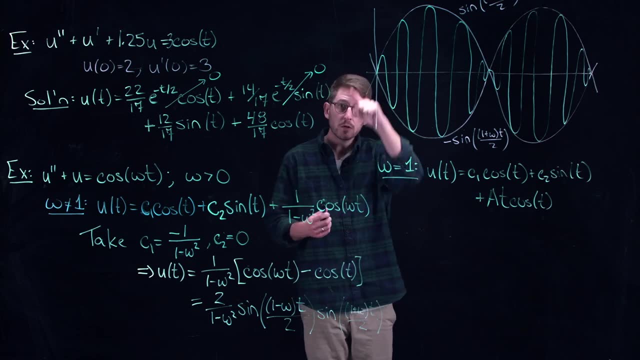 may have seen this before, If you've ever been on a trampoline with your friend. you get your friend bouncing and they fall into a nice periodic bouncing. Then what you do is you start bouncing beside them And what you do is you try and synchronize yourselves so that when you come down, 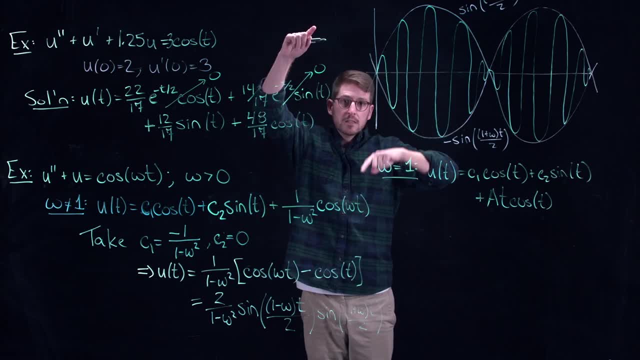 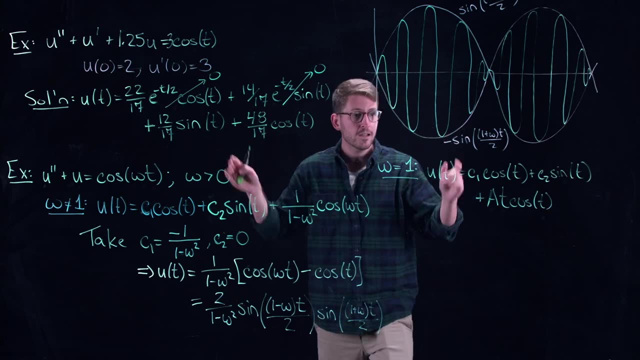 your friend comes down and you skyrocket them, right, It's almost like a double jump. Now, if you were able to sort of maintain this and if you know, physical restrictions aside, you would be able to bounce them as high as you wanted, right? You could bounce them to the moon just using that.